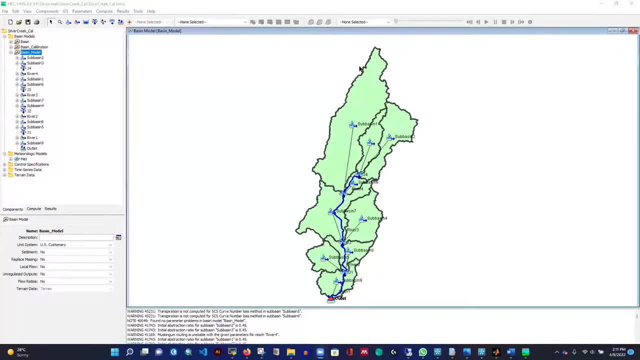 hi everyone, today I'm going to show you how to calibrate a model. basically, this is a HEC-SMS model. if you want to calibrate your model, then you can follow all these steps, and in my previous videos I have already demonstrated how to set up the model. so this model is pretty small, not that big, but if you can, 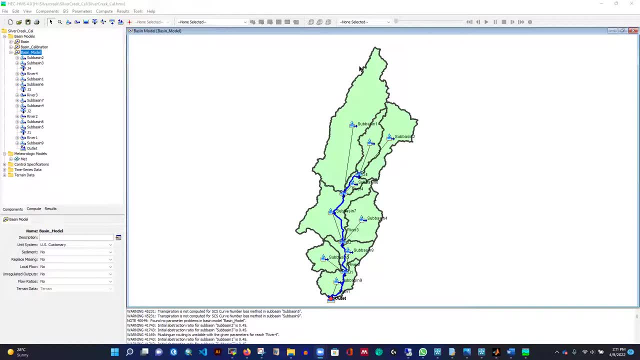 develop a model that is big, it doesn't matter. but here you can see, I have only nine sub watershed here, sub basin 1 to sub basin 9, and I have only one outlet for this entire model. I didn't even add more, because I have only observation. 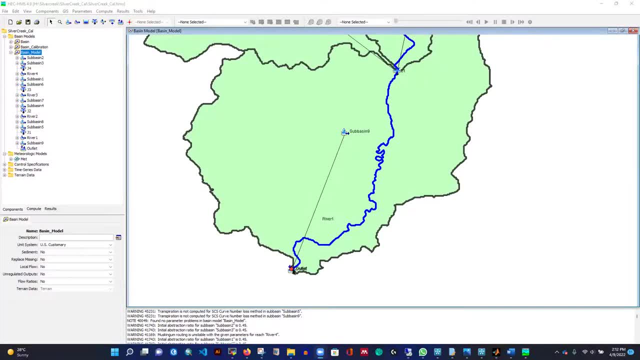 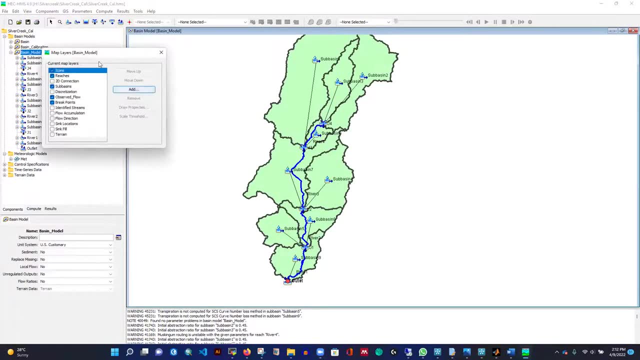 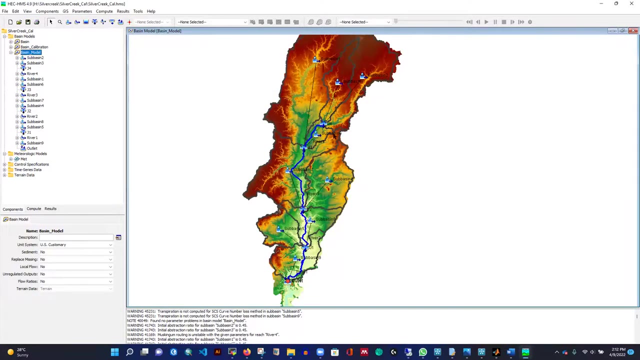 that I have the outlet of this watershed here. so if I want to turn on the DEM, you can see from view map layer and I can turn on the train and you can see it's there. so that is the DEM. that is my model. the area is not that even steep, it is kind of flat area now. 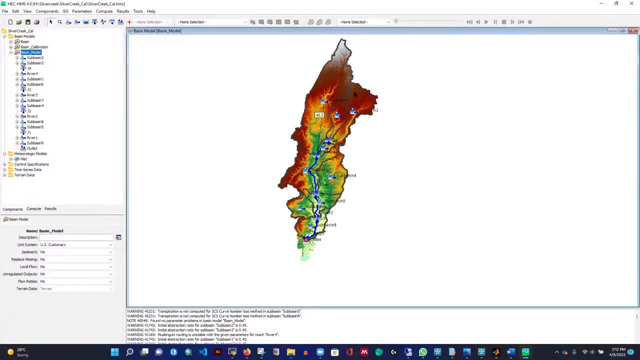 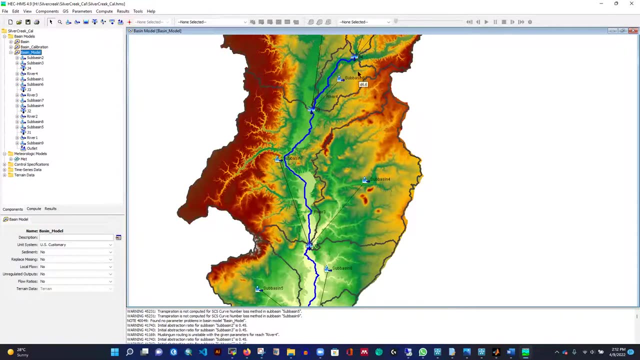 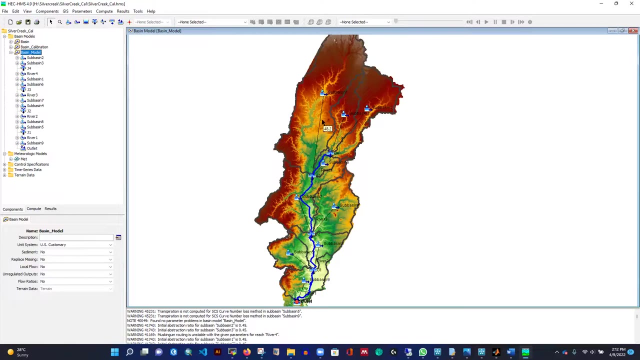 look at it somewhere in Illinois, okay. so here I'll even calibrate the model for all these sub basins and the reaches I have. I have only four reaches: the rivers that are connecting these three sub basins locating upstream of this watershed. so let me explore what I have here means in my sub basin, if I want to show. 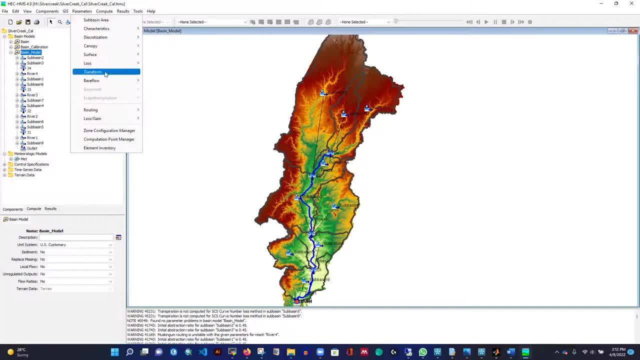 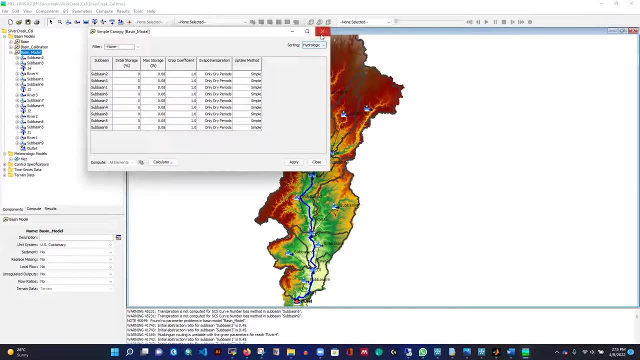 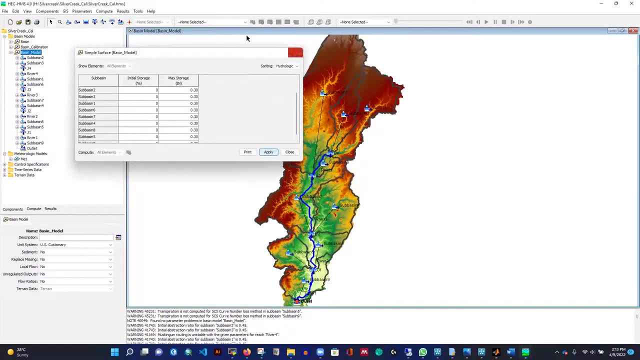 you what method I used, so I'm going to show you from parameter I use this canopy method, a simple canopy right. I have used this once and then. for surface method I've used simple surface and for loss method I use SCS curve number. you can see that this is the surface method and this is the surface method and this is the. 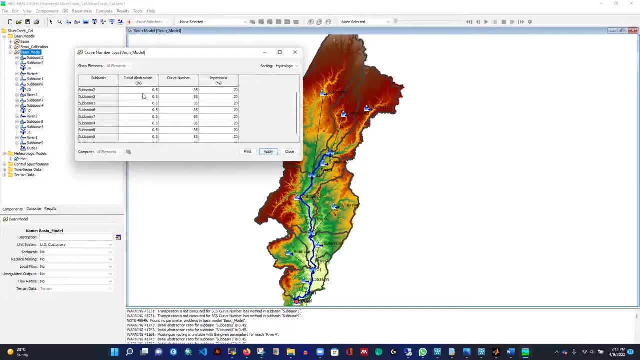 surface method and that is the curve number and for initial abstraction I estimated these values as 0.5 and the curve number I have which go on any, and it's 85 and impervious percentage of imperviousness is 20% for transform. 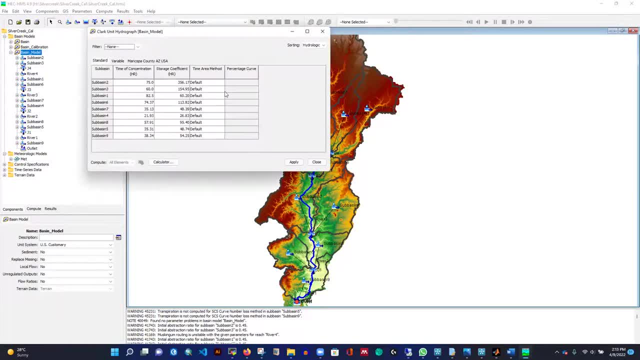 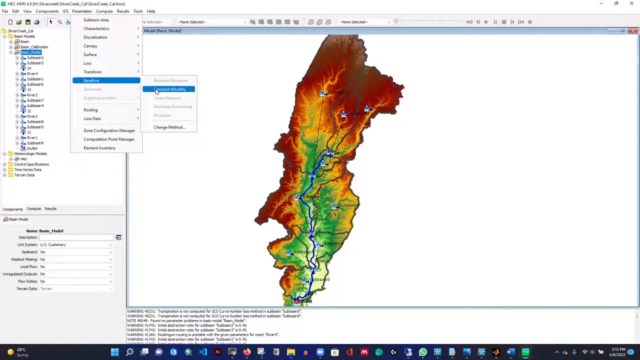 method. I used Clark unit hydrograph and you can see, we need to estimate all these parameters- time of concentration and a storage coefficient- and we will show you how it works. so let's go ahead and start the process. so I have this initial values and then I have the base plus. for this case I use like constant. 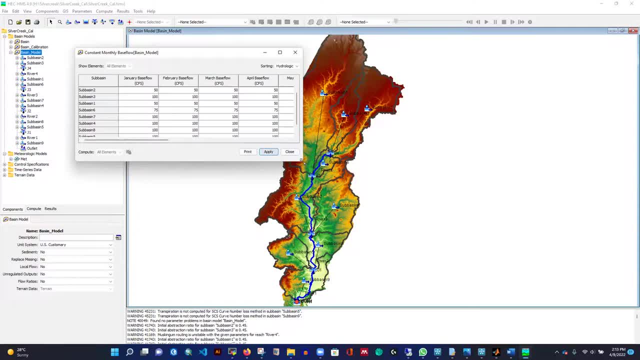 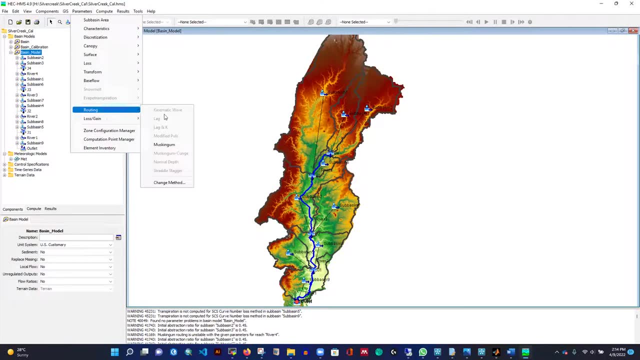 monthly, for each of this month, I have these values, or each of these sub basins, and then for routing method, I use masking gum and for masking game. you know that. okay, we have two parameters, like a screen them K, that is the travel time we need, and we have another X value. 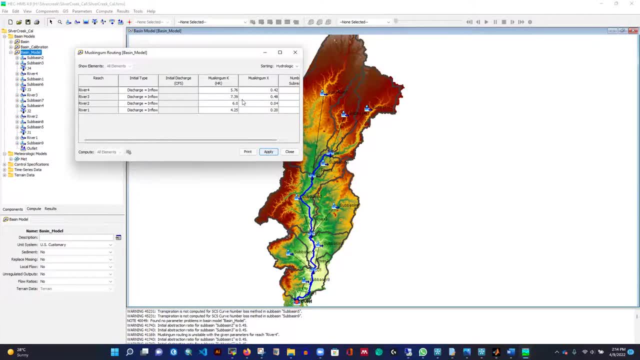 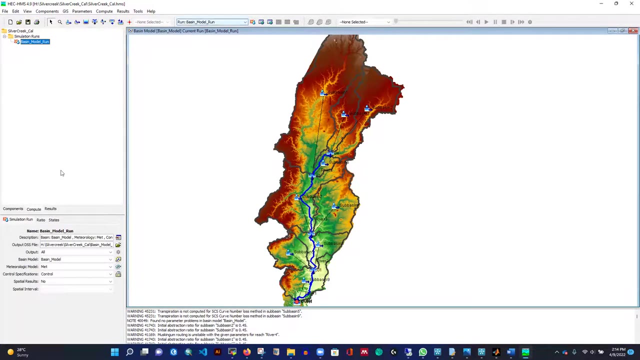 that varies from 0 to 0.5. so this is my first estimation of the model parameter and if I run the model, you can see I have already generated the run and here we can see the run. okay, before going to run the model, I can even show you other parameter I have for Mac model. 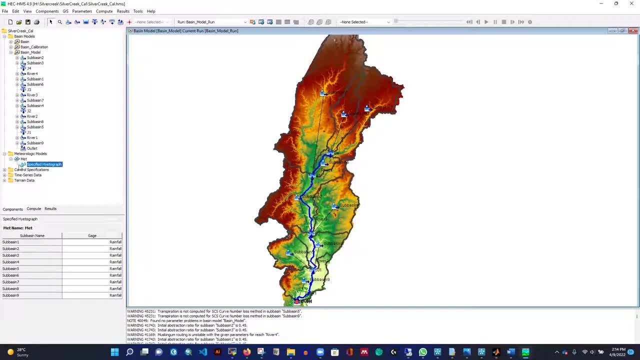 I use like specified hiatograph and for time series- I have precipitation time series- I used only one single gazes, one single gaze for the entire watershed and the study area. so that is another challenging task to calibrate the model and you can see that this is my graph: the rainfall. 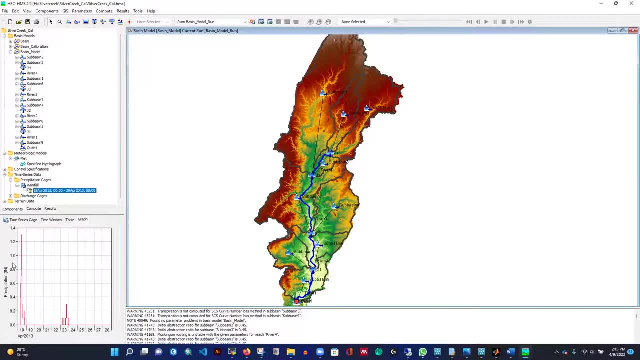 data. I have here the hiatograph, I have rainfall depth in inch and I have this kind of shape. basically this is an event based model and for observation I have the discharge and you can see the plot is like that. so we have pretty flat top of the. 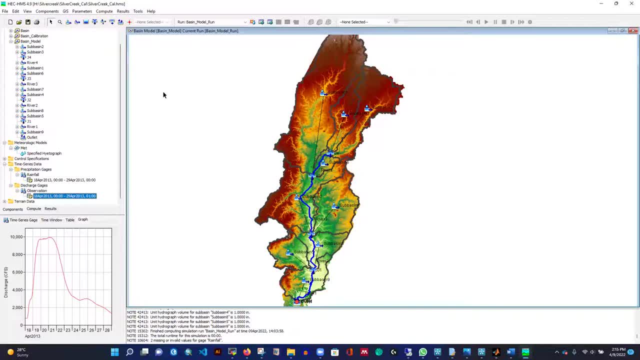 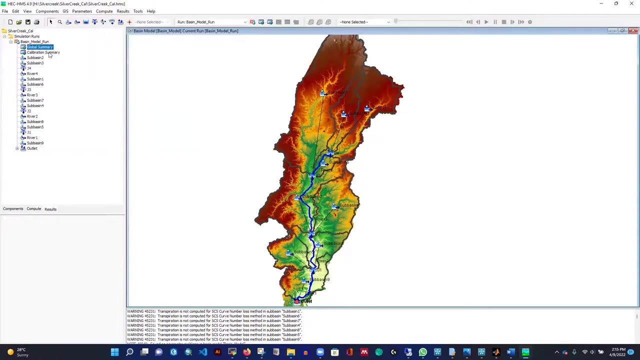 hydrograph and if we run the model, you'll see here, because the model is running for a few days, it's even slow and I can see the results here. so we have the global summary here, we have the summary, okay, and then we can see that the outlet, because we don't have anything for other sub basins. so 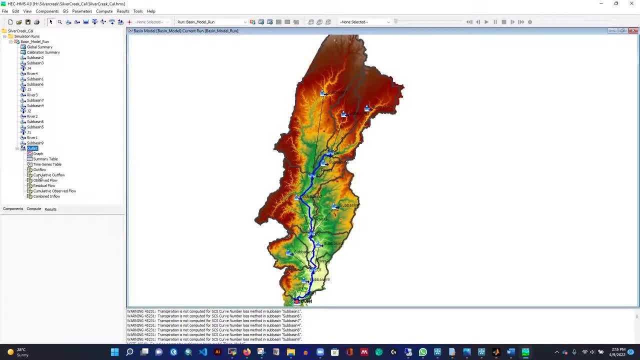 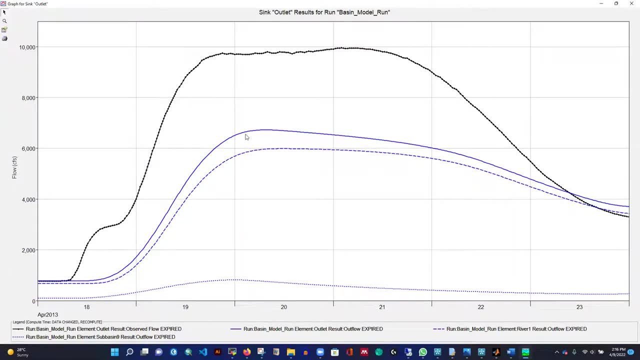 we can see the plot, so you can see this farm line. this line is basically the accumulation of all of this watershed. right, all the flows coming in, so you can see here the sounds like this is mother shot- right, all the flows from the opposite water state and sub basins, and then that is the black line. this is the. 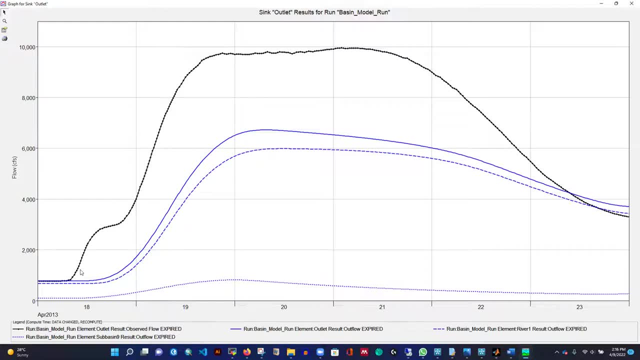 observation. so our goal for today is to match this line, this blue line, to that black line right. so that is pretty challenging because the observation we have, it has a flat, flat top it. it should be like that, but because of some storage of water or some intervention with a dam right within the 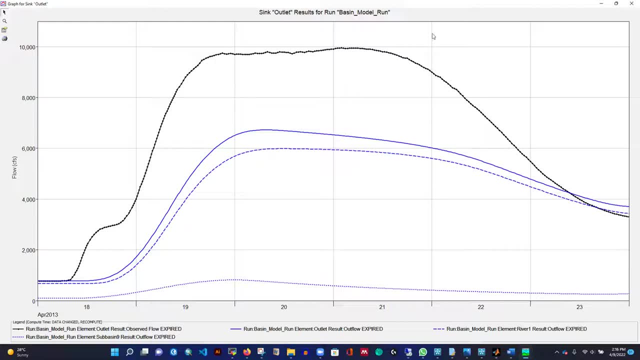 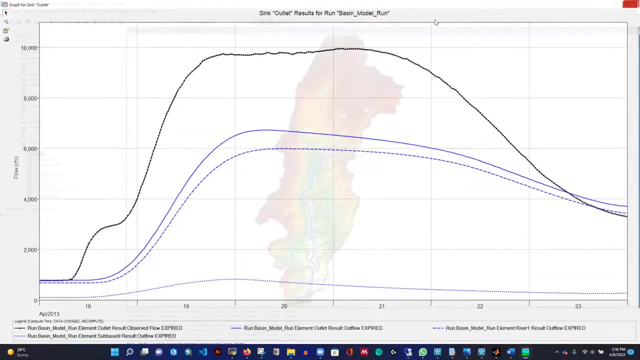 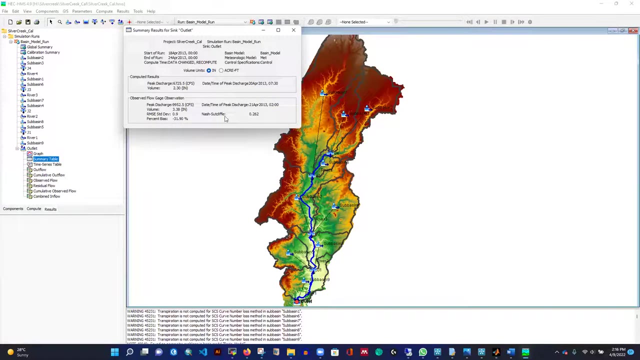 study area. i already checked it, so the curve is like this. so, okay, we'll try our best to capture that observation using our model, whatever parameter we have. so let's see the summary table. the present condition we have, like the nsc value is 0.26. 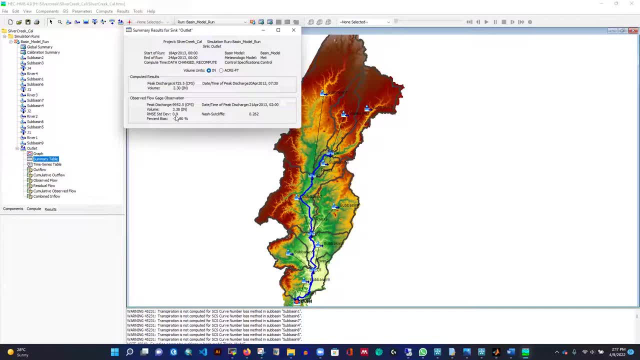 and the percentage bias is more than 30 percent right and the rmsc we have 0.9 standard deviation and the peak discharge is like this. but from observation we have computed is this and this is the observation. so our model is basically underestimating whatever. 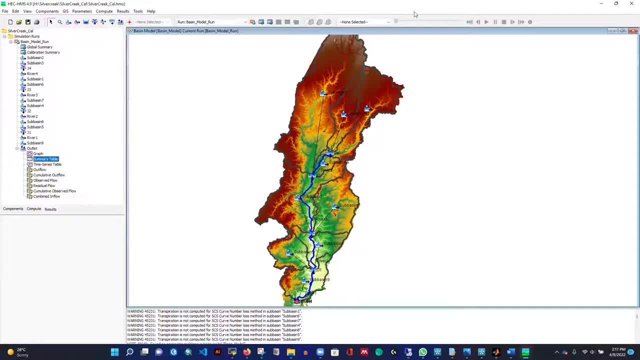 observation we have. so let's see if we can even capture the shape of the hydrograph using our model. so for capturing that one, okay, i can try, because i don't know how to even approach the process. but from my experience, what i do, i start with the loss, because this loss factor is very important, because our model is generating. 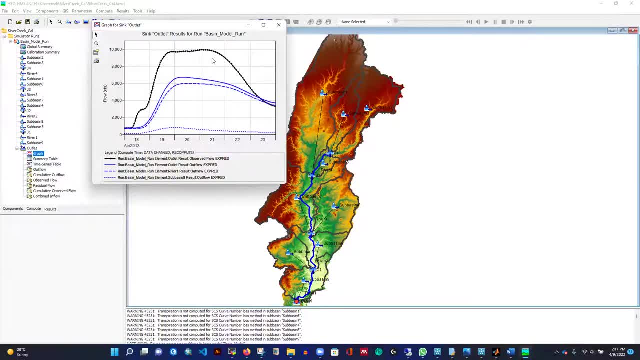 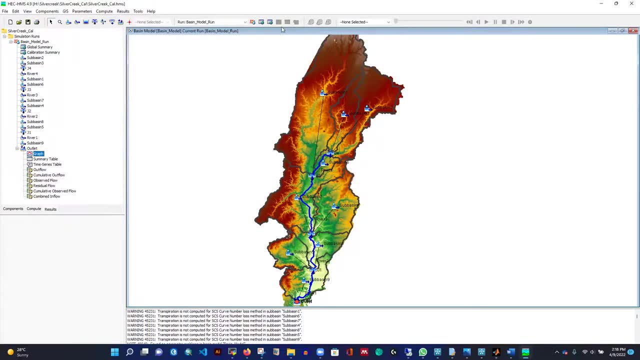 a hydrograph that is even lower than the observation. that means our loss is higher than the actual loss. so we have to reduce the losses right. so we can do it, because, if we don't know, because we have nine servarustshed, we have even four rivers or reaches, so how can i even approach the? 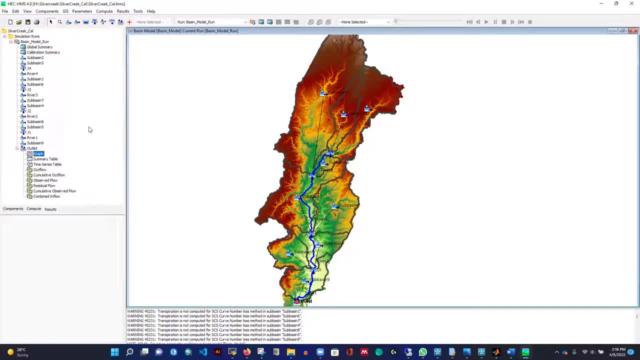 calibration. it will take a lot of time. so at first we'll try with automatic calibration and then we'll try to fix it using a manual calibration process as well. so for automatic calibration process, what i can do, i can even add that compute or from compute you can go to optimization trial manager. 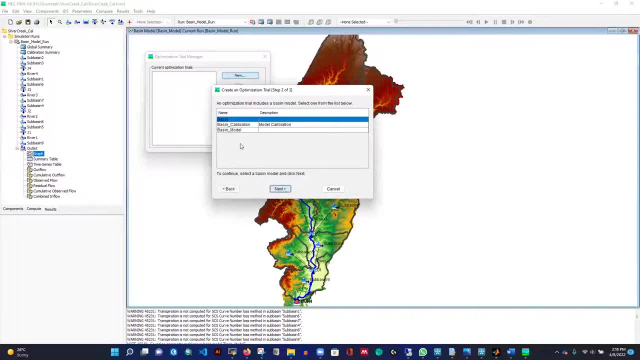 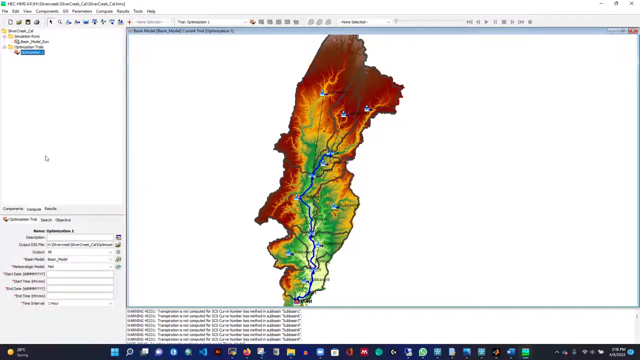 and you can go to new and optimization one. i'm using my basin model. i have three basin models, so basin model is there clicking. next i have one met model and everything is same. so i think it's there. it's there, so it doesn't have any parameter now. so what we have to do, we have to even. 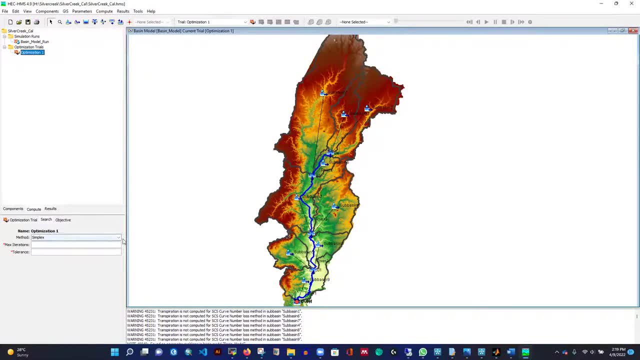 go to search and use the method right, simplex method. we can use the simplex method and then for maximum iteration, i can even select 100, and the tolerance, i can select 0.01, and for objective function- you can see, we have these options- root, minuscule error and in order to 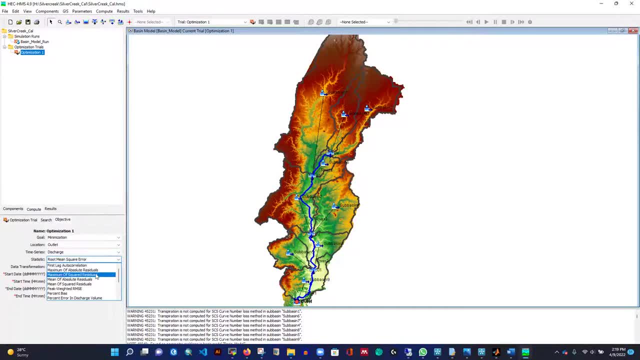 capture. you can even use first lag autocorrelation. you can use of peak weighted rms if you want to capture the peak only, if you are not even bothered about other base flow and everything. even if you want to capture the volume, you can use this one, but for my case i'm using this root mean square error, my objective. 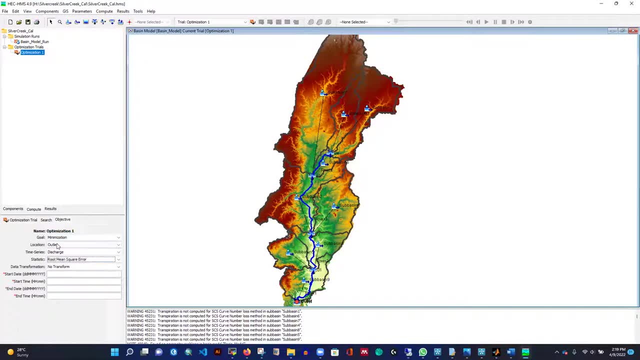 function will minimize this rmsv value, and the location i have is the outlet at the downstream of the entire study area. and for start time, end time: right, we know the like time is zero, zero, zero. we know this and i'll show you the data as well. so here, what is the date? we can even get it. 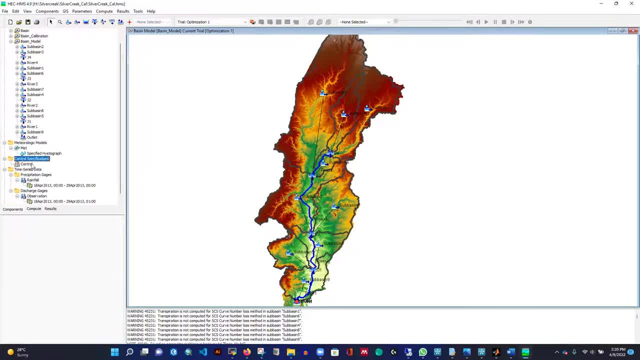 from our control specification. right, it is from 18 to 24. okay, 18, 26, 24. I'm just pasting it there. pasting it there, it should be 24: 8 into 24: 0, 0 and then it has to be like 0: 0. okay, we have this. so the time interval is 1 hour, okay. 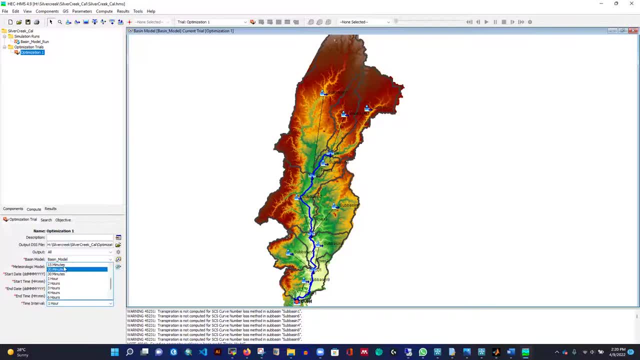 we can keep it 1 hour or we can give it 15 minute. usually I do it for 15 minutes, right? so we have this, this and everything is there. so for this one we can even use the same thing again. it should be 0: 0 and then 0: 0. hour ending. 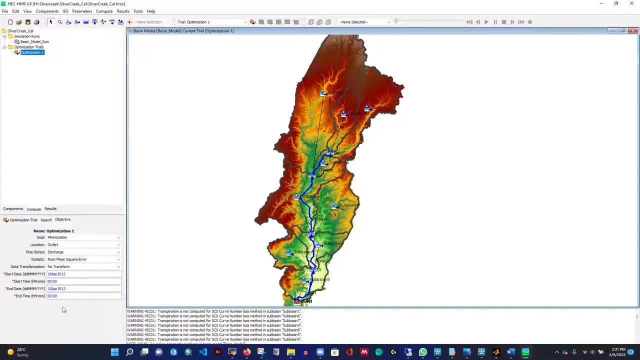 time should be the same, but this should be 24. okay, ending time. so that's it. even now, we need to add our model parameter. so add the parameter. whatever parameter you want to add, so add the parameter. whatever parameter you want to add, so add the parameter. whatever parameter you want you can add, because we have sub. 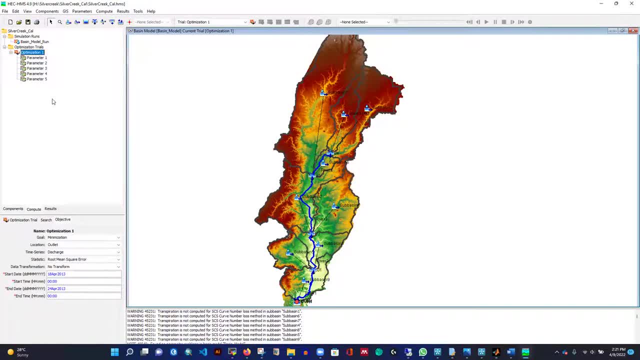 you can add because we have sub, you can add because we have sub basins and we have four rich. so for basins and we have four rich, so for basins and we have four rich. so for each of these reaches, we have like two. each of these reaches, we have like two. 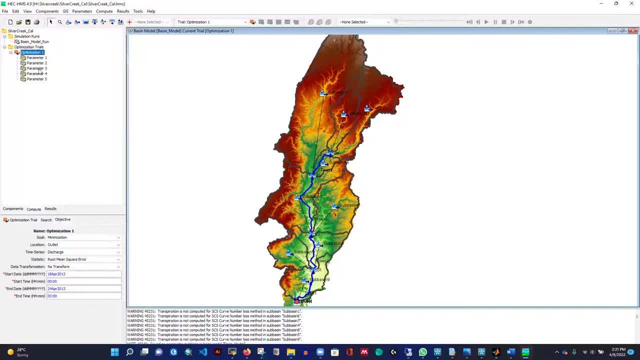 each of these reaches. we have like two different mushroom parameter- X and K, so different mushroom parameter X and K, so different mushroom parameter X and K. so we need to add like eight parameter, for we need to add like eight parameter. for we need to add like eight parameter for those four and then for sub basins we 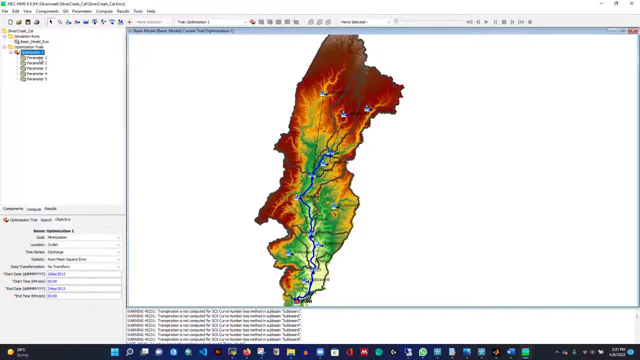 those four and then for sub basins, we those four and then for sub basins, we can use all sub basins and we can even can use all sub basins and we can even can use all sub basins and we can even check it. okay, for our first parameter, we 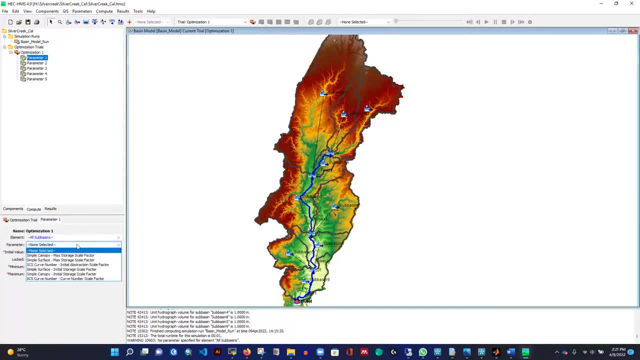 check it okay for our first parameter. we check it okay for our first parameter: we can use all sub basins and let's see: can use all sub basins and let's see can use all sub basins and let's see what parameter we have. so we're not gonna. 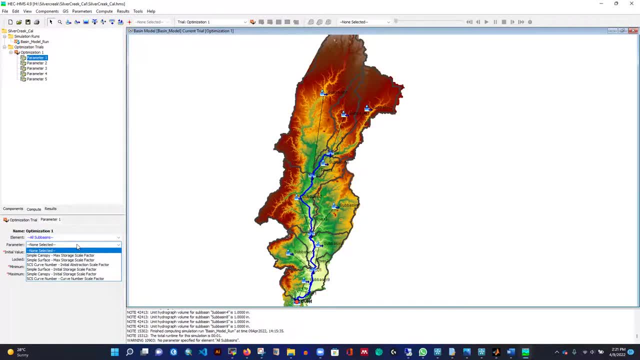 what parameter we have. so we're not gonna what parameter we have, so we're not gonna calibrate simple, canopy, simple surface. calibrate simple, canopy, simple surface. calibrate simple, canopy, simple surface. because these are the parameter value we, because these are the parameter value we, because these are the parameter value we already estimated from literature. we. 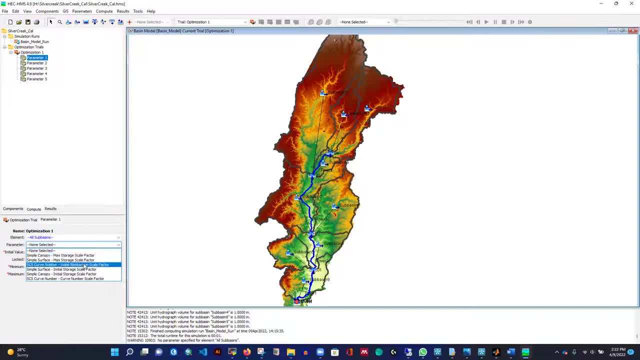 already estimated from literature. we already estimated from literature: we don't need to calibrate those because it don't need to calibrate those, because it don't need to calibrate those, because it has certain limit, so we can't exit that. has certain limit, so we can't exit that. 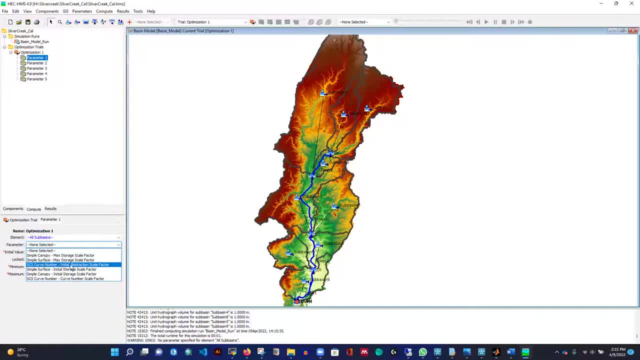 has certain limit. so we can't exit that one. so we can even calculate curve one. so we can even calculate curve number. but this is calibration number, but this is calibration number, but this is calibration parameter. initial obstruction scale parameter. initial obstruction scale parameter. initial obstruction scale factor. I can select that and for 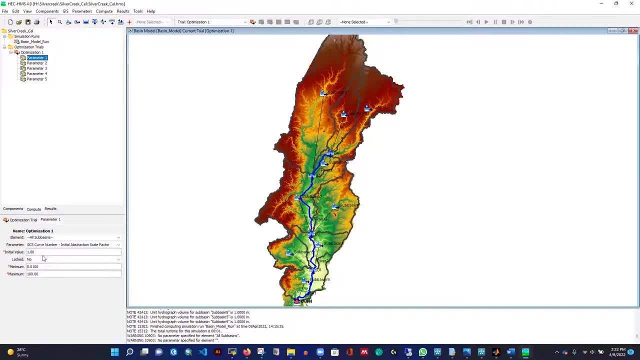 factor: I can select that. and for factor: I can select that. and for parameter 2: when you can check the parameter 2, when you can check the parameter 2, when you can check the initial value, they are giving like 1 and initial value: they are giving like 1 and. 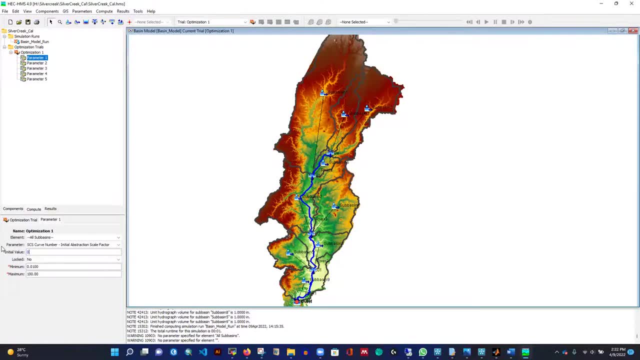 initial value they are giving like 1, and the minimum value is this. but for our the minimum value is this. but for our the minimum value is this. but for our case the initial value is 0.5, right, we case the initial value is 0.5, right we? 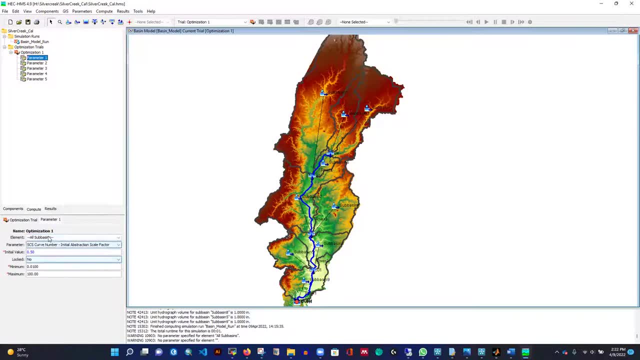 case, the initial value is 0.5. right, we already check that. and the maximum value- already check that. and the maximum value- already check that- and the maximum value will be 100- these are basically in inch- will be 100. these are basically in inch- will be 100. these are basically in inch, okay, so, oh, this is the factor. so, since 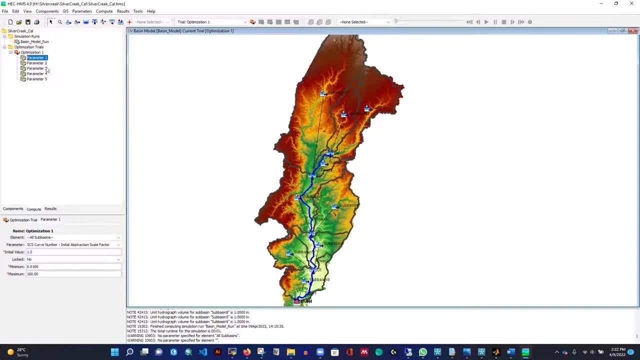 okay, so, oh, this is the factor. so, since, okay, so, oh, this is the factor. so, since it is a factor, we have to use one. no, it is a factor, we have to use one. no, it is a factor, we have to use one, no problem. and then for parameter 2, we can. 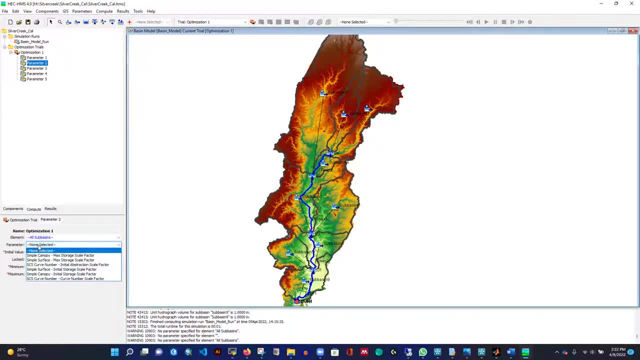 problem. and then for parameter 2 we can problem, and then for parameter 2 we can select all sub basins, and then here the select all sub basins, and then here the select all sub basins, and then here the parameter will be the next one. it says: 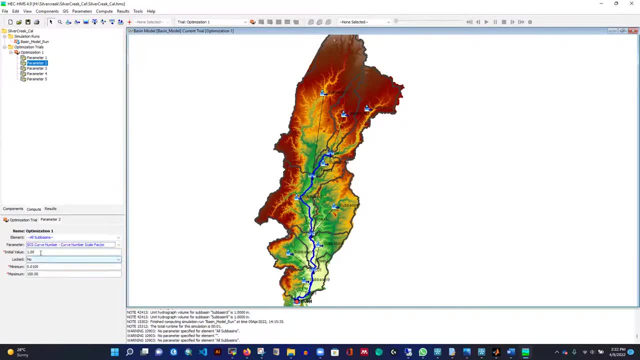 parameter will be the next one. it says parameter will be the next one. it says curve number skill factor. so initial curve number skill factor, so initial curve number skill factor. so initial factor is 1 maximum. is this minimum is. factor is 1 maximum. is this minimum is: 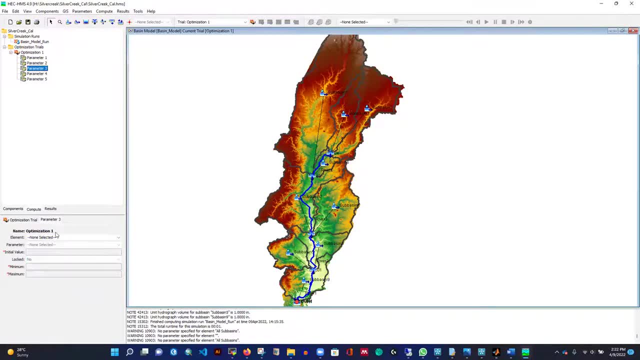 factor is 1. maximum is this, minimum is this, and now we need to add the this, and now we need to add the this, and now we need to add the muskingum. okay, so we have three. we have muskingum. okay, so we have three. we have. 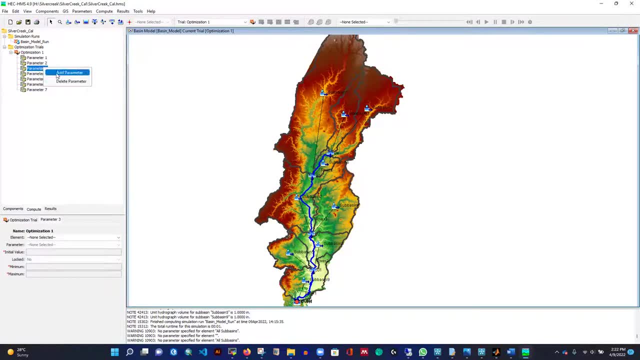 muskingum. okay, so we have three. we have to add more five like one, two, three, four. to add more five like one, two, three, four. to add more five like one, two, three, four and five. so starting from three i can and five. so starting from three, i can. 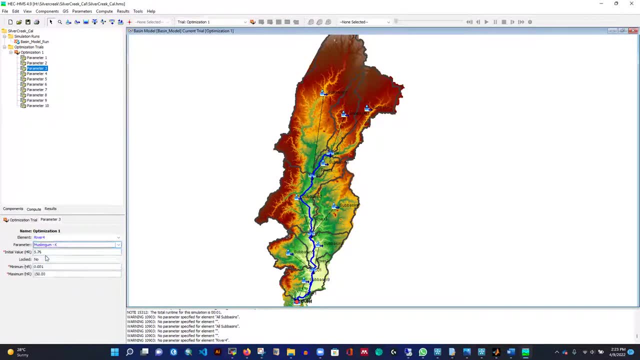 and five. so, starting from three, i can select a river one and for river one. select a river one and for river one. select a river one and for river one: muskingum x, muskingum x, muskingum x and for. okay, so the minimum hr it. 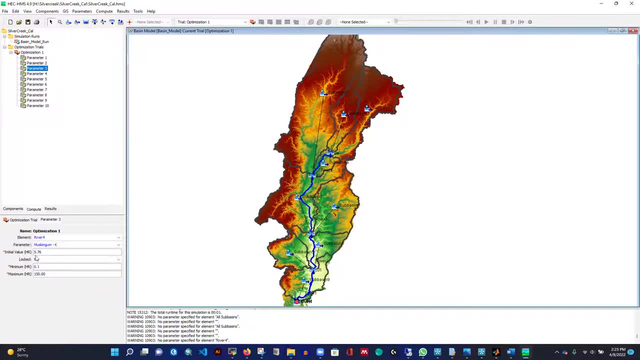 and for: okay, so the minimum hr it. and for: okay, so the minimum hr it should be like 0.1, otherwise the model should be like 0.1. otherwise the model should be like 0.1, otherwise the model won't run the initial value we have it. 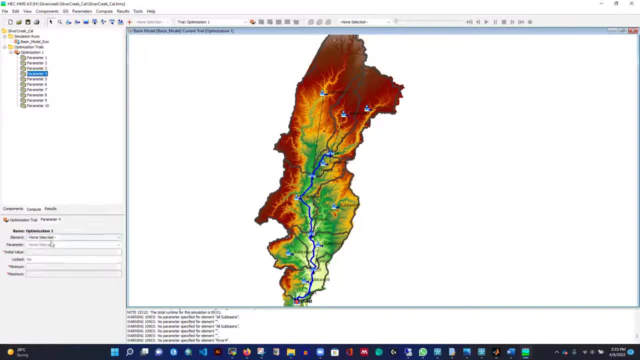 won't run the initial value we have. it won't run the initial value we have. it is this, is this, is this, and then we have like parameter four: we, and then we have like parameter four: we, and then we have like parameter four. we can select river four. 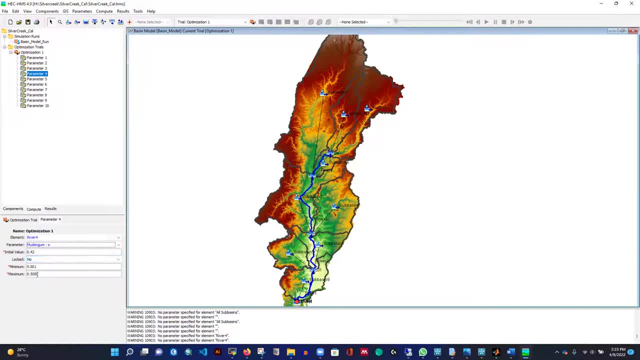 can select river four, can select river four, and then and then, and then: x- the minimum value is for two. the x- the minimum value is for two. the x- the minimum value is for two. the maximum is this okay, minimum it will. maximum is this okay, minimum it will. 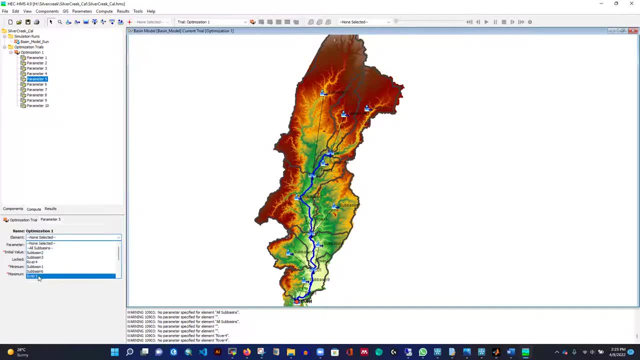 maximum is this: okay, minimum, it will work, work, work. and for this one select river three. and for this one select river three. and for this one select river three. do the same thing again, do the same thing again, do the same thing again. k, but for k, just reduce or increase the. 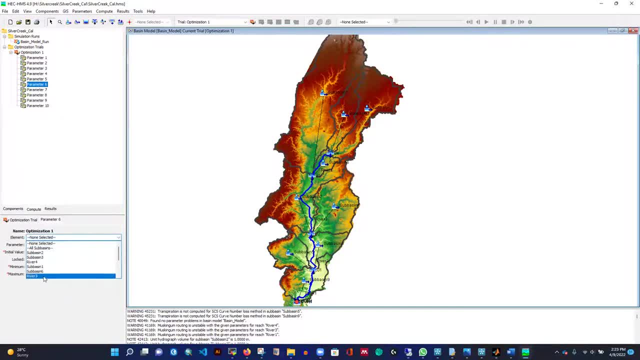 k, but for k just reduce or increase the k, but for k, just reduce or increase the time: minimum time to 0.1 time. minimum time to 0.1 time, minimum time to 0.1. and for and for and for three. we have to add another parameter x. 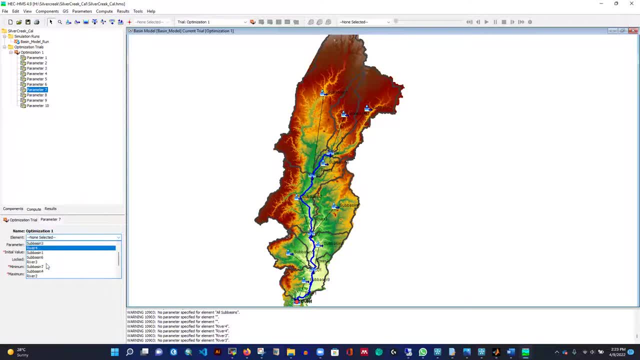 three, we have to add another parameter x. three, we have to add another parameter x, and i can keep it as it is. and i can keep it as it is, and i can keep it as it is for river two. we have two there select. for river two: we have two there select. 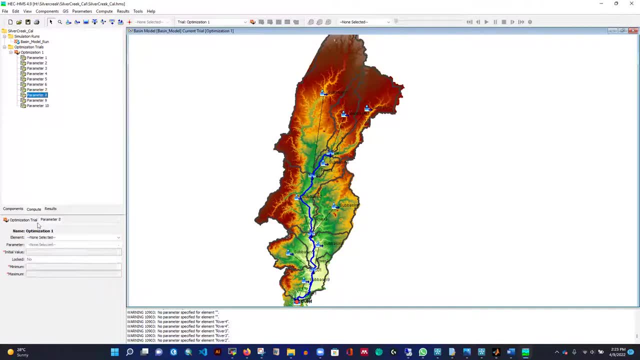 for river two. we have two there. select k- keep this value as 0.1. and for k: keep this value as 0.1. and for k: keep this value as 0.1. and for parameter eight: we can select river two. parameter eight: we can select river two. 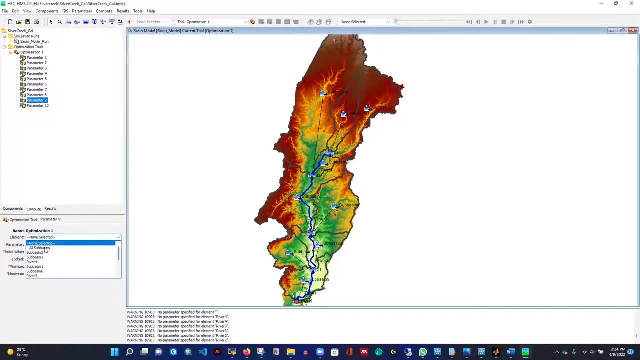 parameter eight: we can select river two, and this time we'll select x and for, and this time we'll select x and for, and this time we'll select x and for. parameter nine: we can select river one. parameter nine: we can select river one. parameter nine: we can select river one, and this will be x, and we increase that. 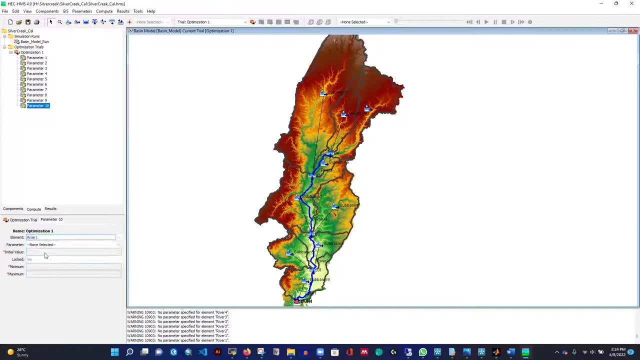 and this will be x, and we increase that, and this will be x, and we increase that to point one, to point one, to point one, and finally we have to select again and finally we have to select again and finally we have to select again river one, and that is the x. so we are. 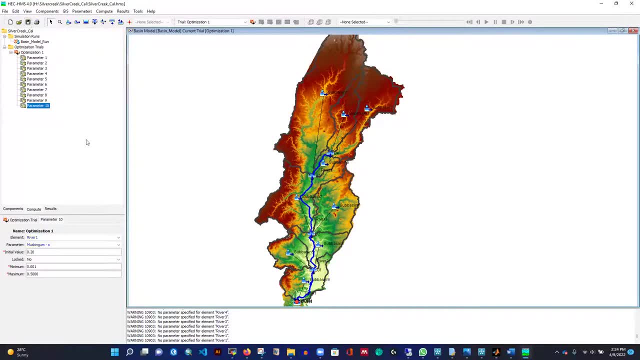 river one and that is the x. so we are river one and that is the x. so we are done with our. done with our, done with our optimization. we can set the model right. optimization, we can set the model right. optimization, we can set the model right. you can see the graph, you can remember. 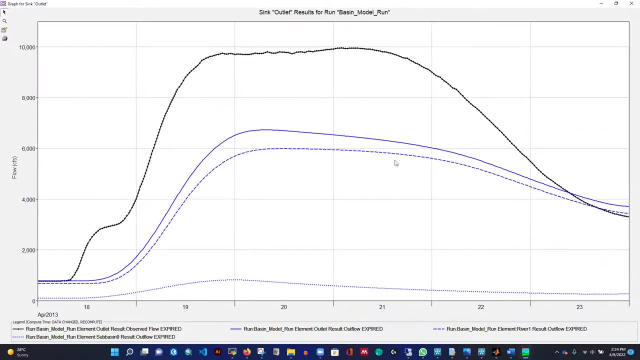 you can see the graph, you can remember, you can see the graph, you can remember that. so the current graph, we have that. so the current graph, we have that. so the current graph we have, that is the graph and we can see it. that is the graph and we can see it. 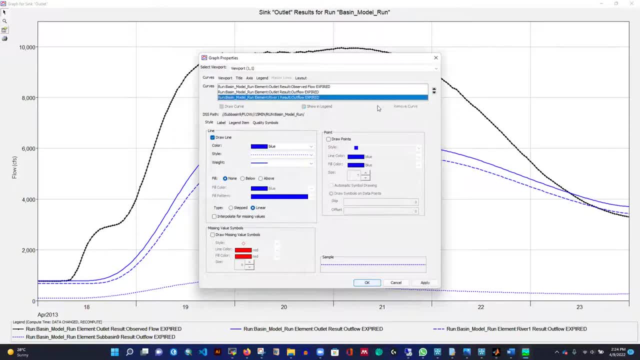 that is the graph and we can see it pretty clearly. that if you can delete pretty clearly that, if you can delete pretty clearly that, if you can delete extra, extra, extra curve- we have curve, we have curve we have here. so that's that, so that's the. 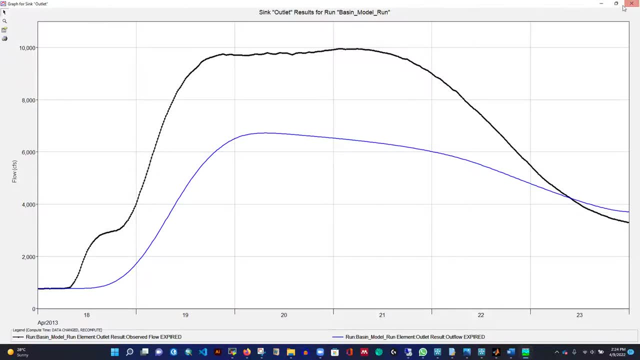 here. so that's that. so that's the here, so that's that. so that's the difference between this observation and difference between this observation, and difference between this observation and the simulation, the simulation, the simulation. okay, you can keep that in mind. okay, you can keep that in mind. 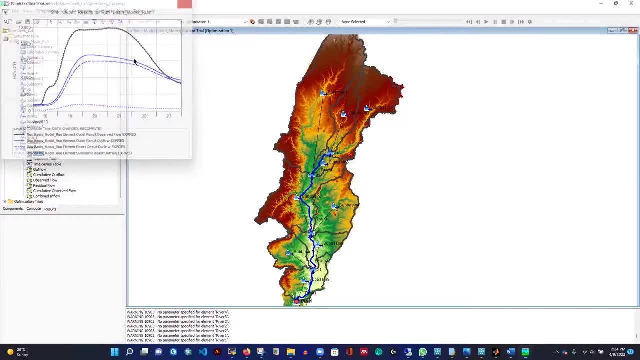 okay, you can keep that in mind, or even i can even, or even, i can even, or even i can even keep it okay. and now what we have to do? we keep it okay. and now what we have to do? we keep it okay. and now what we have to do? we don't have any. 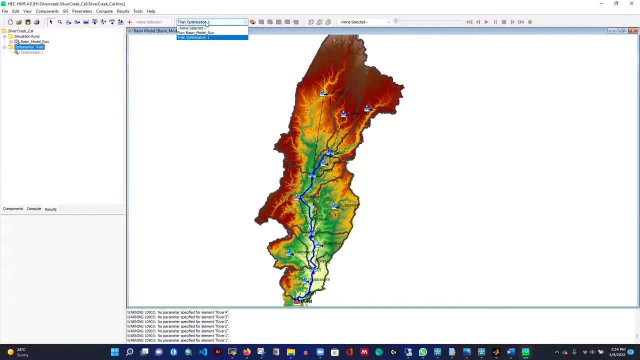 don't have any. don't have any trial run right now, right. so what do you trial run right now? right, so what do you trial run right now? right, so what do you have to do? we have to have to do, we have to have to do. we have to select that and hit it. 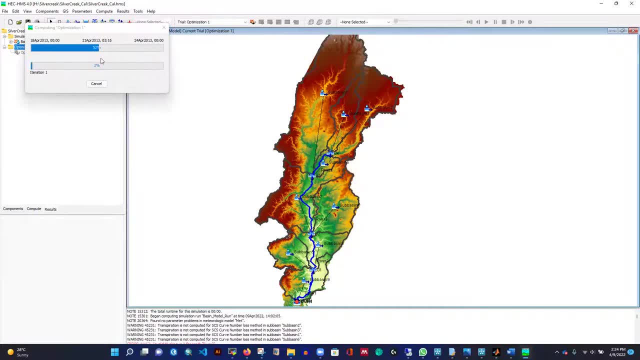 select that and hit it. select that and hit it. then it see it started the optimization. then it see it started the optimization. then it see it started the optimization process and it will take a while because process and it will take a while because process and it will take a while because we specified our maximum number of 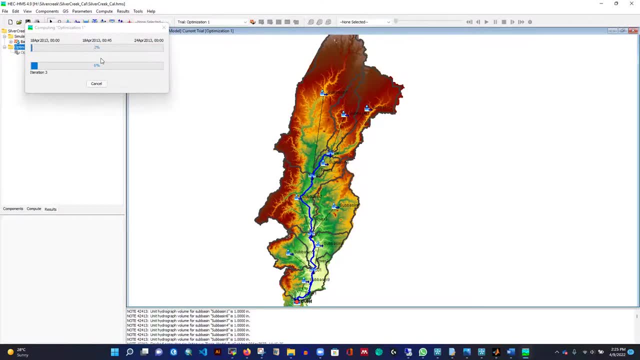 we specified our maximum number of. we specified our maximum number of iteration is 100. iteration is 100, iteration is 100 and we added all these uh calibration and we added all these uh calibration and we added all these uh calibration parameters from parameters, from parameters from uh basins- right, so we are using. 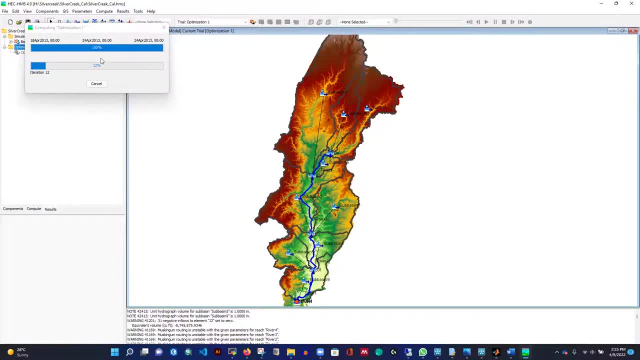 uh basins, right. so we are using uh basins, right. so we are using initial abstraction as our calibration, initial abstraction as our calibration, initial abstraction as our calibration parameter, because we don't know how much parameter, because we don't know how much parameter, because we don't know how much water will be obstructed at the very. 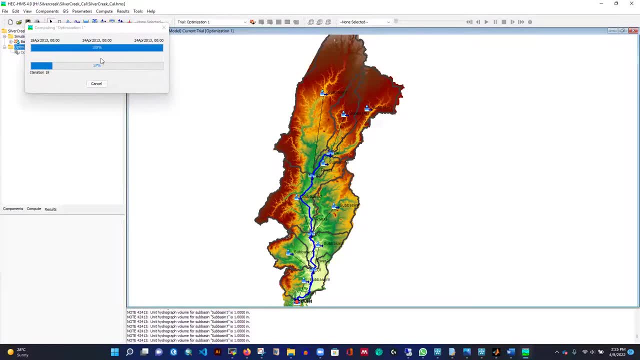 water will be obstructed at the very water will be obstructed at the very beginning of the rainfall, beginning of the rainfall, beginning of the rainfall. and we are using the curve number right and we are using the curve number right and we are using the curve number right. so we calculated the curve number from: 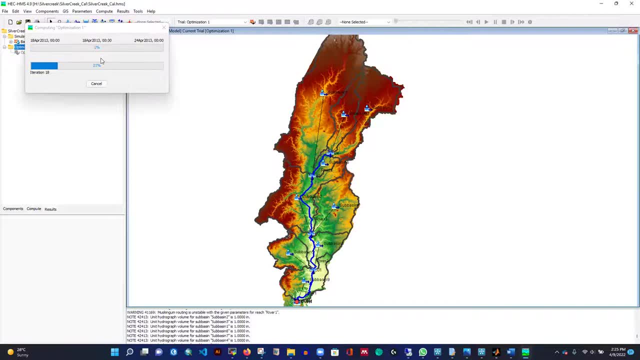 so we calculated the curve number from. so we calculated the curve number from land use and land cover information. but this is uh basically a calibration, but this is uh basically a calibration, but this is uh basically a calibration parameter, we parameter, we parameter. we are getting from the model, so we have to. 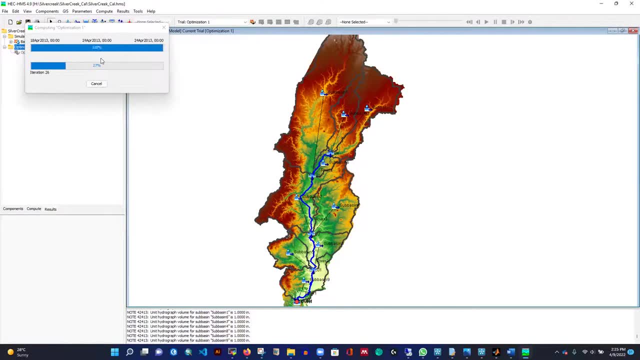 are getting from the model, so we have to are getting from the model, so we have to fix that. let's see if we can fix it. fix that, let's see if we can fix it. fix that, let's see if we can fix it. so what is basically? 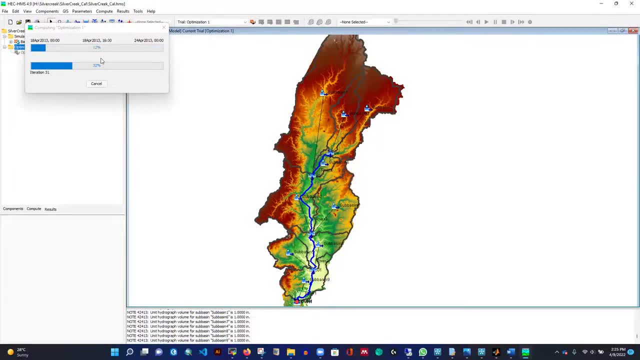 so what is basically so, what is basically we're trying to do here, we're trying to, we're trying to do here, we're trying to, we're trying to do here, we're trying to match the observation with the match, the observation with the match, the observation with the calibration. 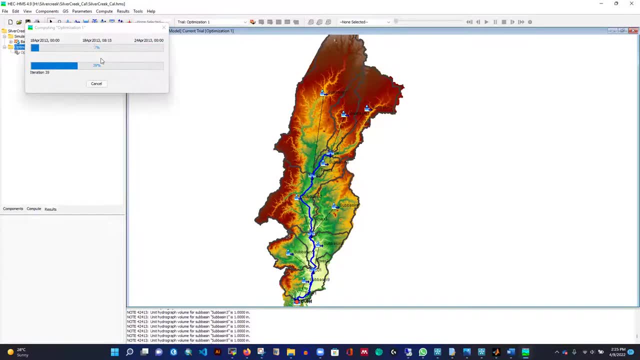 calibration, calibration- yeah with the observation with the model. yeah with the observation with the model, yeah with the observation with the model. uh generated in the hydrograph, but uh generated in the hydrograph, but uh generated in the hydrograph. but if you see right, previously you saw the 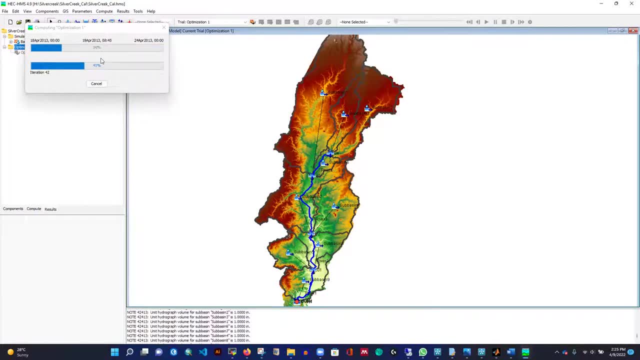 if you see right- previously you saw the. if you see right previously, you saw the. peak is pretty flat, peak is pretty flat, peak is pretty flat. so it's even challenging because we know so. it's even challenging because we know so. it's even challenging because we know the typical. 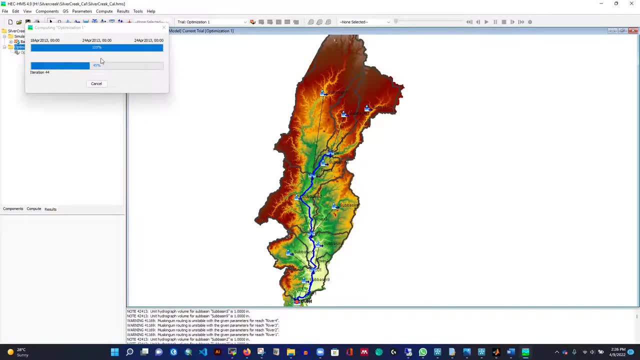 the typical. the typical uh shape of a hydrograph is basically a uh shape of a hydrograph is basically a uh shape of a hydrograph is basically a flat hydrograph. i'm talking about the flat hydrograph. i'm talking about the flat hydrograph. i'm talking about the flat hydrograph. 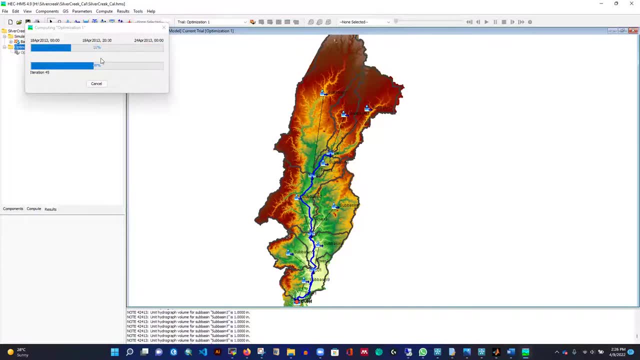 flat hydrograph, flat hydrograph. so we have the. so we have the. so we have the rising limb. we have a recession limb, rising limb. we have a recession limb, rising limb. we have a recession limb. and we have the peak and we have the peak and we have the peak right. but for this case the peak is pretty. 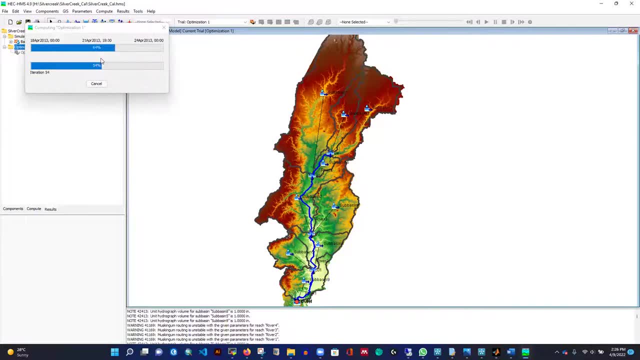 right, but for this case the peak is pretty right. but for this case the peak is pretty flat, so it's challenging. pretty flat, so it's challenging, pretty flat, so it's challenging, pretty challenging to capture, challenging to capture, challenging to capture. so we have to even try. 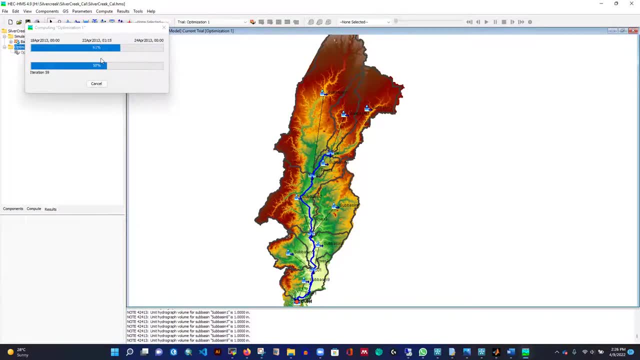 so we have to even try. so we have to even try, and if you can, and if you can, and if you can, use a manual and automatic, use a manual and automatic, use a manual and automatic calibration. that is calibration. that is calibration that is currently going on. we can even capture. 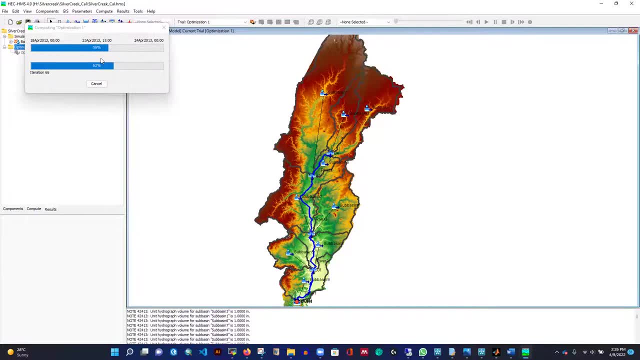 currently going on, we can even capture. currently going on, we can even capture it, so i'm not gonna even show you this. it so i'm not gonna even show you this. it, so i'm not gonna even show you this. automatic calibration over and over. automatic calibration over and over. 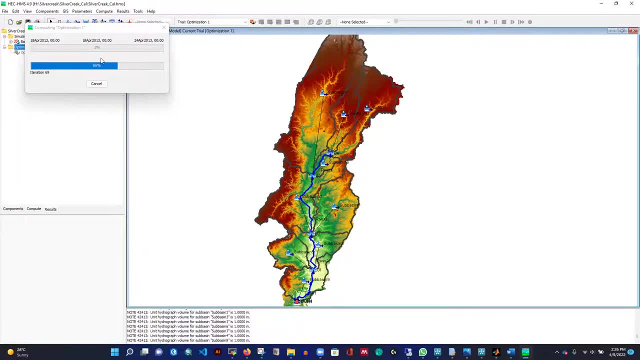 automatic calibration over and over, because i'm gonna use it for the first. because i'm gonna use it for the first, because i'm gonna use it for the first time time time here, and then i'll use manual calibration here and then i'll use manual calibration. 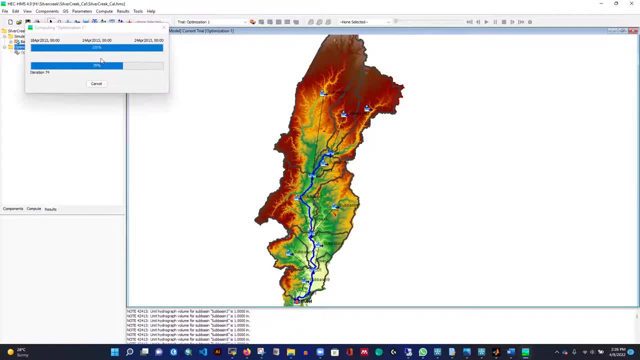 here, and then i'll use manual calibration, otherwise it will take a lot of time, but otherwise it will take a lot of time, but otherwise it will take a lot of time. but you can try, you can try. you can try now, both like now, both like now, both like first, use that automatic calibration, get. 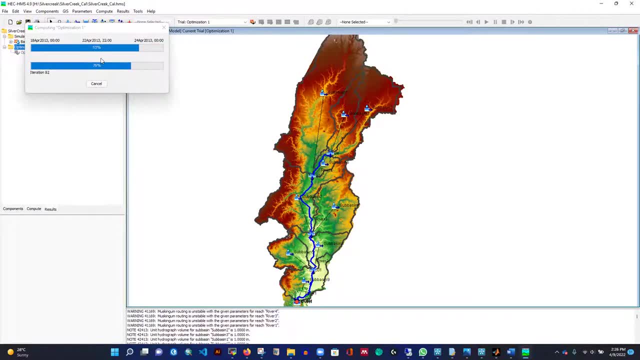 first, use that automatic calibration, get first. use that automatic calibration, get the parameter, the parameter, the parameter, and then use it in into your model and and then use it in into your model and and then use it in into your model and then, then, then change the parameter manually and then. 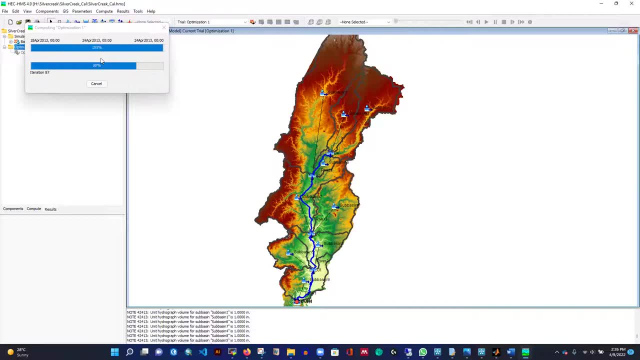 change the parameter manually and then change the parameter manually and then check it, and again you can even check it, and again, you can even check it, and again you can even run your automatic calibration both way. run your automatic calibration both way. run your automatic calibration both way, you can. 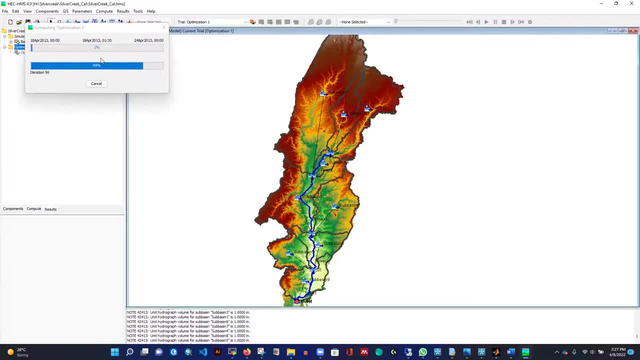 you can. you can even do that. that will even give you more even. do that. that will even give you more even. do that. that will even give you more accurate results. but for the accurate results, but for the accurate results, but for the sake of time, i'm not gonna make the 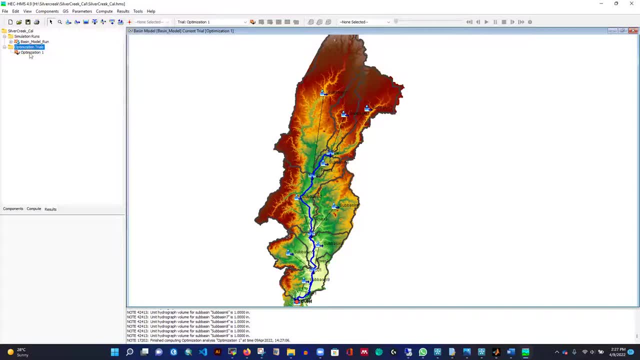 sake of time. i'm not gonna make the sake of time. i'm not gonna make the longer video, so we are done. so that's longer video, so we are done. so that's longer video, so we are done so. that's why i'm just running. so whatever we. 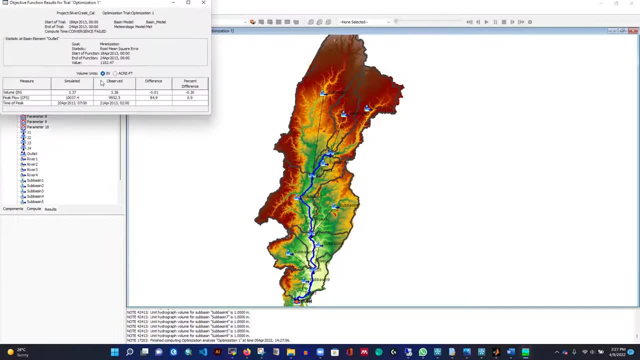 why i'm just running. so, whatever we, why i'm just running. so, whatever we have, let's check the results. have. let's check the results, have. let's check the results. so let's see the objective function: the. so let's see the objective function, the. so let's see the objective function, the objective function. 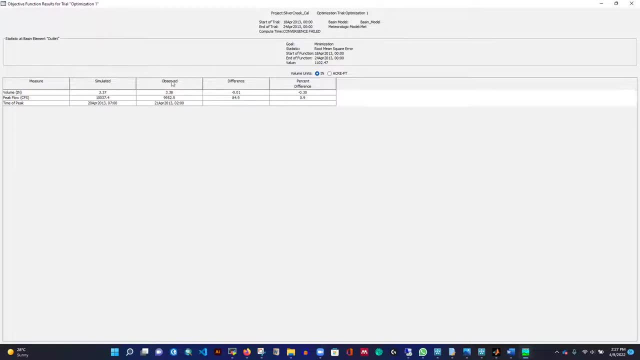 objective function. objective function: we are getting here. see the simulated we are getting here. see the simulated we are getting here. see, the simulated value is basically 3.37 and the object value is basically 3.37, and the object value is basically 3.37 and the object value is 3.38. so it is pretty close. 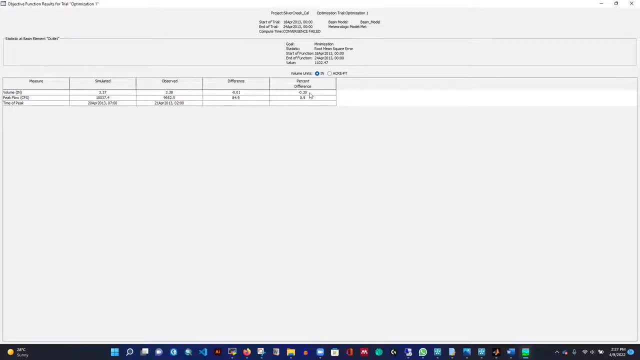 value is 3.38, so it is pretty close. value is 3.38, so it is pretty close, right, so the difference is nearly zero. right so the difference is nearly zero, right so the difference is nearly zero. and we have this percentage: 0.3 it's. 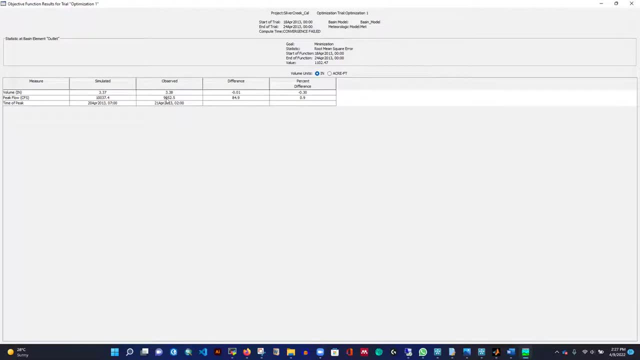 and we have this percentage 0.3. it's, and we have this percentage 0.3, it's pretty good, pretty good, pretty good. and see the observation: we have 10 000 and see the observation: we have 10 000 and see the observation: we have 10 000 and we have nine, almost ten thousand. 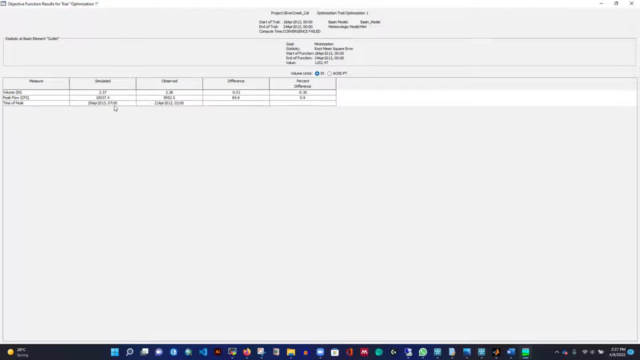 and we have nine, almost ten thousand, and we have nine, almost ten thousand, right nine thousand nine hundred and right nine thousand nine hundred and right nine thousand nine hundred and fifty two, fifty two, fifty two. and we have a little difference between, and we have a little difference between 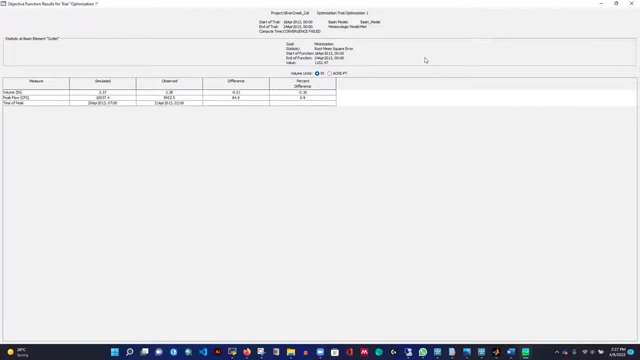 and we have a little difference between the peak time, that's okay. the peak time, that's okay. the peak time: that's okay because the shape is a little bit, because the shape is a little bit, because the shape is a little bit different, different, different. so, in terms of this, 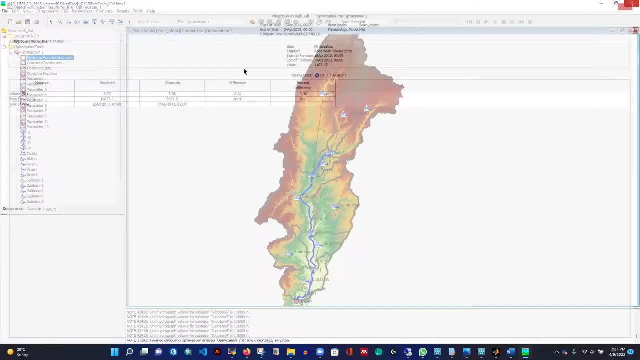 so in terms of this, so in terms of this, it is looking like the volume. it is looking like the volume. it is looking like the volume is pretty accurate. but what about? the is pretty accurate, but what about? the is pretty accurate, but what about the shape? and we can see the optimized. 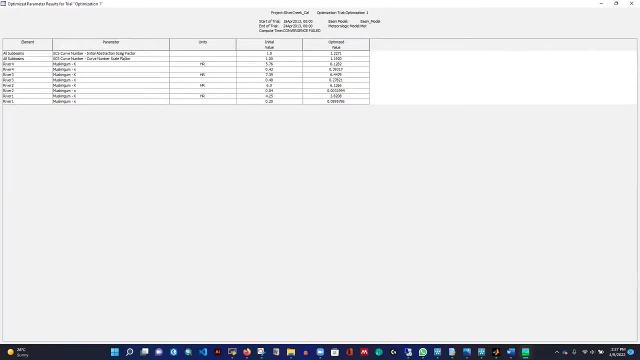 shape and we can see the optimized shape and we can see the optimized parameter, parameter, parameter. we can see if initially the initial, we can see if initially the initial, we can see if initially the initial obstruction value, whatever value we had, obstruction value, whatever value we had, obstruction value, whatever value we had, it doesn't matter, it assumed. 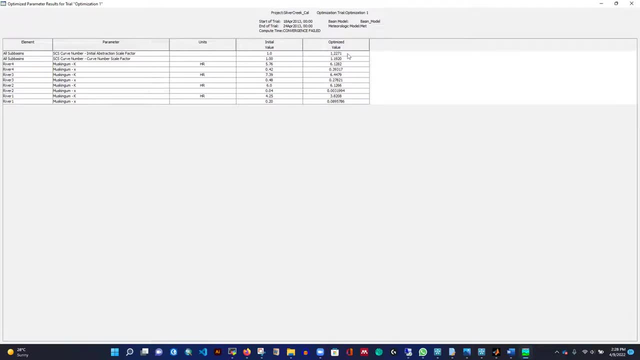 it doesn't matter, it assumed. it doesn't matter, it assumed as one and it is giving us the option as one and it is giving us the option as one and it is giving us the option that okay, if you want to, that okay if you want to. 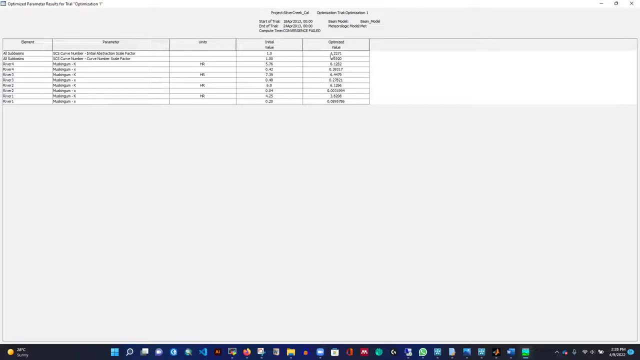 that okay, if you want to get the result that we just saw- we have get the result that we just saw, we have get the result that we just saw- we have to multiply that value by this one, and to multiply that value by this one, and to multiply that value by this one, and for curve number, we have to even. 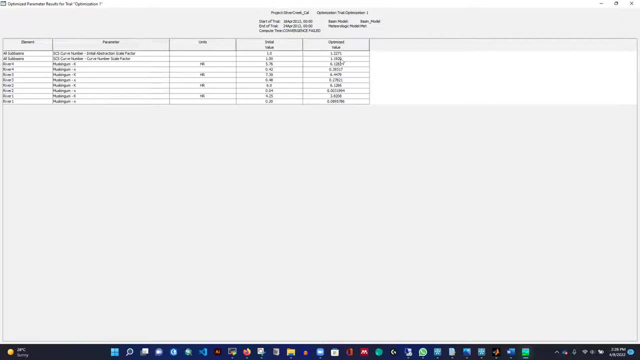 for curve number, we have to even for curve number, we have to even increase it as, increase it as, increase it, as, like one point it's like 90 percent, and like one point it's like 90 percent, and like one point it's like 90 percent, and for 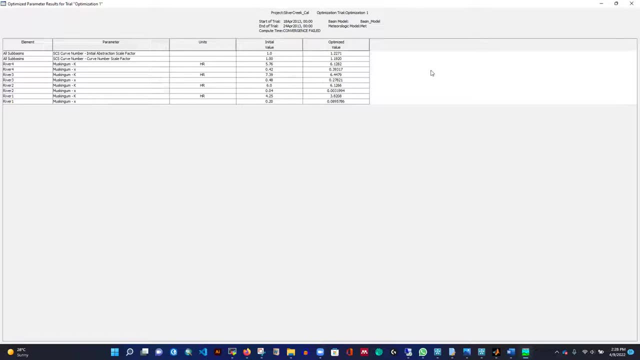 for, for this one, we have to increase it, and we, this one, we have to increase it, and we, this one, we have to increase it. and we have to change these values like that, have to change these values like that, have to change these values like that. we'll do that, okay, no problem. 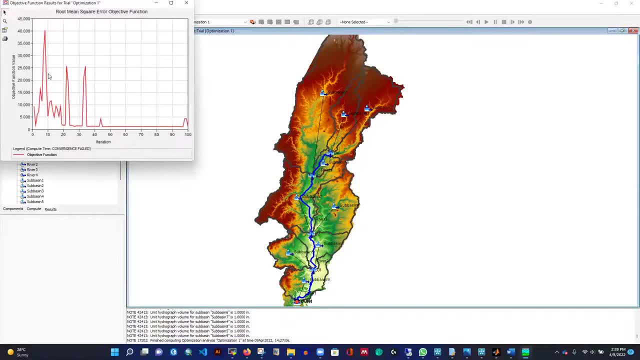 we'll do that, okay, no problem. we'll do that, okay, no problem. so let's see the, so let's see the. so let's see the function objective function. so initially it function objective function. so initially it function objective function. so initially it was just kind of. 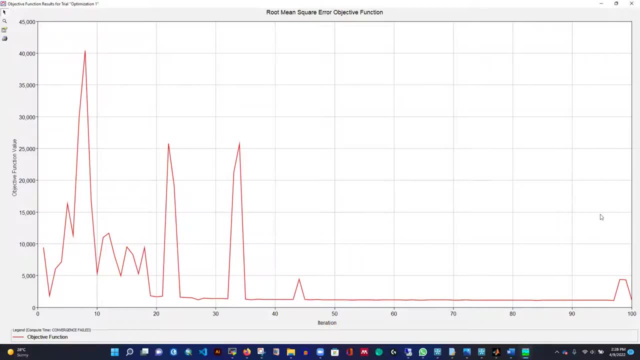 was just kind of was just kind of changing, and then it became like stable changing, and then it became like stable changing, and then it became like stable, right, right, right. so let's see the plot, so let's see the plot, so let's see the plot outlet. okay, because we are calibrating the 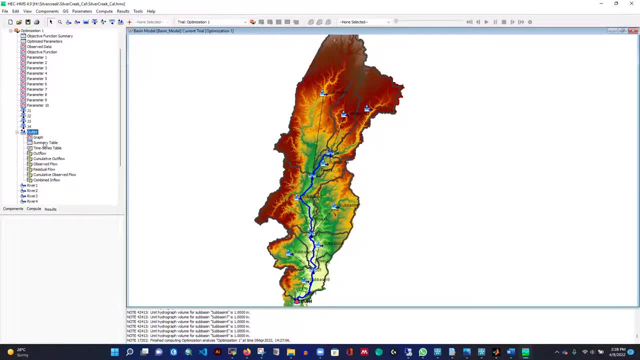 outlet. okay, because we are calibrating the outlet. okay, because we are calibrating the model at the outlet. model at the outlet. model at the outlet means here, so at first check the graph. means here, so at first check the graph. means here, so at first check the graph. if it is can, oh man, it's really good. 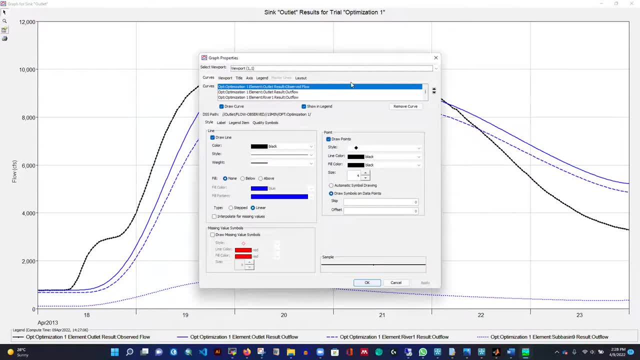 if it is can, oh man, it's really good. if it is can, oh man, it's really good. see, it's really good, right, yeah? so see, it's really good, right, yeah, so see, it's really good, right, yeah. so that's why i like automatic calibration. 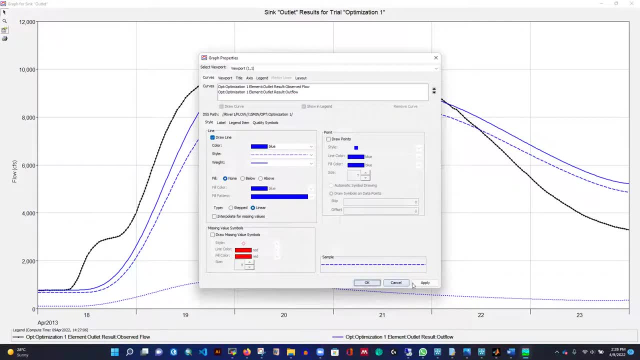 that's why i like automatic calibration. that's why i like automatic calibration. so i'm removing the extra plot we have. so i'm removing the extra plot we have. so i'm removing the extra plot we have. okay, so, okay, so, okay. so that is the plot. 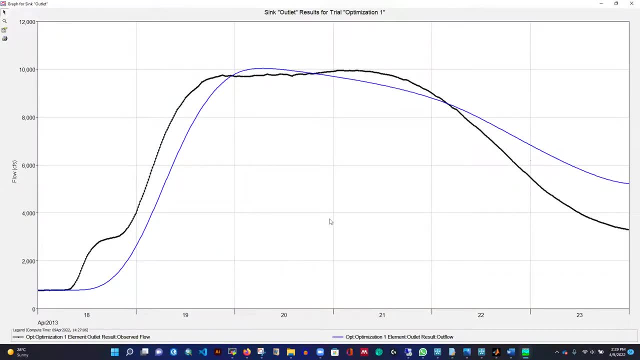 that is the plot. that is the plot. we need to capture it. it's pretty good, we need to capture it. it's pretty good, we need to capture it. it's pretty good. see, see, see, but we need to even fix this, that's okay. but we need to even fix this, that's okay. 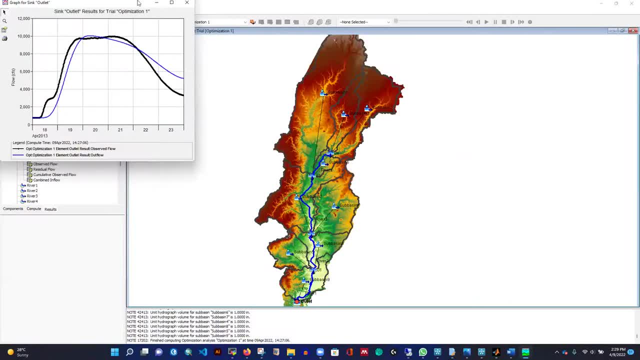 but we need to even fix this. that's okay. but it is capturing almost capturing, but it is capturing almost capturing, but it is capturing, almost capturing, right the volume it captured, right the volume it captured, right the volume it captured. and we can check the summary table. and we can check the summary table. 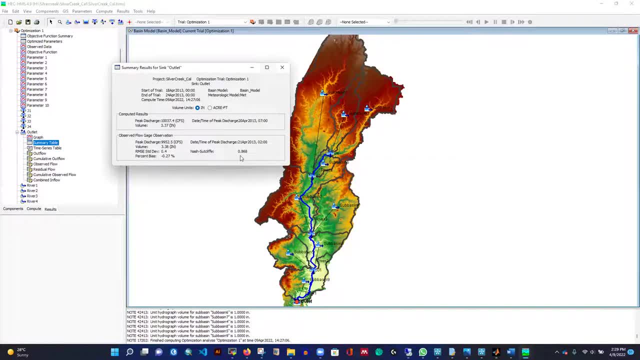 and we can check the summary table and oh man, it's really good and oh man, it's really good and oh man, it's really good. so 8: 0.86 from 0.26 to 0.86. so 8: 0.86 from 0.26 to 0.86. 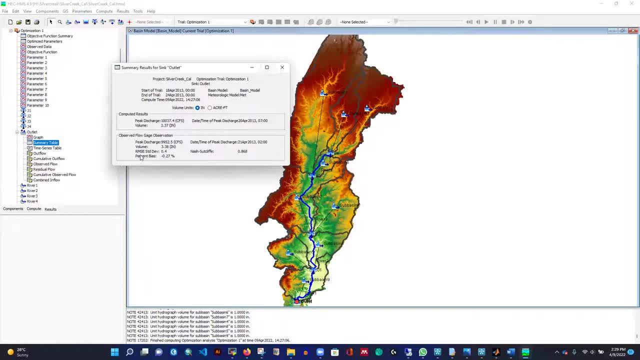 so 8: 0.86 from 0.26 to 0.86. it's really good and we can see the. it's really good and we can see the. it's really good and we can see the percent bias is like 0.27. 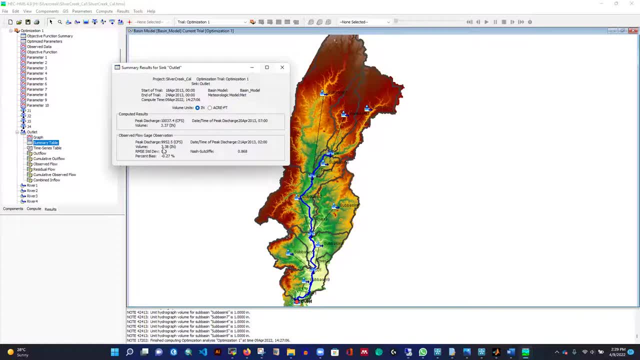 percent bias is like 0.27 percent bias is like 0.27 right and the peak. we know already that right and the peak. we know already that right and the peak. we know already that the, the, the observation, it has like 0.3.38 inch. 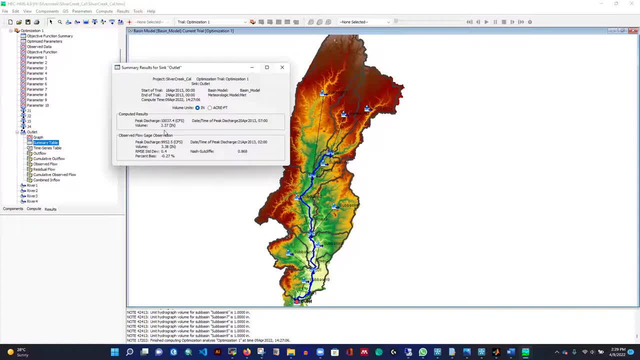 observation, it has like 0.3.38 inch observation. it has like 0.3.38 inch. however, from simulation, we are getting, however, from simulation, we are getting, however, from simulation, we are getting 3.37, 3.37, 3.37. it's really good. 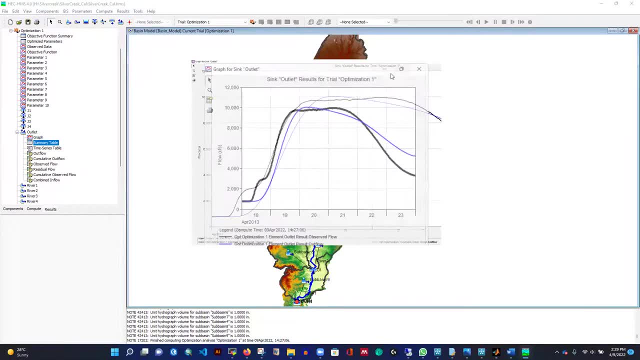 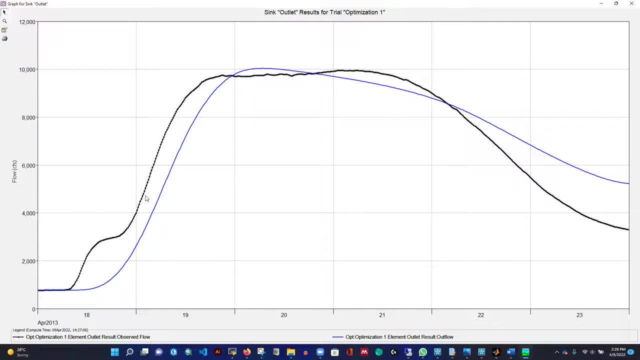 it's really good. it's really good what we have here. we have some what we have here. we have some what we have here. we have some time shift here. we have to even capture time shift here. we have to even capture time shift here. we have to even capture this rising limp, otherwise we have a 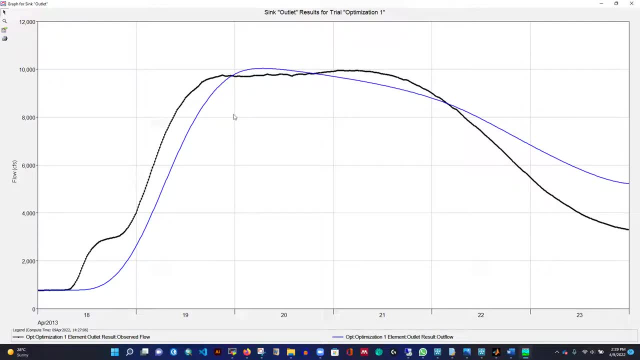 this rising limp, otherwise we have a this rising limp, otherwise we have a delay, delay, delay. right, this right, this right. this blue line is basically blue line is basically blue line is basically using more time to concentrate. that's using more time to concentrate. that's using more time to concentrate. that's why we have to reduce the time of 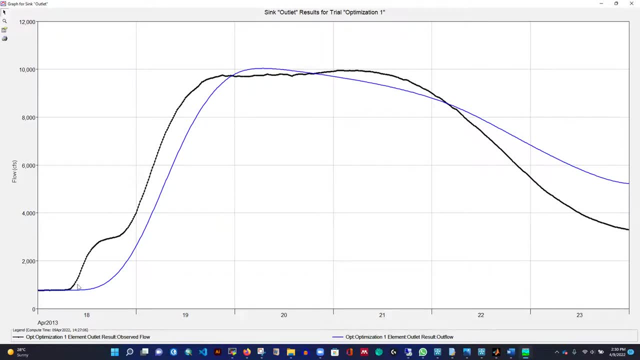 why we have to reduce the time of, why we have to reduce the time of concentration, concentration, concentration. so from this, so from this, so from this plot we can see plot, we can see plot, we can see we need to shift this graph from here to. we need to shift this graph from here to. 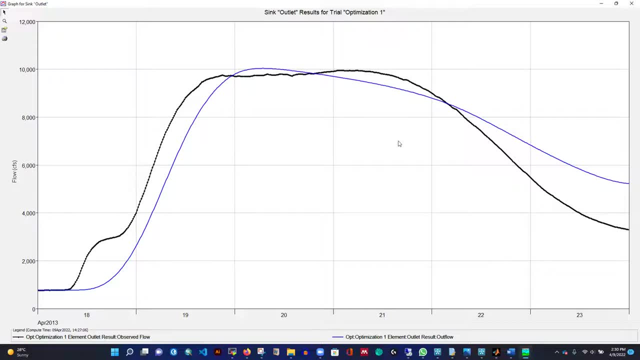 we need to shift this graph from here to there, so we don't need to there. so we don't need to there, so we don't need to lose any water other than losing any lose any water other than losing any lose any water other than losing any water. so we we're done with loss factor. 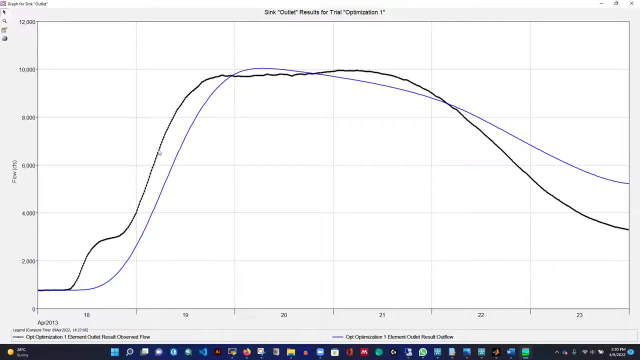 water. so we we're done with loss factor water. so we we're done with loss factor. so what we'll do next time, we'll even so. what we'll do next time, we'll even. so, what we'll do next time, we'll even use, use, use, calibration. 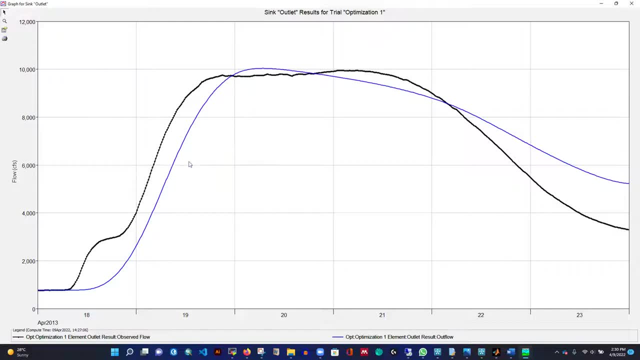 calibration: calibration for, for, for the, the, the clark unit hydrograph. the transform clark unit hydrograph. the transform clark unit hydrograph. the transform method. because we need to transform the method, because we need to transform the method, because we need to transform the depth of. 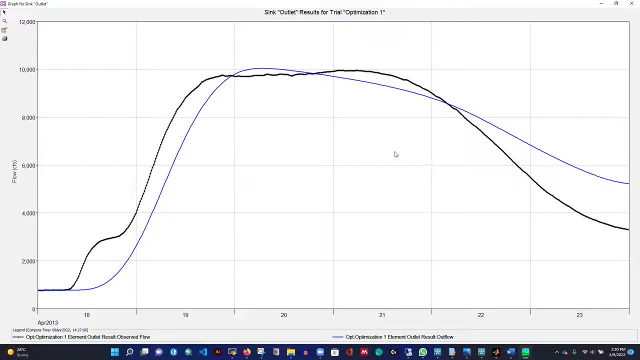 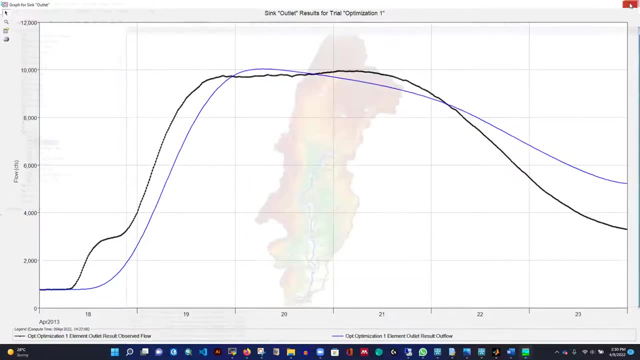 rainfall into rainfall, into rainfall, into this hydrograph flow rate, so this hydrograph flow rate, so this hydrograph flow rate. so transform method will do the job, transform method will do the job. transform method will do the job, but before that, what we have to do, because 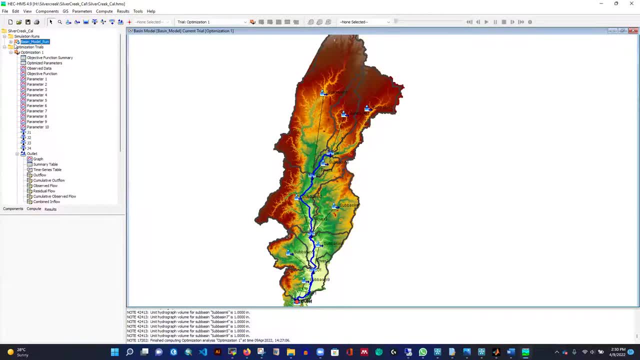 but before that, what we have to do because, but before that, what we have to do, because our model main simulation is not our model main simulation is not our model main simulation is not capturing this shape. this is our main capturing this shape. this is our main capturing this shape, this is our main model. 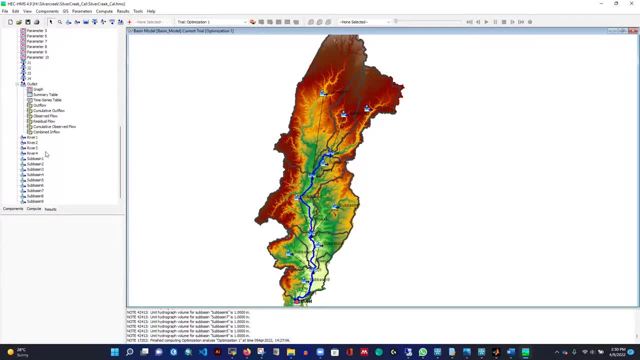 model, model. we have this shape, we have this shape, we have this shape, but from optimization, but from optimization, but from optimization, we're, we're, we're getting this one, so we have to getting this one, so we have to getting this one, so we have to be able to get this. 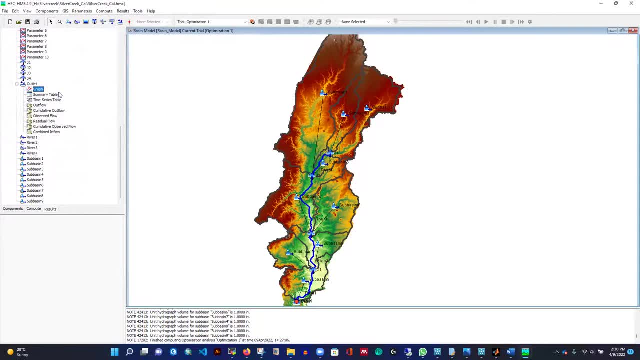 be able to get this, be able to get this right. we have to be able to accept this right. we have to be able to accept this right. we have to be able to accept this. graph, graph, graph from our simulation. so how can i? from our simulation. so how can i? 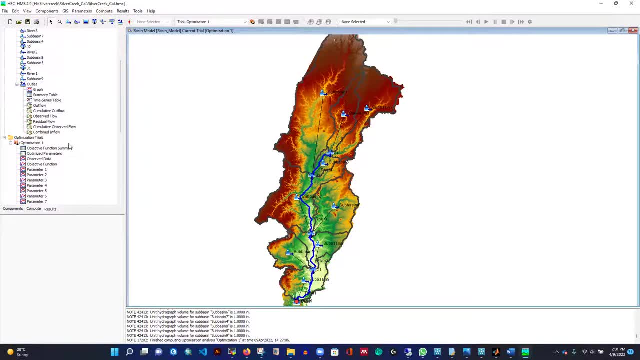 from our simulation. so how can i do that? do that, do that. so that is the thing i'm going to show. so that is the thing i'm going to show. so that is the thing i'm going to show you. we have the function, we have the. 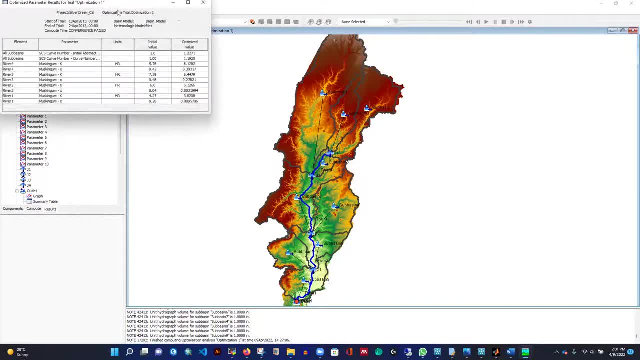 you, we have the function, we have the you, we have the function, we have the values: optimized values, optimized values, optimized parameters. so keep that in mind there. parameters, so keep that in mind, there, parameters. so keep that in mind there and go to your component and then model. 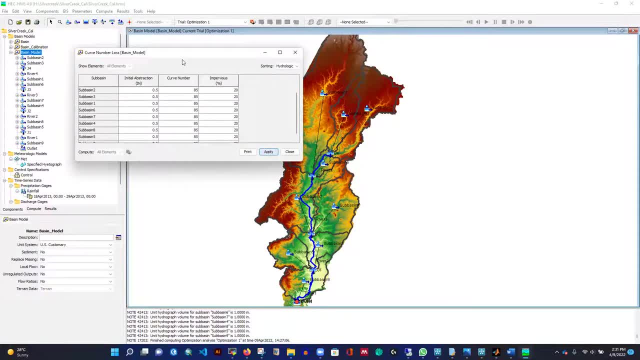 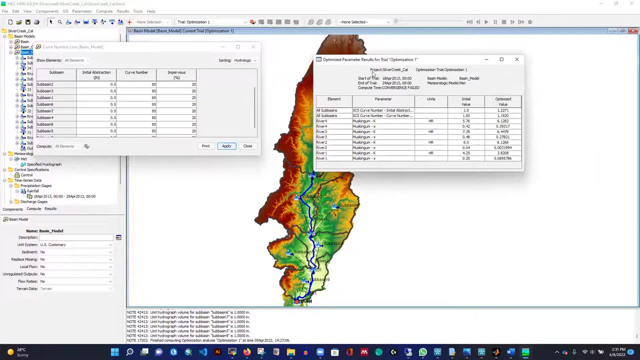 and go to your component, and then model and go to your component, and then model, go to parameter and the loss factor go to parameter and the loss factor go to parameter and the loss factor here. okay, open that here. okay, open that here. okay, open that optimized parameter. so what we have to do, 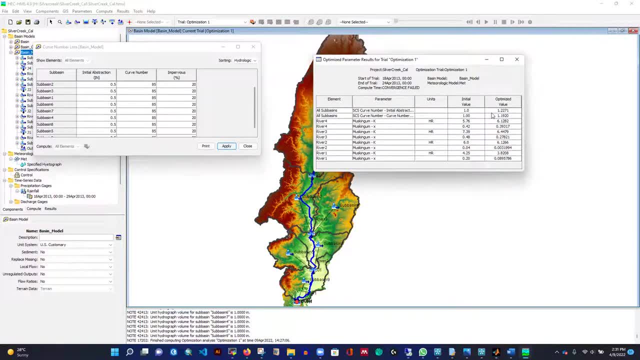 optimized parameter. so what we have to do, optimized parameter. so what we have to do, we have to change it for the first one, we have to change it for the first one, we have to change it for the first one: initial obstruction, we have to multiply. initial obstruction, we have to multiply. 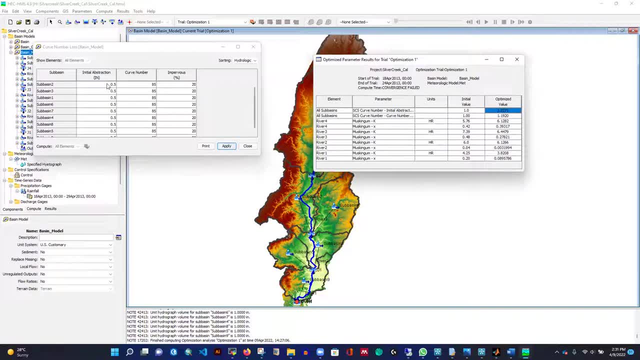 initial obstruction. we have to multiply these values 1.2271, so this one. these values 1.2271, so this one. these values 1.2271, so this one will be multiplied by 1.2271, will be multiplied by 1.2271. 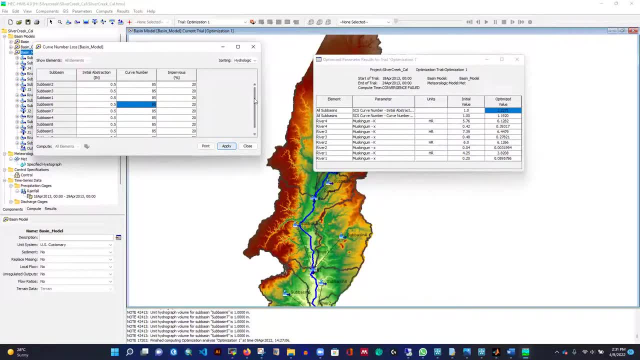 will be multiplied by 1.2271. so select that. so select that. so select that 1.2271. select that and click on fill. select that and click on fill. select that and click on fill. multiply, multiply. multiply by constant 1.2271, so it will be. 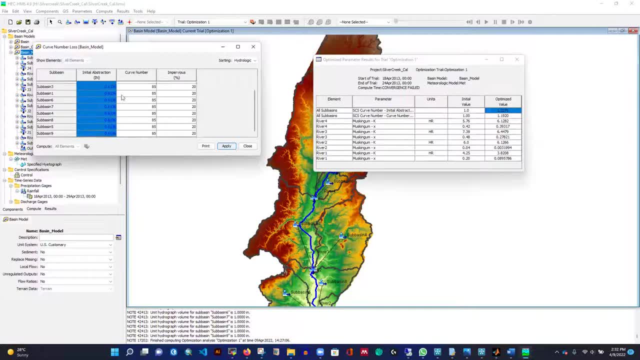 by constant 1.2271, so it will be by constant 1.2271. so it will be multiplied by this value to all of this, multiplied by this value to all of this, multiplied by this value to all of this. so now we are getting this one. 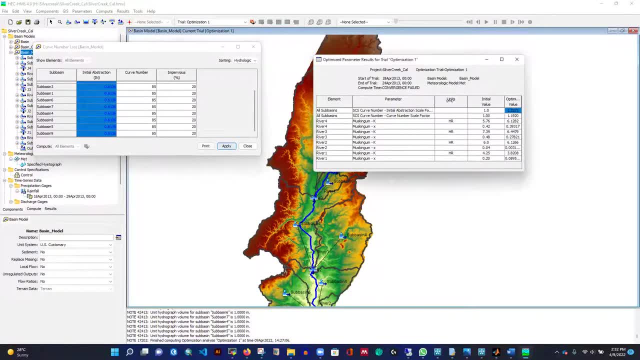 so now we are getting this one, so now we are getting this one. another one is that curve number- okay. another one is that curve number- okay. another one is that curve number- okay, this one, this one, this one. curve number scale factor, so this curve. curve number scale factor, so this curve. 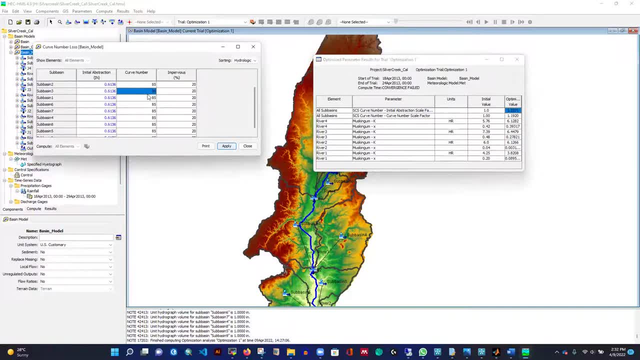 curve number scale factor. so this curve number should be multiplied by number, should be multiplied by number. should be multiplied by 1.920. so select all this 1.920. so select all this 1.920. so select all this curve number at once and right click. 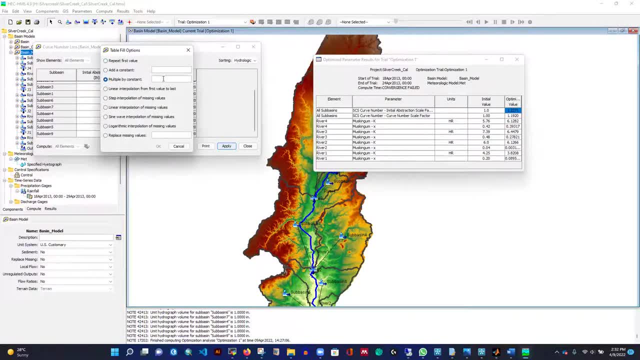 curve number at once and right click curve number at once and right click and fill and again multiply by a and fill and again multiply by a and fill and again multiply by a constant. that will be 1.1. constant: that will be 1.1. 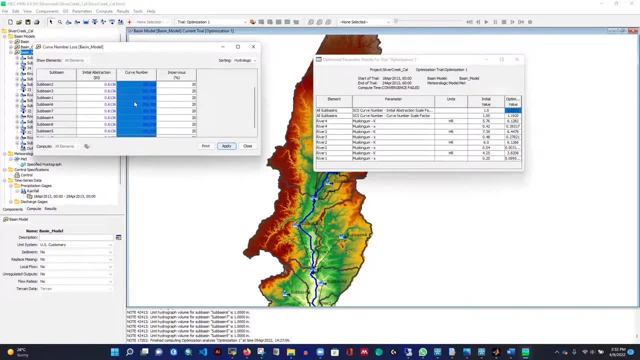 constant, that will be 1.1 r9 t. okay, and then we have this r9 t okay, and then we have this r9 t okay, and then we have this. but see, it's not even we know the limit. but see, it's not even we know the limit. 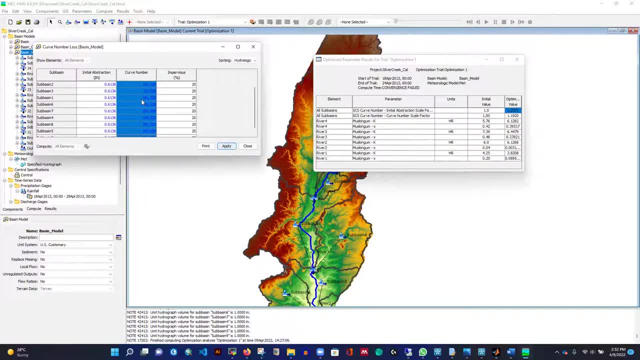 but see, it's not even we know. the limit of curve number should be of curve number, should be of curve number should be within, within, within 100. so it is not realistic, right 100. so it is not realistic, right 100. so it is not realistic, right. so what do you have to do? 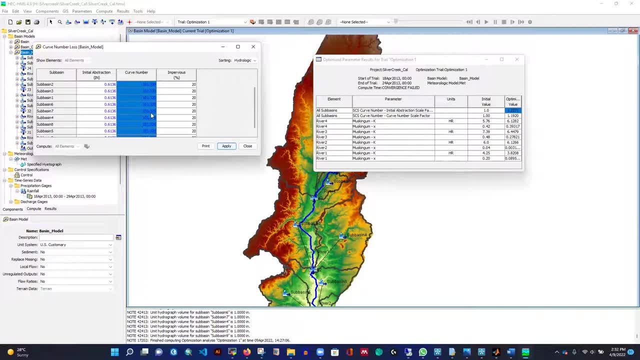 so what do you have to do? so, what do you have to do, even though the optimization it doesn't, even though the optimization it doesn't, even though the optimization it doesn't have that idea on that, have that idea on that, have that idea on that. so what it? 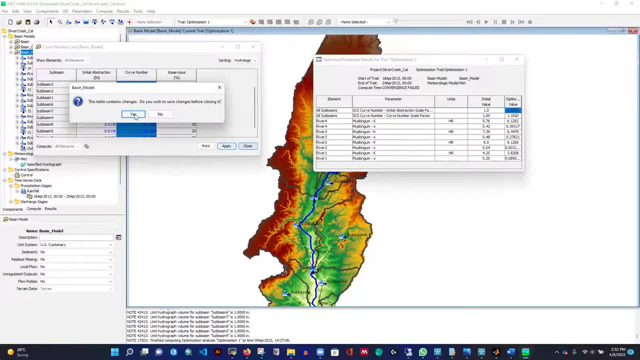 so what it, so what it? did we have to change it? okay, did we have to change it? okay, did we have to change it? okay, okay, so, okay, so, okay. so i'm just canceling the. okay, i cancel. i'm just canceling the. okay, i cancel. 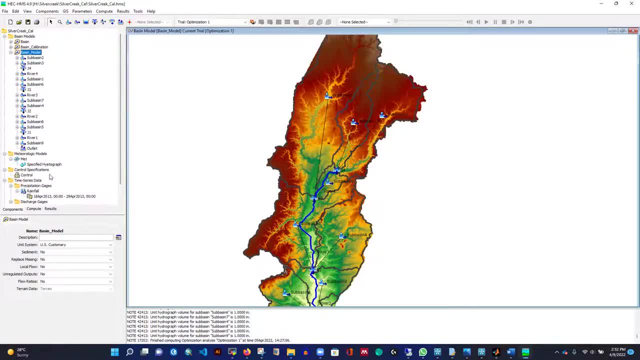 i'm just canceling the. okay, i cancel that, that, that, and i have to change it, and i have to change it and i have to change it. go back to your. go back to your. go back to your computation. the parameter we use the computation. the parameter we use the. 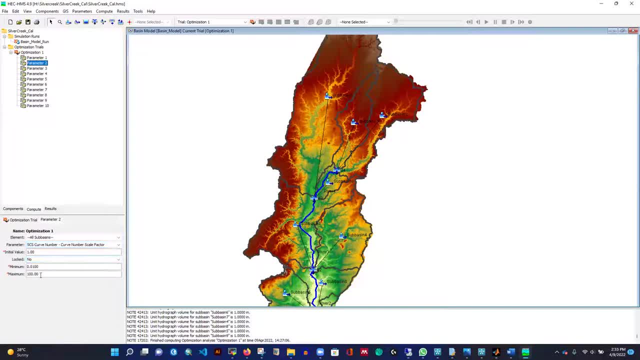 computation, the parameter we use. the second one probably the curve number. second one, probably the curve number. second one, probably the curve number here, see, even though it's one, here, see, even though it's one here, see, even though it's one means initial is one the value we are. 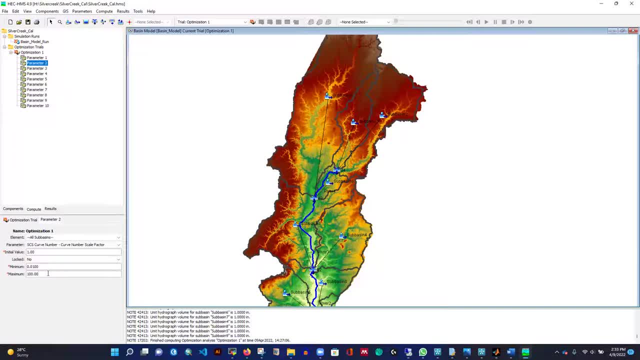 means initial is one the value we are means initial is one. the value we are using and the maximum is 100 using and the maximum is 100 using and the maximum is 100. this is basically the factor, not the. this is basically the factor, not the. 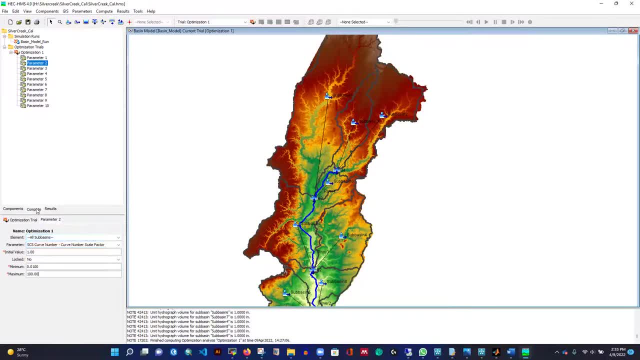 this is basically the factor, not the value. that's why it is going to give us value. that's why it is going to give us value. that's why it is going to give us that, that, that abrupt number. if you multiply that so abrupt number, if you multiply that so. 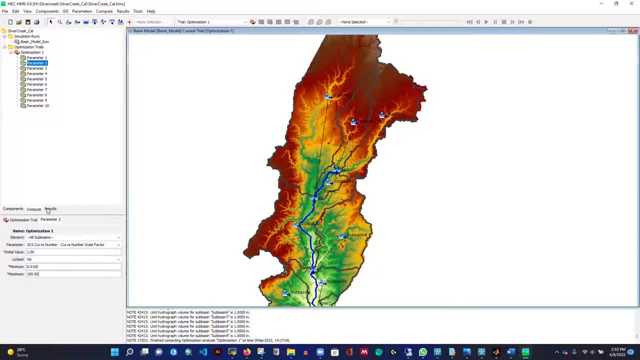 abrupt number if you multiply that. so you have to even think about that. okay, you have to even think about that. okay, you have to even think about that. okay, my maximum value of curve number is 100. my maximum value of curve number is 100. my maximum value of curve number is 100. i can. 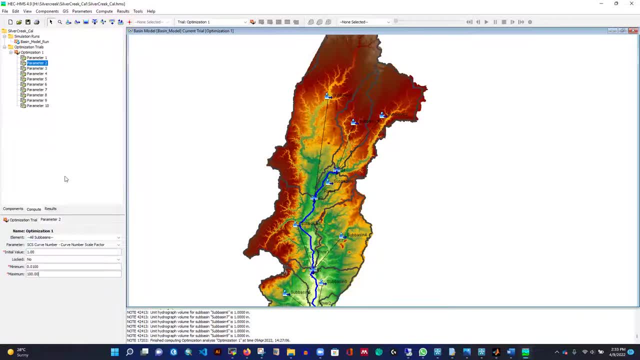 i can, i can, i cannot go beyond that. so if you use, i cannot go beyond that. so if you use, i cannot go beyond that. so if you use that more than 100, the model on run that more than 100, the model on run that more than 100, the model on run, so 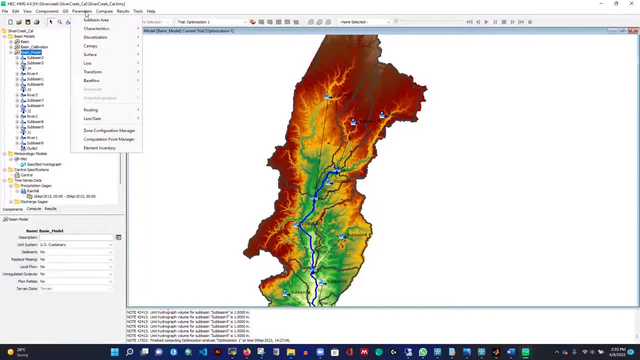 so. so again, i'm going to open the, again i'm going to open the, again i'm going to open the parameters, parameters, parameters, loss factor, loss factor, loss factor. so, instead of changing that because i so, instead of changing that because i so, instead of changing that because i know from the 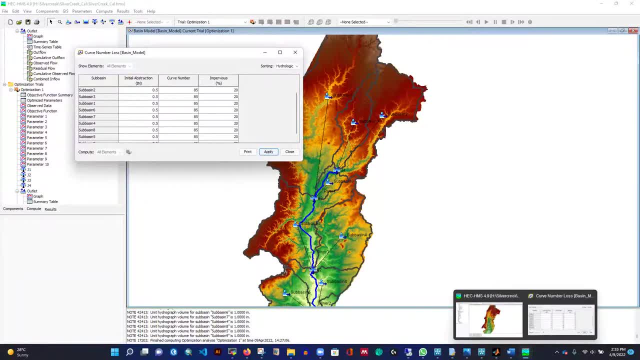 know, from the know, from the optimization right, that optimization right, that optimization right, that it is going to be, it is going to be, it is going to be more than whatever value we have, and it more than whatever value we have, and it more than whatever value we have, and it has to be increased. 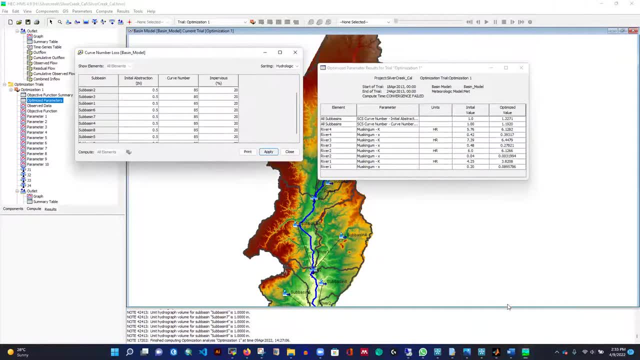 has to be increased, has to be increased. so this is my optimized parameter. so this is my optimized parameter, so this is my optimized parameter, and these are my curve number so at, and these are my curve number so at, and these are my curve number. so at first, again, i'm doing the same thing. i'm 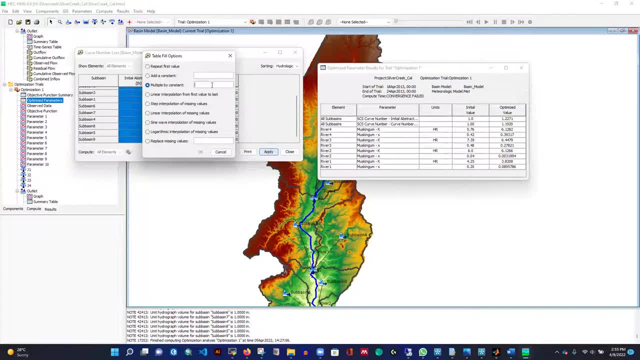 first. again, i'm doing the same thing. i'm first. again, i'm doing the same thing. i'm increasing this one, increasing this one, increasing this one. i'm multiplying this. this is okay. i'm multiplying this. this is okay. i'm multiplying this. this is okay because it has to be 0.2271. 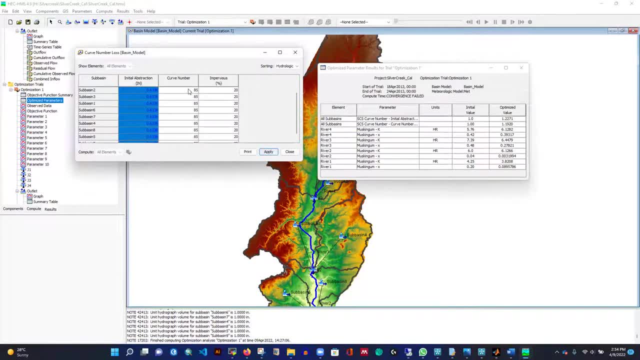 because it has to be 0.2271. because it has to be 0.2271. i'm multiplying that, so that's okay. but i'm multiplying that, so that's okay. but i'm multiplying that, so that's okay. but for curve number instead of. 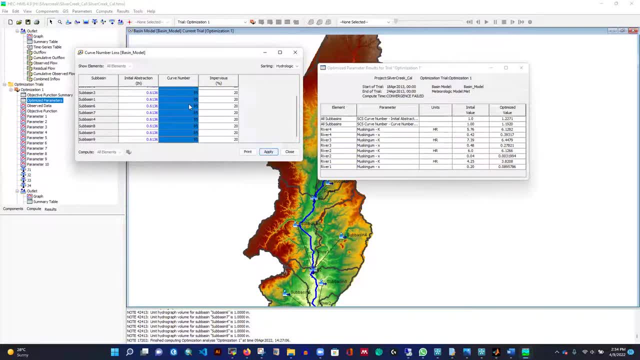 for curve number instead of for curve number. instead of doing it like more than 100, i'm just doing it like more than 100. i'm just doing it like more than 100. i'm just putting it as uh, putting it as uh, putting it as uh: nine two, okay. 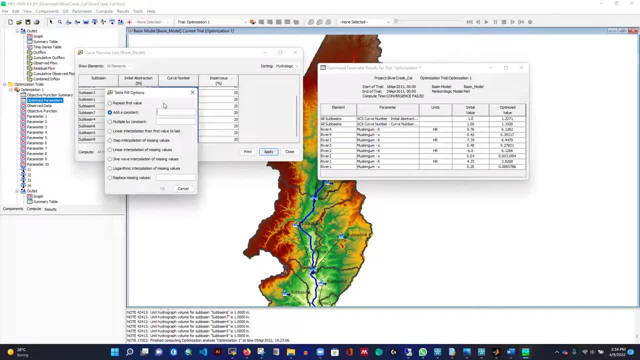 nine two, okay, nine two, okay. ninety two, ninety two, ninety two, so so, so i can add it, so i can add it, so i can add it, so i can add five, i can add seven, so i'm i can add five, i can add seven, so i'm. 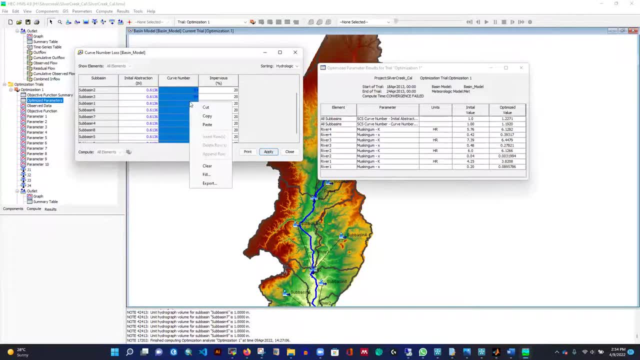 i can add five. i can add seven. so i'm adding like seven. okay, adding like seven. okay, adding like seven. okay, i'm putting it as not not okay, just minus two minus two. minus two. so it is going to be like 92 apply. so it is going to be like 92 apply. 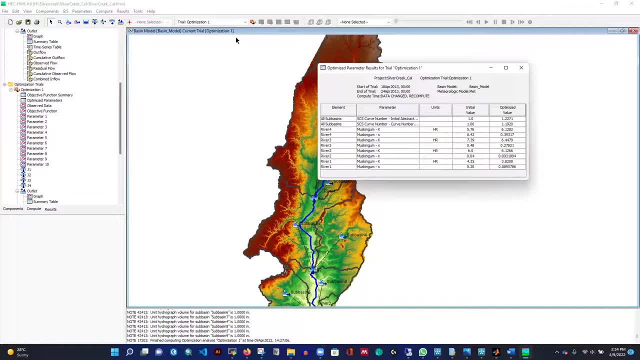 so it is going to be like 92 apply and that's okay, and that's okay and that's okay. so now, if i even so, now, if i even so, now, if i even run it now, whatever run it now, whatever run it now, whatever value we added, we have to run our main. 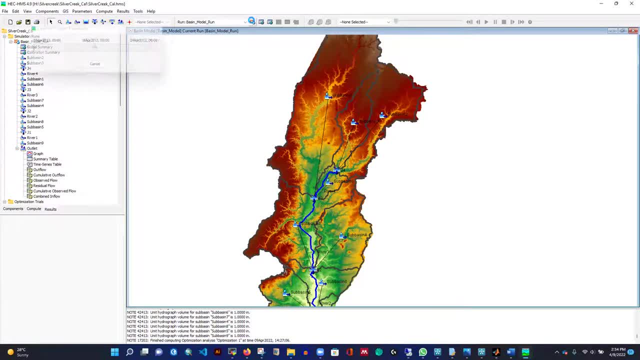 value. we added: we have to run our main value. we added: we have to run our main model, this model, this model, this simulation okay and we have to check it. simulation okay and we have to check it. simulation okay and we have to check it. if you are getting the 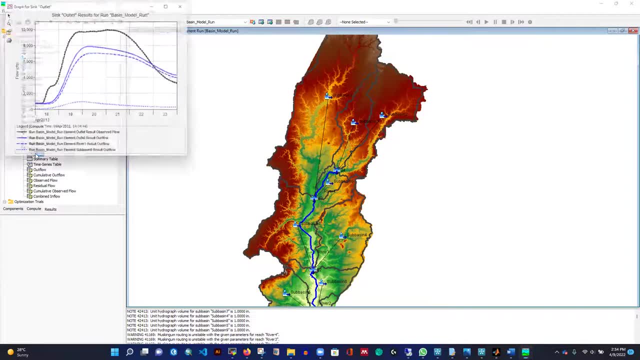 if you are getting the, if you are getting the exact, exact, exact, same shape of the hydrograph, same shape of the hydrograph, same shape of the hydrograph. see, now it's increased a little bit. see, now it's increased a little bit. see, now it's increased a little bit, but it is not. 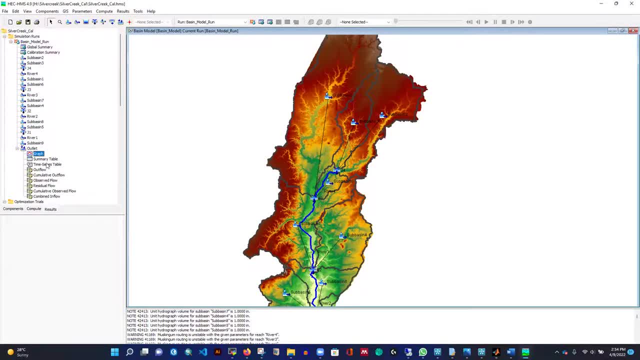 but it is not. but it is not as good as we just saw, because we didn't as good as we just saw, because we didn't as good as we just saw, because we didn't change the routing parameter as well and change the routing parameter as well, and 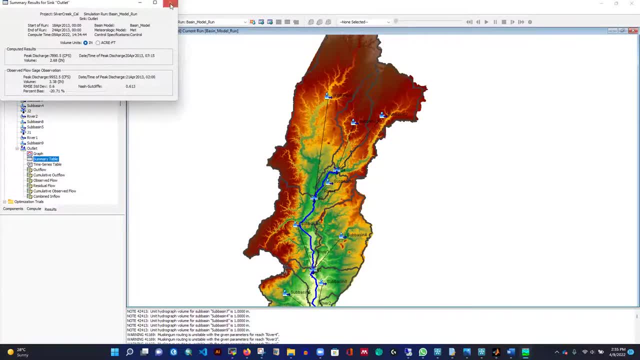 change the routing parameter as well. and let's check series even 0.61 previously. let's check series even 0.61 previously. let's check series even 0.61 previously. it was, it was, it was 0.26, but it increased. 0.26, but it increased. 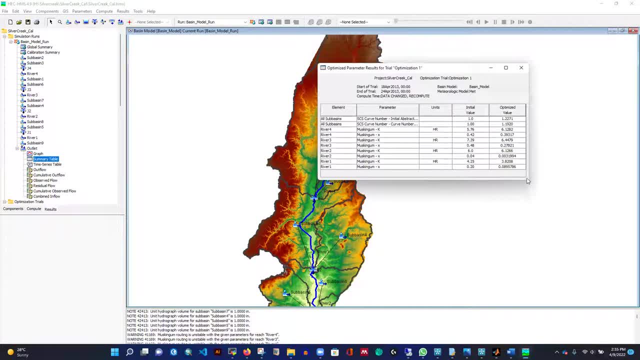 0.26, but it increased. now, what we have to do from the now, what we have to do from the now, what we have to do from the optimization: we need to change the optimization. we need to change the optimization. we need to change the routing parameter as well. 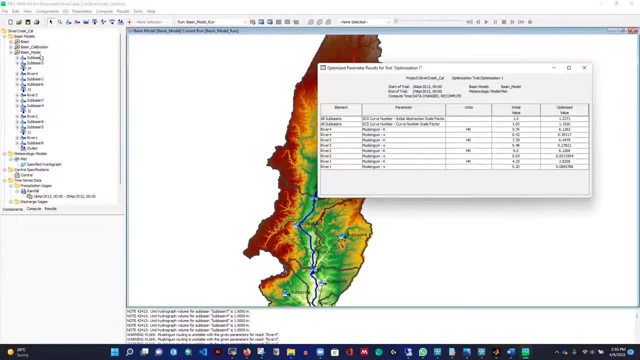 routing parameter as well, routing parameter as well. we didn't change that, we didn't change that. we didn't change that. so again, i'm gonna open. so again, i'm gonna open, so again i'm gonna open. i'm gonna open the parameter and then routing. we use the muskingum method and 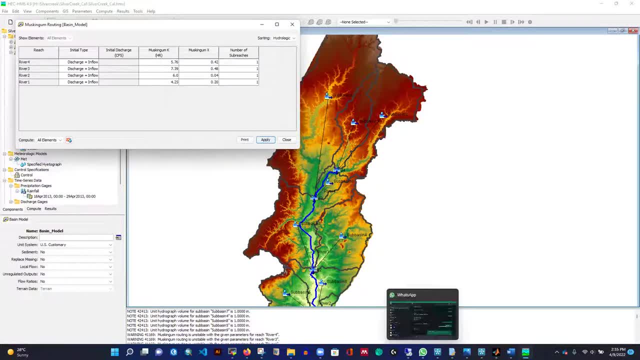 routing: we use the muskingum method. and routing: we use the muskingum method. and here we have to select, here we have to select, here we have to select this, and we can even this, and we can even this, and we can even add all this. okay, so for 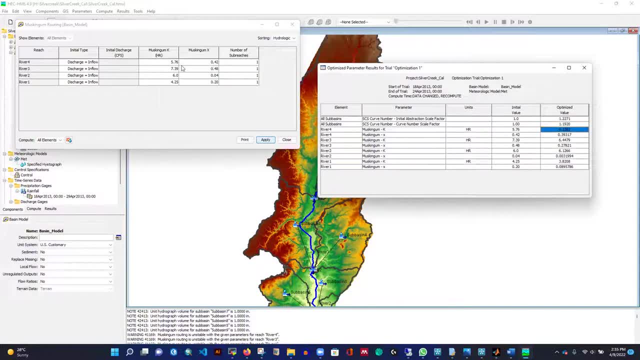 add all this. okay. so for add all this. okay. so for river 4, the x value will be this river 4, the x value will be this. river 4, the x value will be this instead of that. okay, it has to be. instead of that. okay, it has to be. 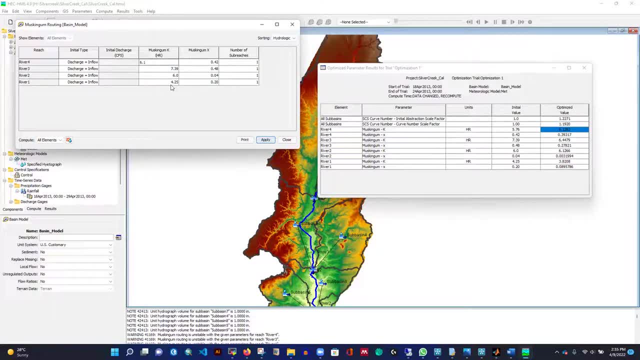 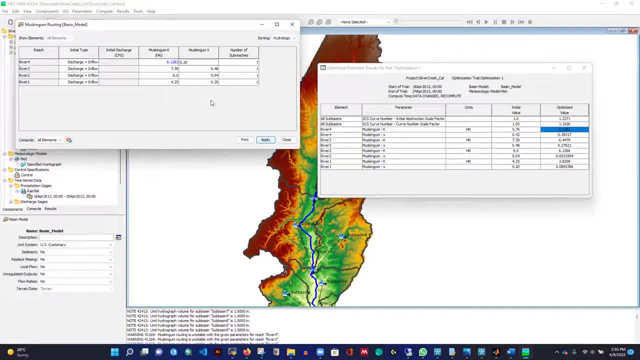 zero point three. nine instead of four. zero point three. nine instead of four. two zero point three. two. zero point three. nine. two. zero point three. nine. three, that's okay. so for river three, that's okay. so for river three, that's okay. so for river uh three, the value will be reduced okay. 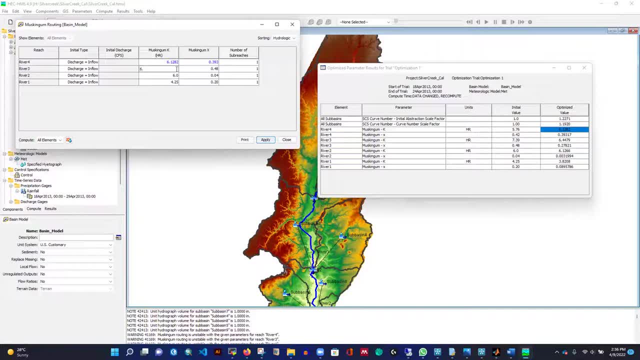 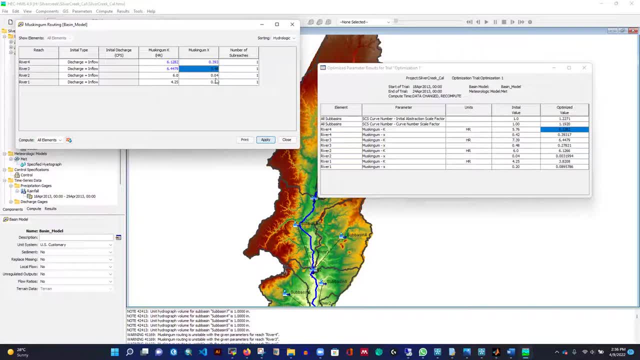 x for reach three, x for reach three. it is going to be zero point two. it is going to be zero point two. it is going to be zero point two. seven, eight, seven, eight, seven, eight. zero point two, zero point two. zero point two, seven, eight and for: 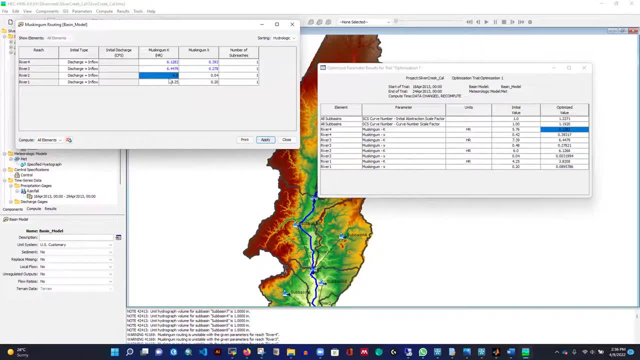 seven, eight, and for seven, eight and for reach two, the value six point one, two, reach two, the value six point one, two, reach two, the value six point one, two, it's six. so just uh, 6.12 didn't change, it's six. so just uh, 6.12 didn't change. 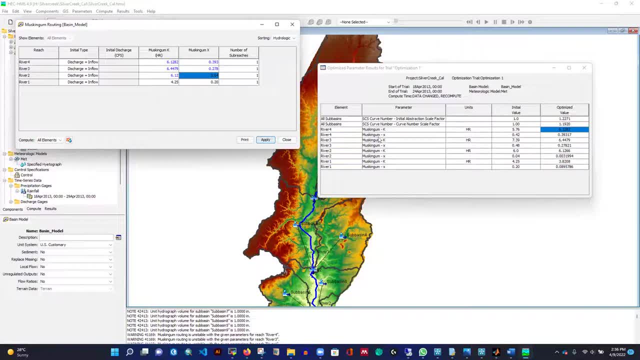 it's six, so just uh, 6.12 didn't change that much, that much, that much. and what will be the value of this and what will be the value of this and what will be the value of this parameter? nearly zero, so we can't even. 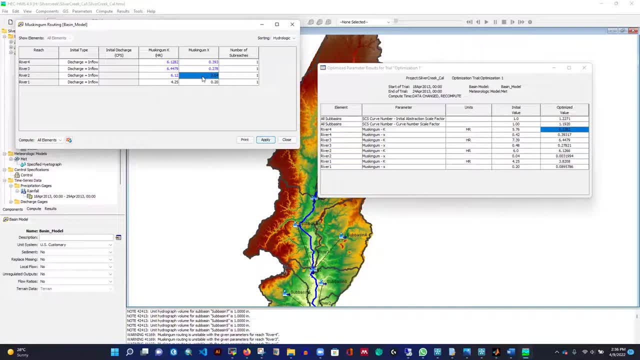 parameter nearly zero, so we can't even parameter nearly zero, so we can't even keep it. zero point, keep it zero point, keep it zero point. zero four, zero four, zero four. there is no. so whatever we are getting, there is no so whatever we are getting, there is no. so whatever we are getting from the upstream, it is just quickly. 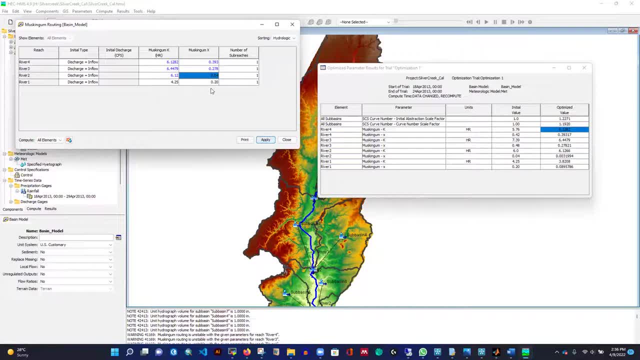 from the upstream, it is just quickly from the upstream, it is just quickly shifting the shifting, the shifting the flat without uh just flat, without uh just flat, without uh just reducing the peak or shifting the peak, reducing the peak or shifting the peak, reducing the peak or shifting the peak. so for 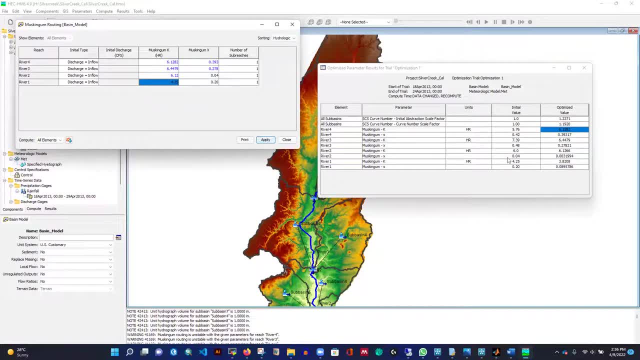 so for so, for sub river number one, the last one, we sub river number one, the last one. we sub river number one, the last one. we have 4.25, but it is going to give us. have 4.25, but it is going to give us. 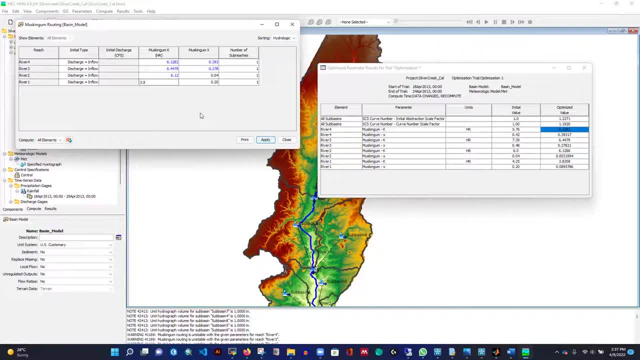 have 4.25, but it is going to give us 3.8, 3.8, 3.8, uh, 3.82, uh, 3.82, uh, 3.82, and then this value is also basically, and then this value is also basically. 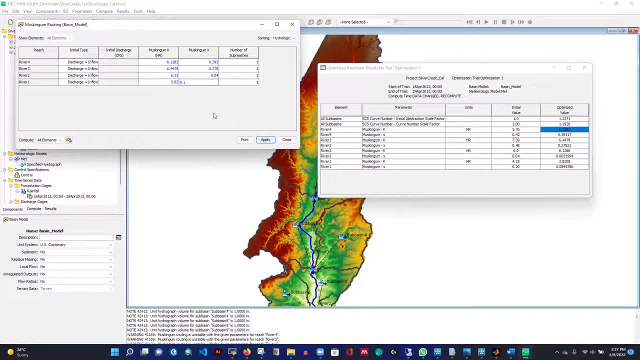 and then this value is also basically zero point, uh, zero point, uh, zero point, uh, eight. okay, we can use like zero point eight. okay, we can use like zero point eight. okay, we can use like zero point. one as well, not a problem. one as well, not a problem. 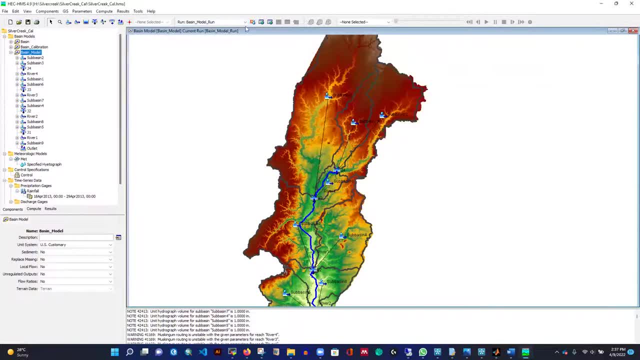 one as well, not a problem. so i'm closing these and again i'm so. i'm closing these and again i'm so, i'm closing these, and again i'm setting the model. i'm just running it. so, setting the model, i'm just running it. so. 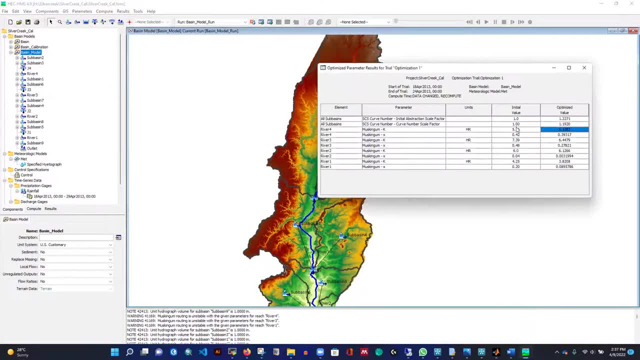 setting the model. i'm just running it, so it takes a lot of time. it takes a lot of time. it takes a lot of time and passions as well. so let's see what, and passions as well. so let's see what. and passions as well. so let's see what i have got. 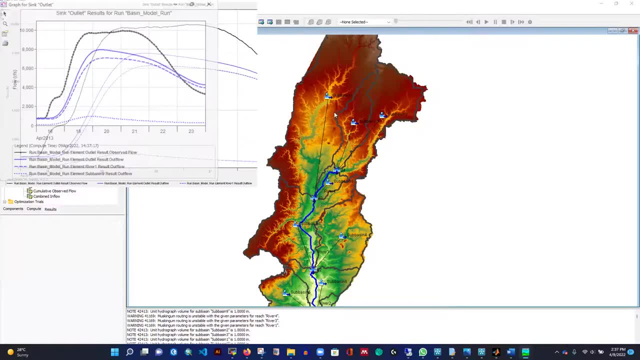 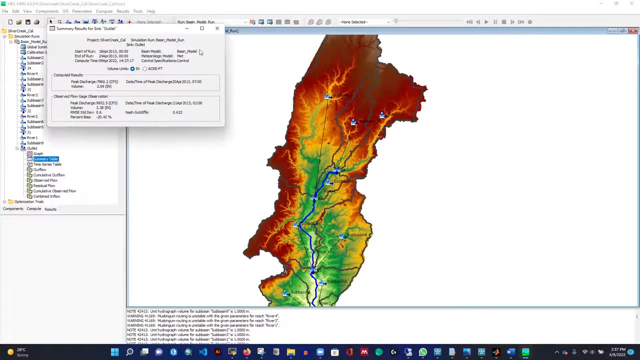 i have got, i have got from the simulation and it from the simulation and it from the simulation and it increase a little bit right, and let's increase a little bit right, and let's increase a little bit right, and let's check, check, check. the sum reset 6: 3 instead of 6: 1, so it 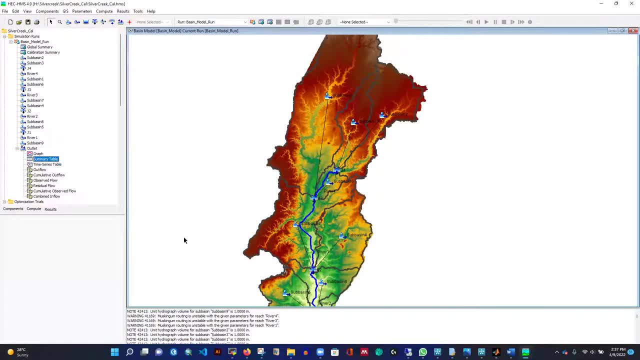 the sum reset 6: 3 instead of 6: 1. so it the sum reset 6: 3 instead of 6: 1. so it is increasing, is increasing, is increasing a bit by bit, so even we can't. a bit by bit, so even we can't. 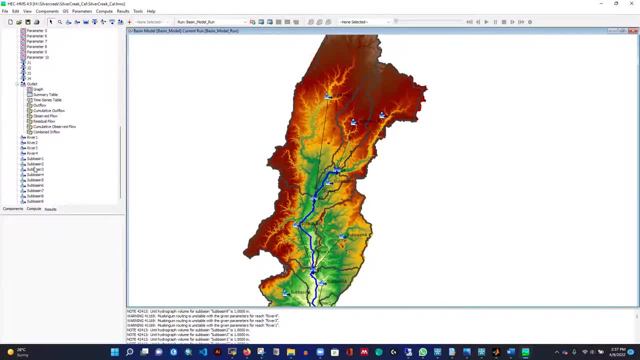 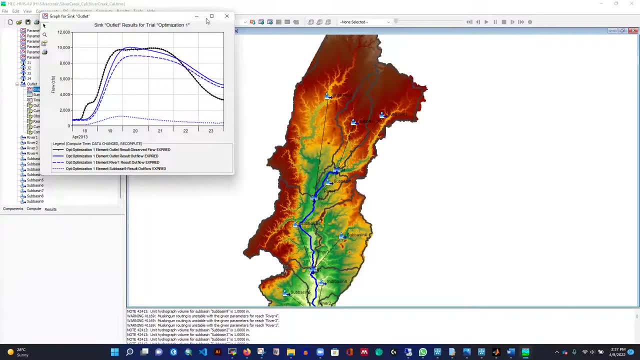 a bit by bit. so even we can't increase more because the graphic got increase more, because the graphic got increase more, because the graphic got from optimization. this is for more than 100. this is for more than 100. this is for more than 100 curve number. but that is not realistic. so 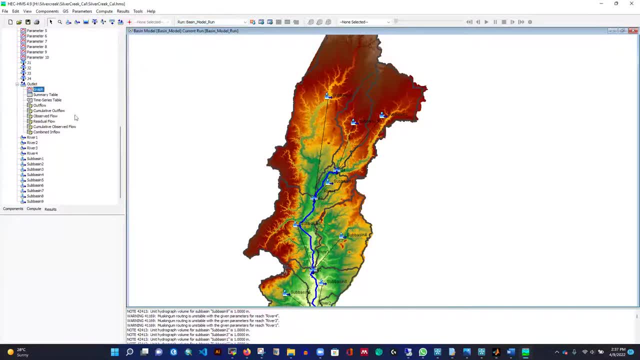 curve number, but that is not realistic. so curve number, but that is not realistic, so there's, so we're not taking that value. there's, so we're not taking that value. there's, so we're not taking that value. so whatever value we have, we have other. 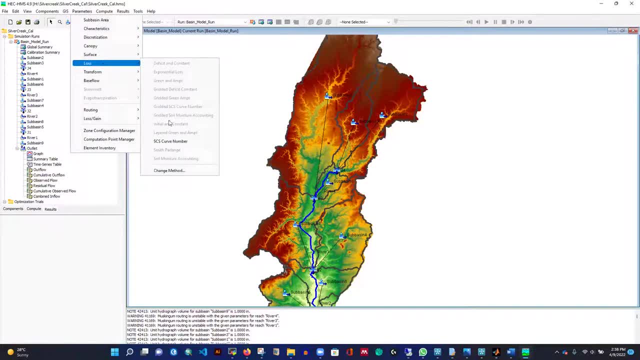 so, whatever value we have, we have other. so, whatever value we have, we have other, even, even even other calibration parameters. so we other calibration parameters, so we other calibration parameters. so we are done with our, are done with our, are done with our loss method, we're done with our. 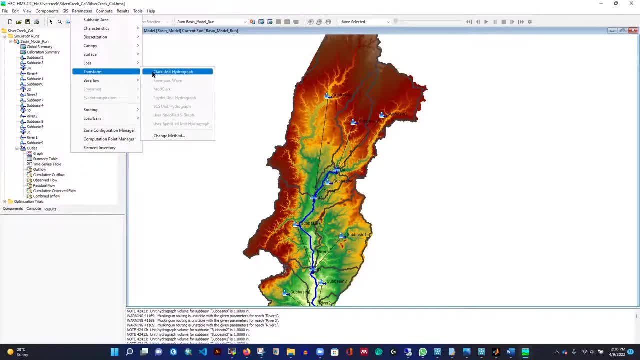 routing. so we have transform method routing, so we have transform method routing, so we have transform method: right, this one clark, right, this one clark, right, this one clark unit hydrograph. so whatever value we unit hydrograph, so whatever value we unit hydrograph, so whatever value we have here, 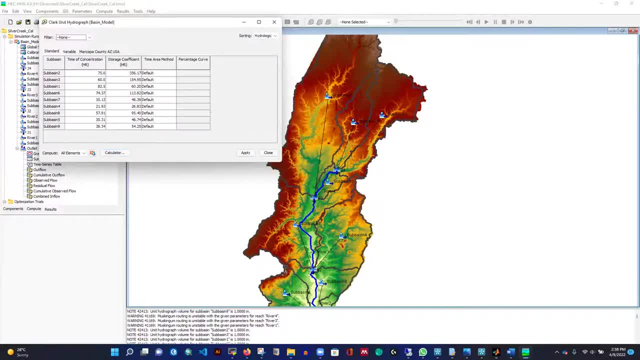 have here, have here, this value looks pretty big. that's why this value looks pretty big. that's why this value looks pretty big. that's why we have a curve, we have a curve, we have a curve, that curve, even that curve, even that curve. even giving us 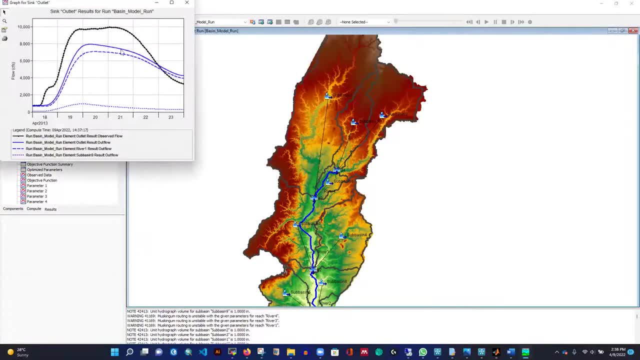 giving us, giving us a hint right that? okay, we have a hint right that. okay, we have a hint right that. okay, we have to shift the curve on the left, to shift the curve on the left, to shift the curve on the left. see, we need to shift it on the left. 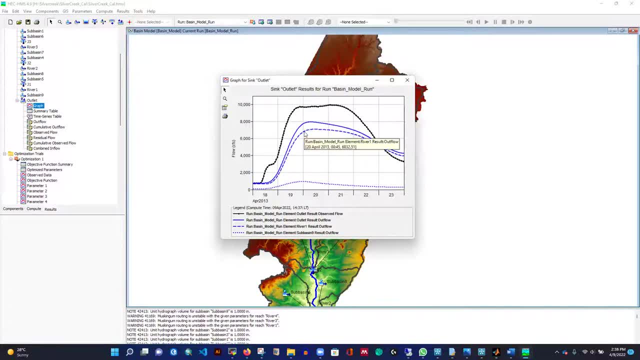 see, we need to shift it on the left. see, we need to shift it on the left side. so if your time of concentration is side, so if your time of concentration is side, so if your time of concentration is high, high, high, that means it is taking time to 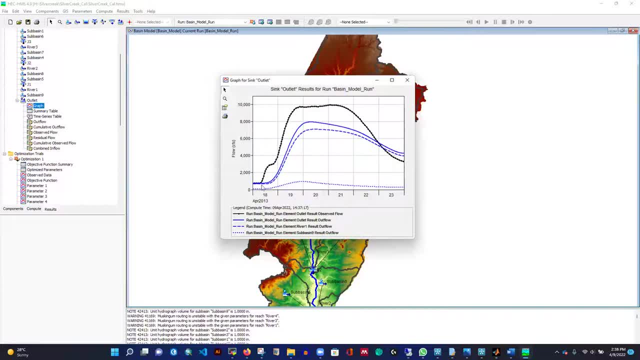 that means it is taking time to, that means it is taking time to concentrate and then flow. so that's why concentrate and then flow. so that's why concentrate and then flow. so that's why the flow, the flow, the flow is starting at a, is starting at a. 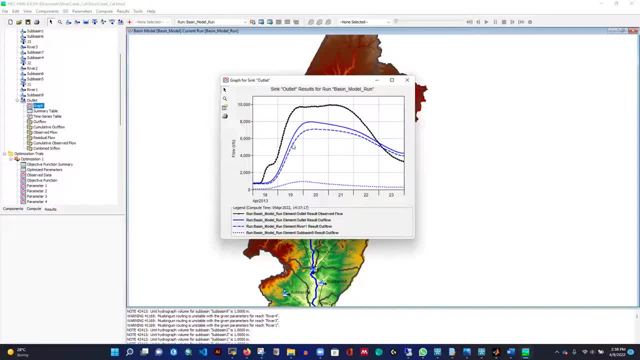 is starting at a delayed, the flow is being delayed, delayed, the flow is being delayed, delayed. the flow is being delayed. so it has to be so, it has to be, so it has to be fast. so we have to reduce the time of fast, so we have to reduce the time of. 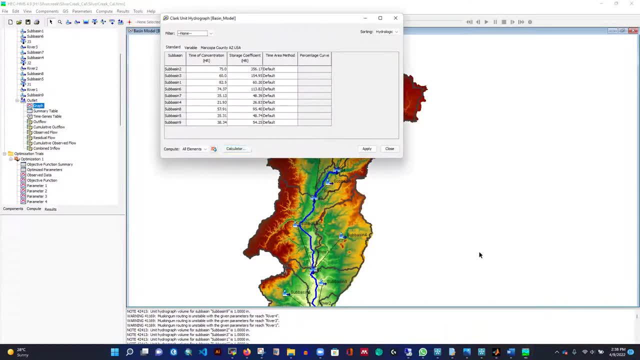 fast. so we have to reduce the time of concentration, concentration, concentration. if you want to reduce the time of, if you want to reduce the time of, if you want to reduce the time of concentration, concentration, concentration. what we have to do so for all of this. what we have to do so for all of this. 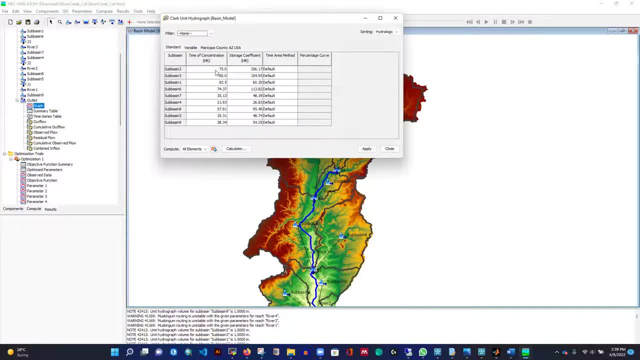 what we have to do. so, for all of this, what i can do, what i can do, what i can do, i can even reduce this value by what will be the value i can reduce, we, what will be the value i can reduce, we, what will be the value i can reduce? we have this, so i can even multiply a. 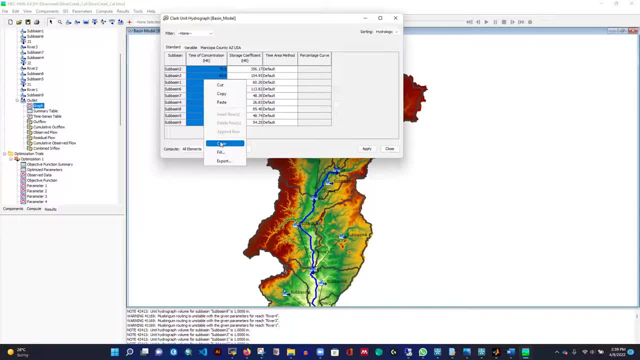 have this, so i can even multiply a. have this, so i can even multiply a factor. that's what i do factor. that's what i do factor. that's what i do, instead of doing this, what i do, i just. instead of doing this, what i do, i just 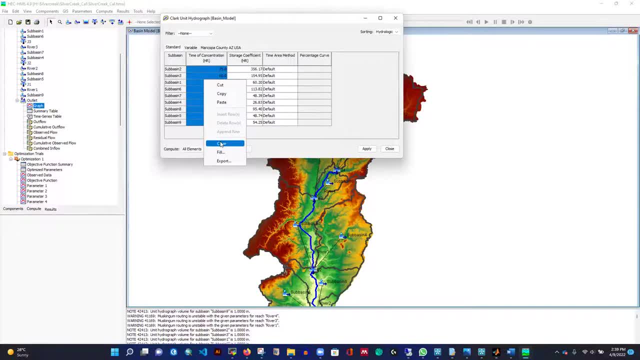 instead of doing this, what i do i just multiply, multiply, multiply. or i divide by this one or that one, or i divide by this one or that one, or i divide by this one or that one. so, instead of doing that, so, instead of doing that, so, instead of doing that, i can. 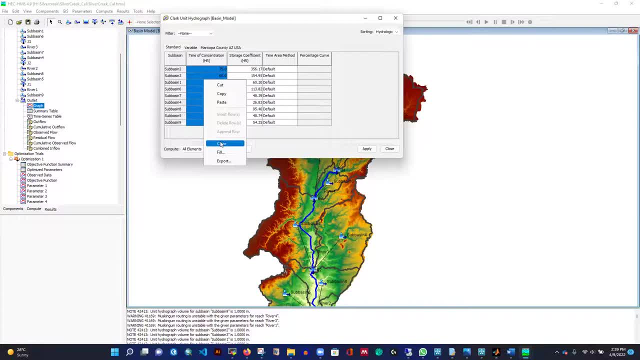 70, 70, or i can even reduce uh 50, 70, 70, or i can even reduce uh 50, 70, 70, or i can even reduce uh 50, right, so i can multiply this value. so i can multiply this value, so i can multiply this value. let's see: 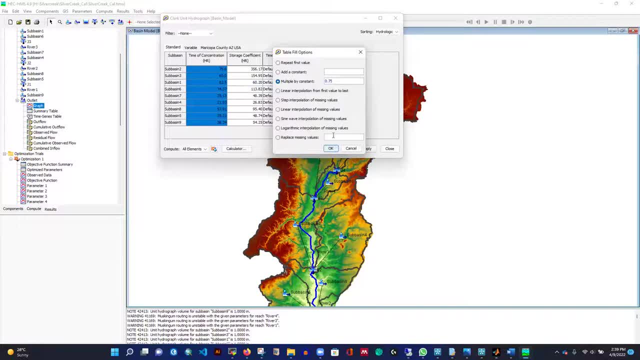 let's see. let's see, by a constant like 0.75, by a constant like 0.75, by a constant like 0.75- okay, i'm multiplying this. okay, i'm multiplying this, okay, i'm multiplying this. so we are getting this and apply, and 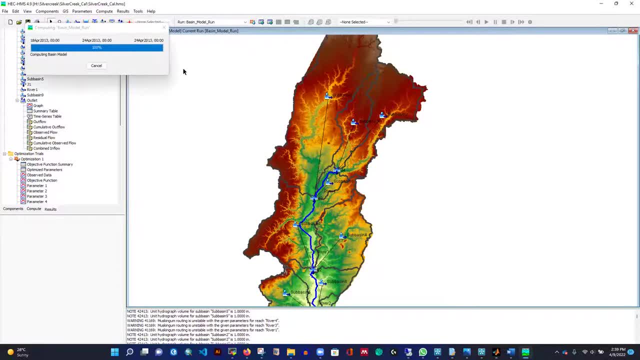 so we are getting this and apply. and so we are getting this and apply and let's see if we can get any increased. let's see if we can get any increased, let's see if we can get any increased or improved or improved or improved shape and going to result, and check. 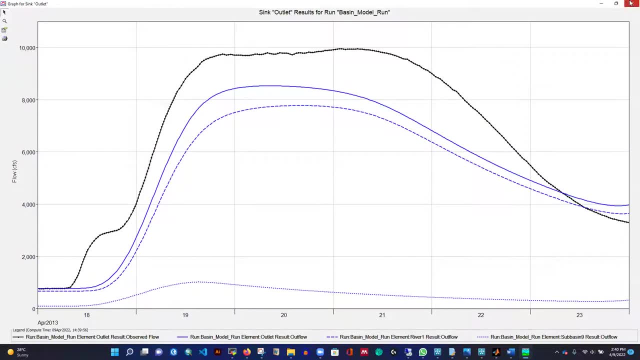 shape and going to result and check. shape and going to result and check. yeah, it is maybe shifting on the left. yeah, it is maybe shifting on the left. yeah, it is maybe shifting on the left side, a little bit side, a little bit side, a little bit. but at the same time we have to even 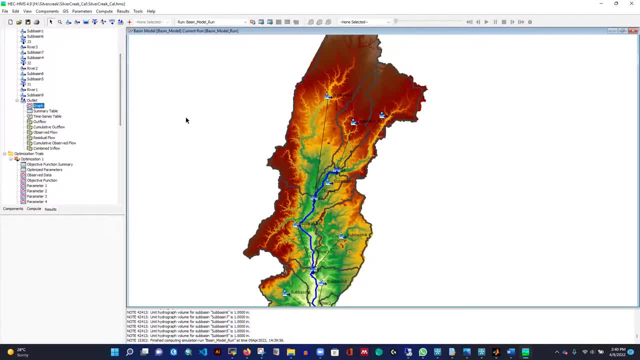 but at the same time we have to even. but at the same time we have to even reduce the losses as well, reduce the losses as well, reduce the losses as well. so we'll do that, just capture. so we'll do that, just capture. so we'll do that, just capture the shape first and check. see it's. 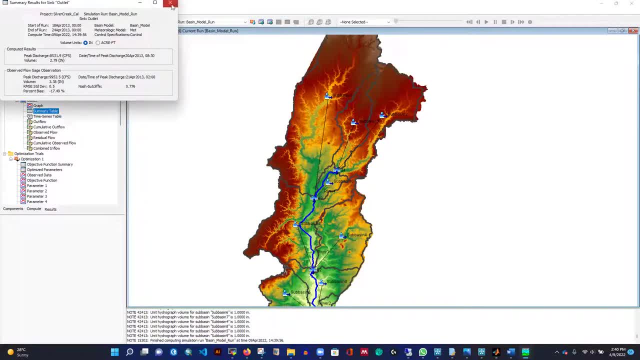 the shape first and check, see it's the shape first and check, see it's increased 0.776, increased 0.776, increased 0.776. so from 0.26 to this one, so from 0.26 to this one, so from 0.26 to this one, so it's working. 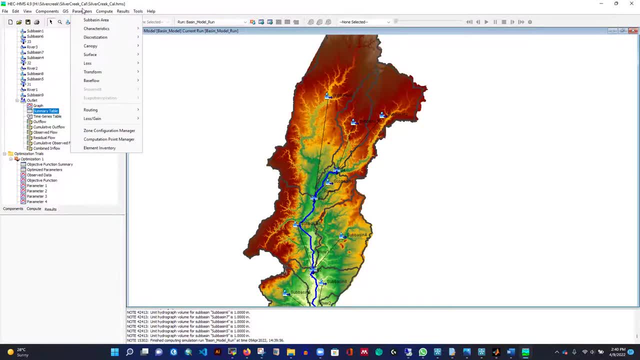 so it's working. so it's working. and one thing we have even there and one thing we have even there, and one thing we have even there: storage right. so we are there transform storage right. so we are there transform storage right. so we are there transform. so, if you want to even, 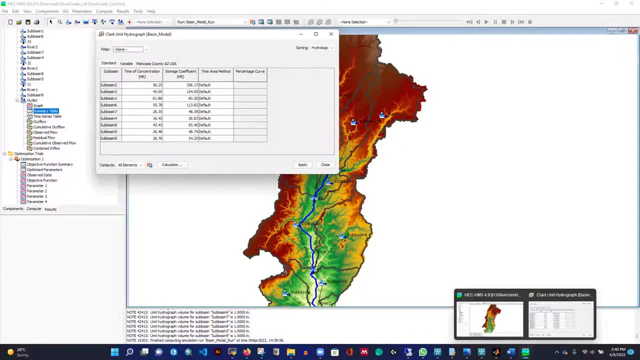 so, if you want to, even so, if you want to even capture the shape you have to play with, capture the shape you have to play with, capture the shape, you have to play with this. this, this transform method. so here, transform method. so here, transform method. so here, instead of doing this, uh, a big value. 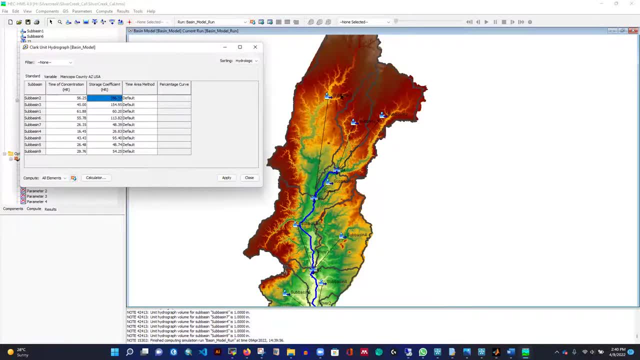 instead of doing this: uh, a big value. instead of doing this, uh, a big value. because these sub bases number two, because these sub bases number two, because these sub bases number two and three. these are basically these sub and three. these are basically these sub and three. these are basically these sub bases. you can see. 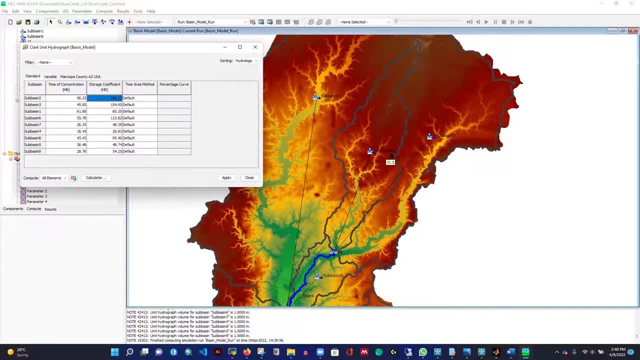 bases. you can see bases. you can see. these are the most office stream one. these are the most office stream one. these are the most office stream one, two and three. so we can play with all two and three. so we can play with all two and three. so we can play with all this thing. 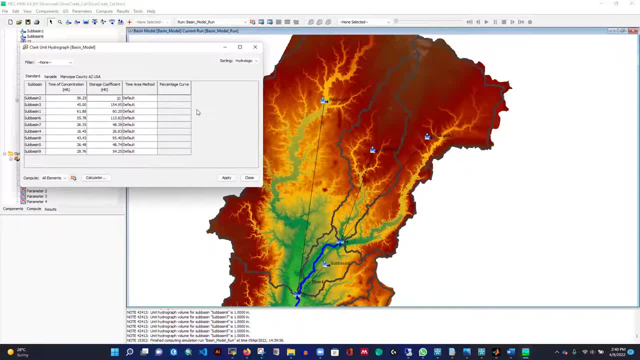 this thing, this thing. so, for this one, i'm gonna reduce it to. so, for this one, i'm gonna reduce it to. so, for this one, i'm gonna reduce it to 200, and similarly. okay, let's run 200. and similarly okay, let's run 200. and similarly okay, let's run first with this one, one by one, because 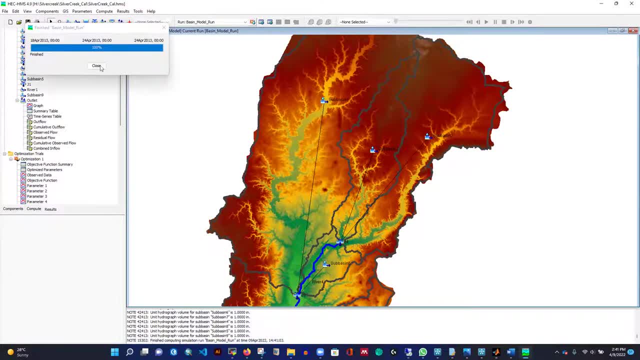 first with this one one by one, because first with this one one by one, because this is the manual calibration we're, this is the manual calibration we're, this is the manual calibration we're talking about, talking about talking about so close and let's check, yeah it. 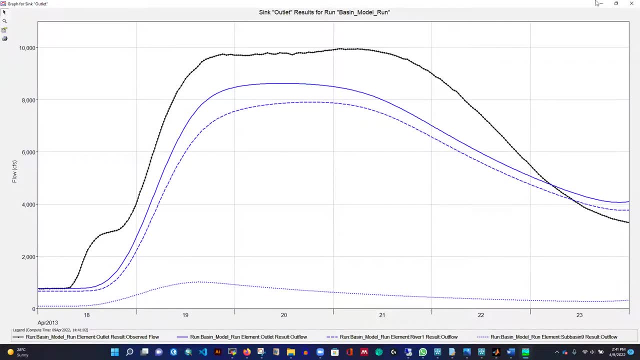 so close and let's check. yeah, it so close and let's check. yeah, it increased. see the difference increased. see the difference increased. see the difference reduce and it increased a little bit. reduce and it increased a little bit. reduce and it increased a little bit and we can check. 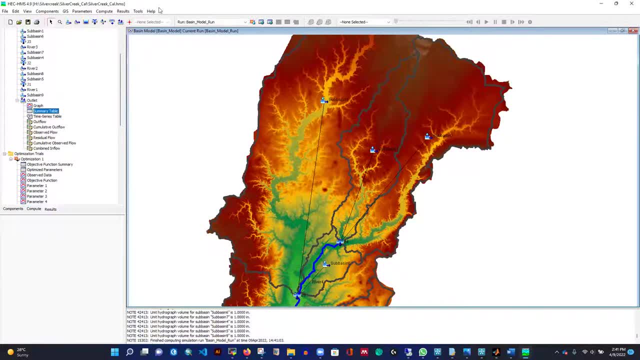 and we can check. and we can check c 0.80 right it increasing means it's. and we can check c 0.80: right it increasing means it's. and we can check c 0.80 right it increasing means it's improving, improving. 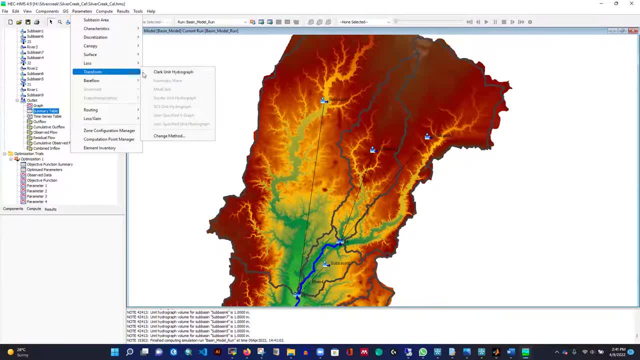 improving. so we have other parameter as well. let's, so we have other parameter as well. let's, so we have other parameter as well. let's transform method clark. we can even transform method clark. we can even transform method clark. we can even change this. 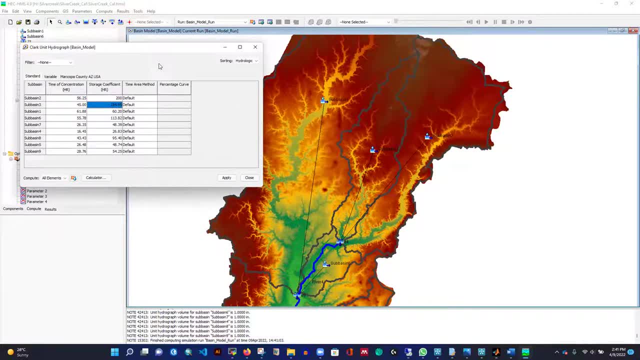 change this. change this can reduce this, because, if you want to, can reduce this, because, if you want to, can reduce this, because if you want to increase the volume, you have to increase the volume. you have to increase the volume, you have to reduce the storage coefficient. okay, so. 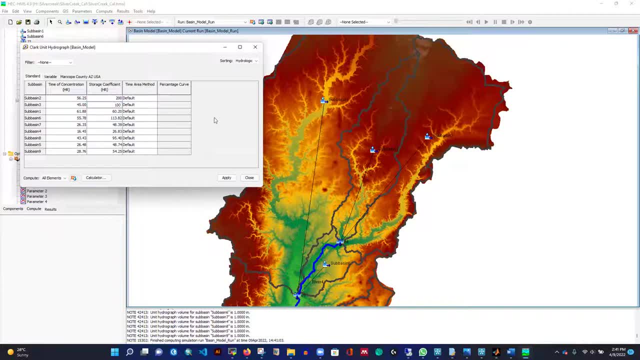 reduce the storage coefficient- okay. so reduce the storage coefficient, okay. so that will be okay. 100, that will be okay. 100, that will be okay. 100, let's see, let's see, let's see 100 and let's run it. so this is how we have to even fix that. 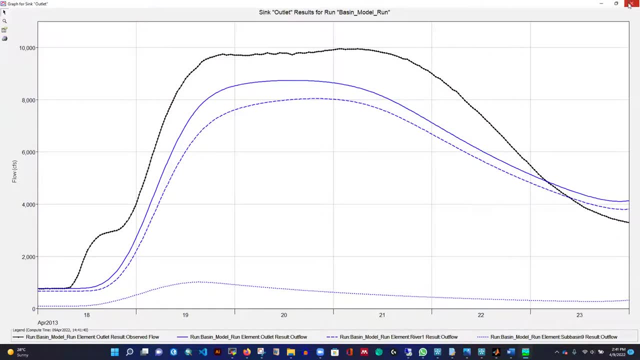 so this is how we have to even fix that, so this is how we have to even fix that: manual, manual, manual and automatic, even and automatic, even and automatic, even. we can't see the difference. maybe little. we can't see the difference, maybe little. we can't see the difference, maybe little difference we can check. 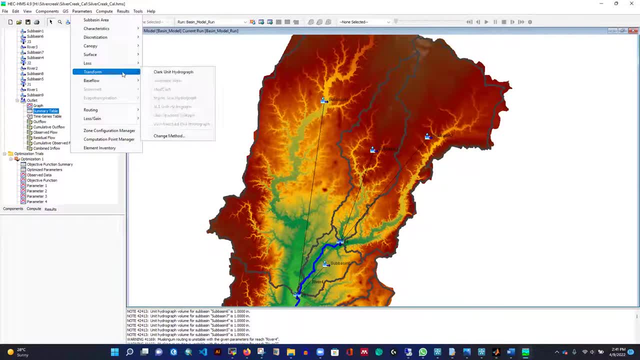 difference. we can check difference. we can check 82, 82, 82 and i can even, and i can even, and i can even transform method. okay, i can reduce it to transform method. okay, i can reduce it to transform method. okay, i can reduce it to 90. 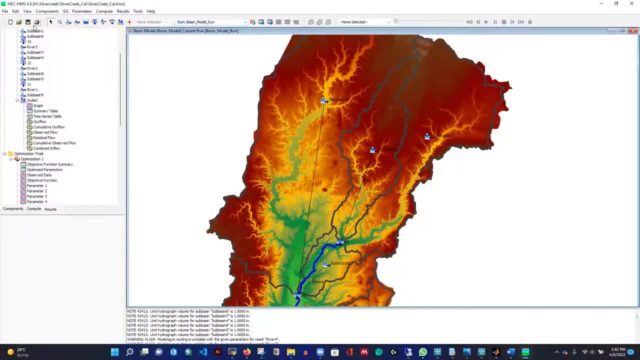 90, 90, and then i won't do that anymore, because, and then i won't do that anymore, because, and then i won't do that anymore because i, i, i don't see any change, don't see any change, don't see any change, let's run it. 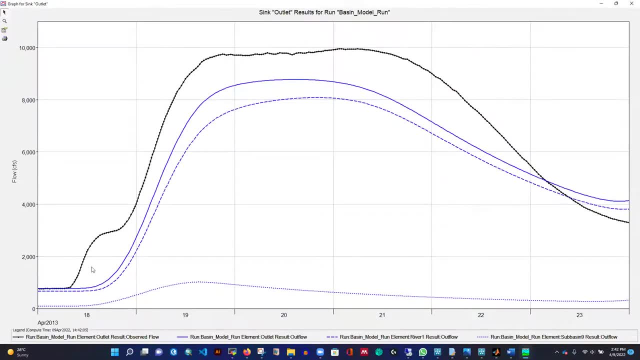 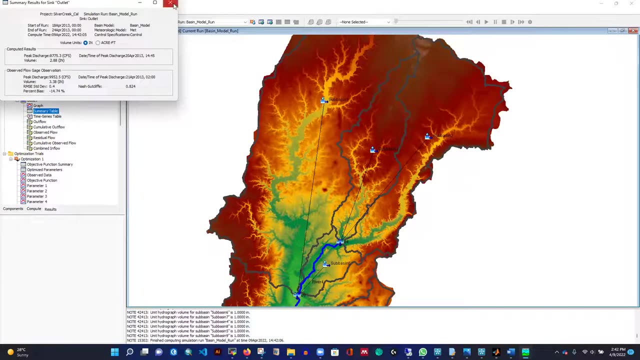 and check the graph if it improved or not. and check the graph if it improved or not. and check the graph if it improved or not. yeah, it improved a little bit. yeah, it improved a little bit. yeah, it improved a little bit and we can check that value 82. 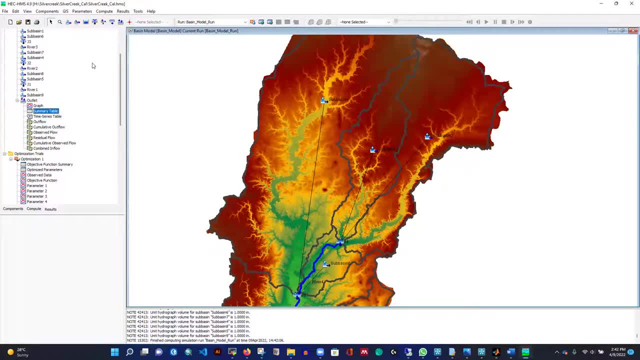 and we can check that value 82, and we can check that value 82. okay, okay, okay, so that's it. so we, whatever value we are, so that's it. so we, whatever value we are, so that's it. so we, whatever value we are changing, changing. 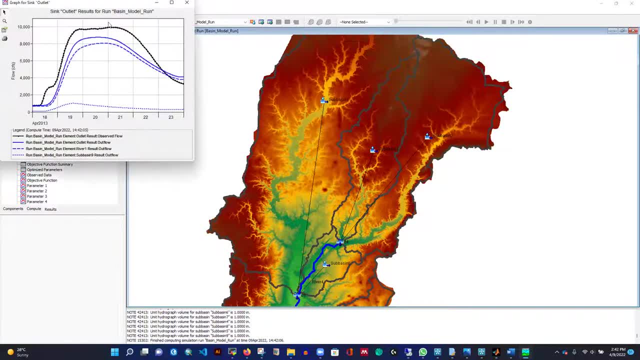 changing. now we have to reduce the loss, right, we. now we have to reduce the loss. right, we, now we have to reduce the loss. right, we can see that. okay, can see that. okay, can see that. okay, still, our model is underestimating the. still our model is underestimating the. 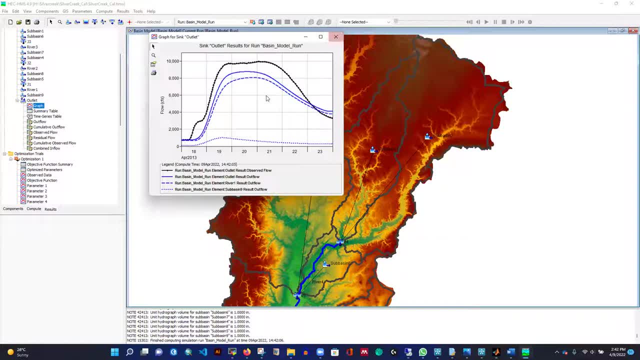 still, our model is underestimating the stream flow we have. we have to stream flow we have. we have to stream flow we have. we have to even reduce the loss so that we can even reduce the loss, so that we can even reduce the loss, so that we can even uh. 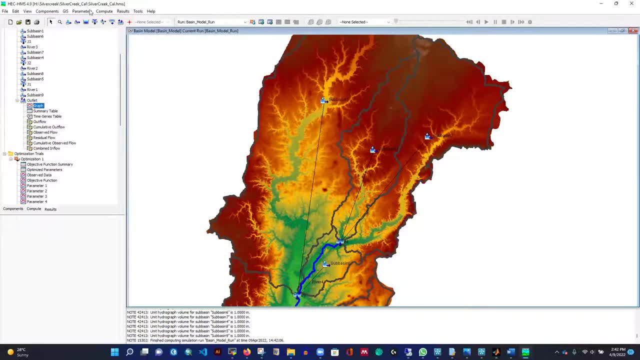 even, uh, even, uh, diminish the gap between these two, diminish the gap between these two, diminish the gap between these two. so we have only three things like so. we have only three things like. so we have only three things like loss, loss, loss, transform, transform, transform and then the routing. so 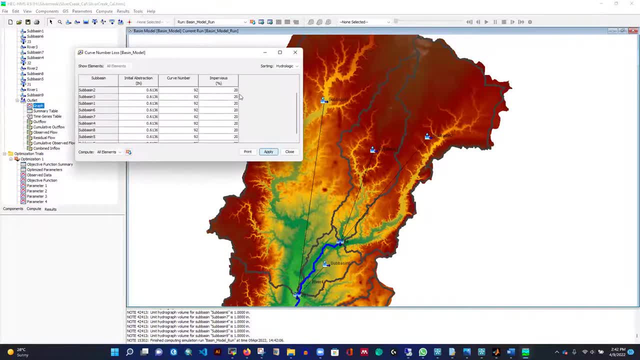 and then the routing. so and then the routing. so let's play with the loss. we have to. let's play with the loss. we have to. let's play with the loss. we have to reduce the loss, reduce the loss, reduce the loss. we're going to reduce the losses and 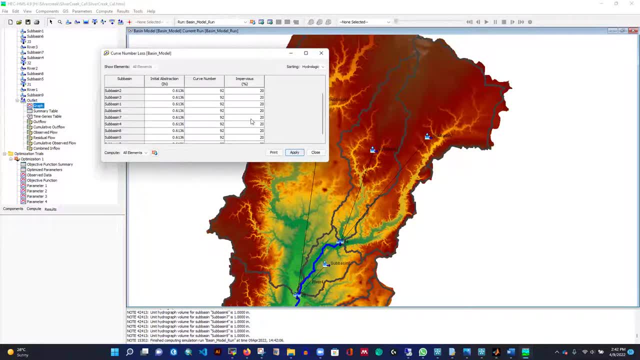 we're going to reduce the losses and we're going to reduce the losses, and then what we can do then, what we can do, then what we can do, okay. so, instead of using 30, okay. so, instead of using 30, okay. so, instead of using 30, we can even at 20, we can use 30, okay. 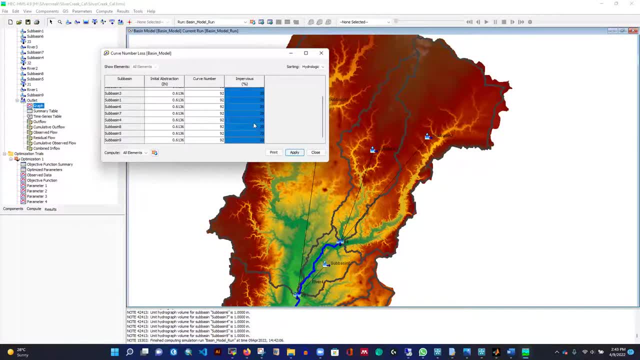 we can even at 20, we can use 30. okay, we can even at 20, we can use 30. okay, we can use 30. you can select. we can use 30. you can select, we can use 30. you can select. right click, uh fill. 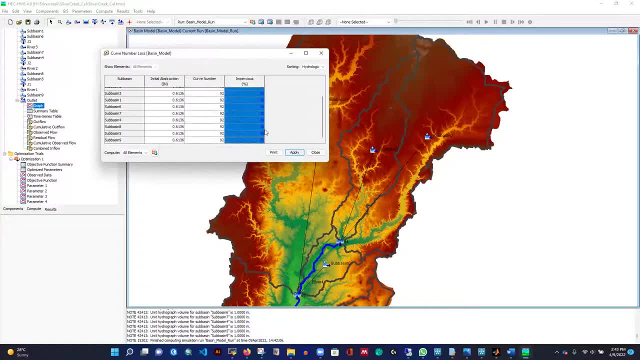 right click, uh fill, right click, uh fill, add constant. so we are going to add 10, add constant. so we are going to add 10, add constant. so we are going to add 10 percent to all, percent to all, percent to all, and apply and see, because we're 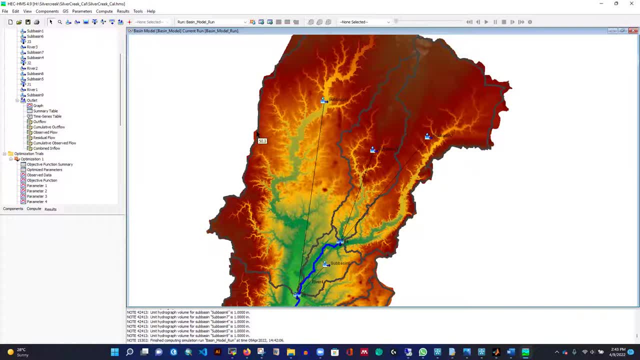 and apply, and see because we're and apply, and see, because we're increasing the percentage, increasing the percentage, increasing the percentage. imperviousness so that imperviousness, so that imperviousness, so that there will be less loss, there will be less loss. 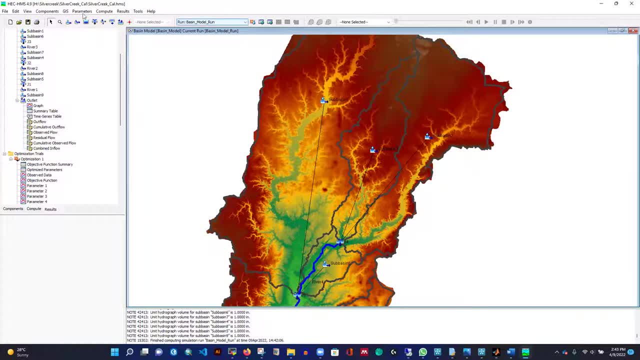 there will be less loss, right? so it will even increase the flow, right? so it will even increase the flow, right so it will even increase the flow. and we can even run it. set the model and we can even run it. set the model and we can even run it. set the model and run it. 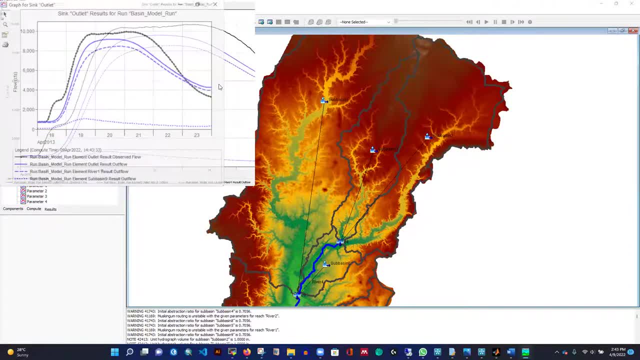 and run it and run it okay. so let's see if we get anything. okay, okay, so let's see if we get anything. okay, okay, so let's see if we get anything. okay, yeah, it improved. see, yeah, it improved. see, yeah, it improved. see, reduce the gap. that is pretty good. 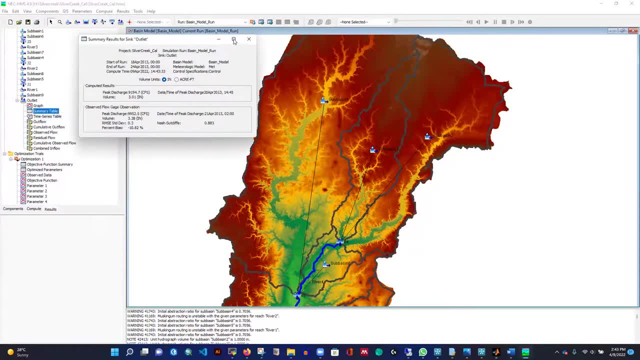 reduce the gap, that is pretty good. reduce the gap: that is pretty good. so, from the summary table: see 88. it's so. from the summary table: see 88. it's so. from the summary table: see 88. it's really good. right, we already got 88. 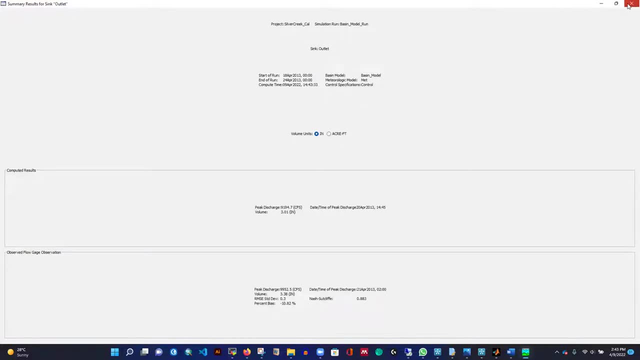 really good, right, we already got 88. really good, right, we already got 88 without capturing the, without capturing the, without capturing the shape. 0.88 nse- nse. 0.88 means it's really shape. 0.88 nse- nse. 0.88 means it's really. 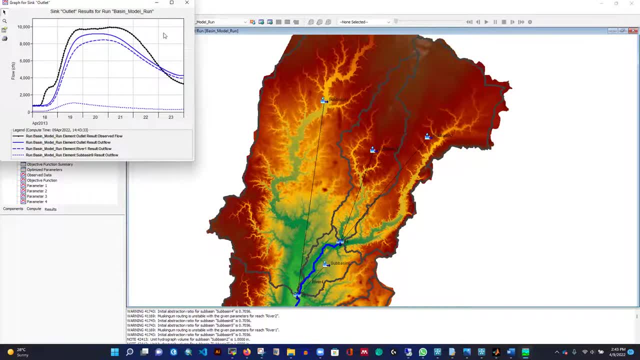 shape: 0.88, nse, nse. 0.88 means it's really good, good, good. so we have a very good shape, so we have a very good shape, so we have a very good shape. i can even show you that one as well. i can even show you that one as well. 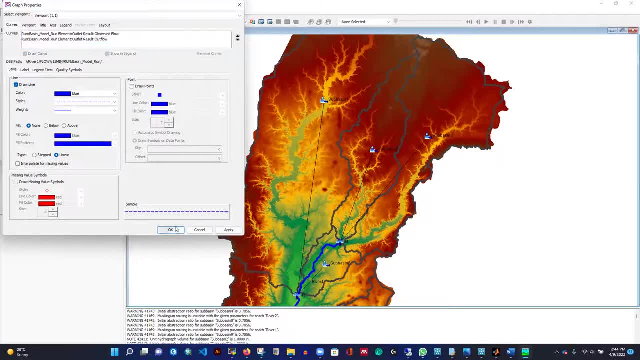 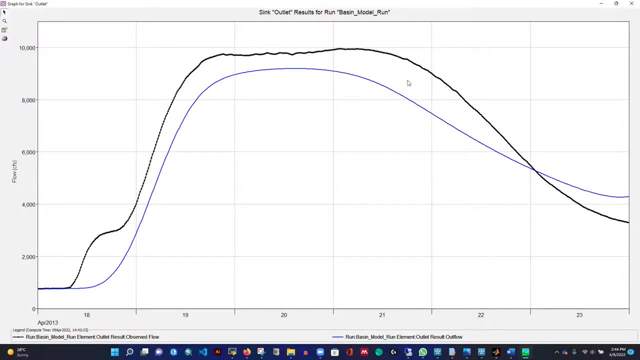 i can even show you that one as well. after removing this, after removing this, after removing this element: okay, so that's that element, okay, so that's that element, okay, so that's that. see, the shape is really good, right. see, the shape is really good, right? see, the shape is really good, right? yeah, shape is really good. only one thing: 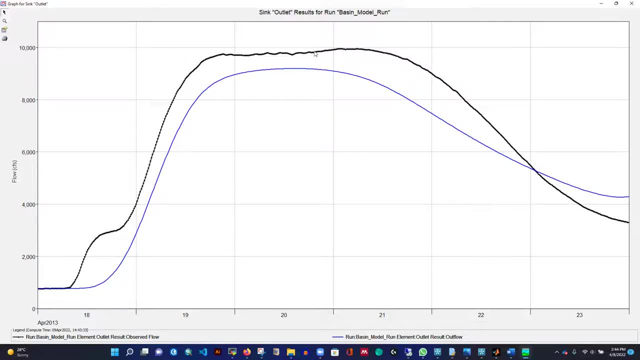 yeah, shape is really good. only one thing: yeah, shape is really good. only one thing we need to do. we need to do, we need to do: okay, at first, we need to reduce the gap. okay, at first, we need to reduce the gap. okay, at first, we need to reduce the gap, this gap. so the loss should be. 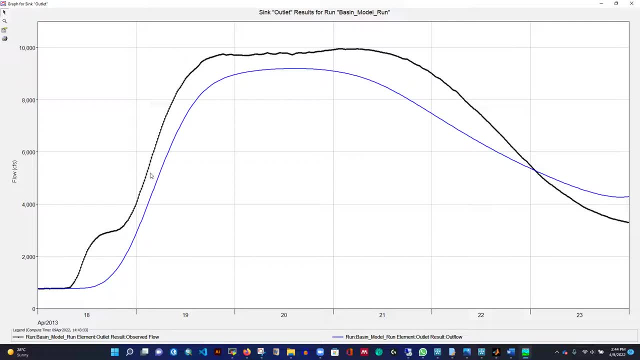 this gap, so the loss should be this gap, so the loss should be less then we can capture. we can even less, then we can capture. we can even less, then we can capture. we can even reduce this gap in between these two, reduce this gap in between these two. 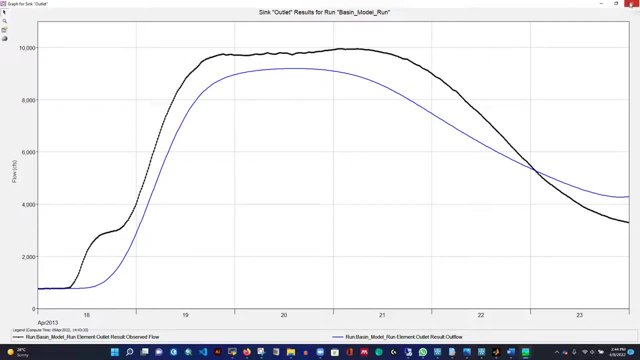 reduce this gap in between these two. that's okay, it's yeah. so in terms of that's okay, it's yeah. so in terms of that's okay, it's yeah. so in terms of volumetric comparison, volumetric comparison, volumetric comparison- the model is performing pretty good. 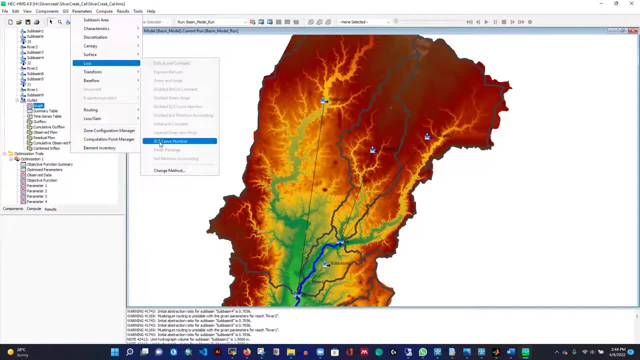 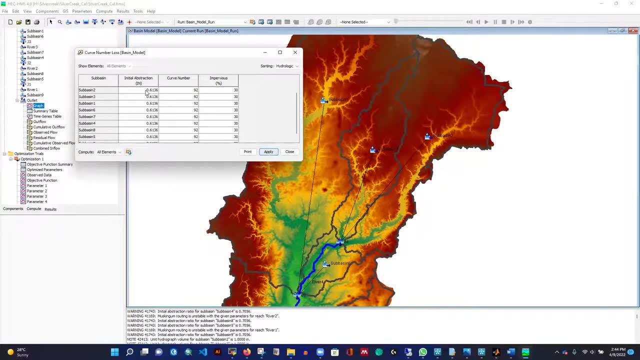 the model is performing pretty good. the model is performing pretty good, so what else we can do? you can go to. so what else we can do? you can go to. so what else we can do? you can go to parameter parameter parameter initial abstraction, like from 0.61 to. 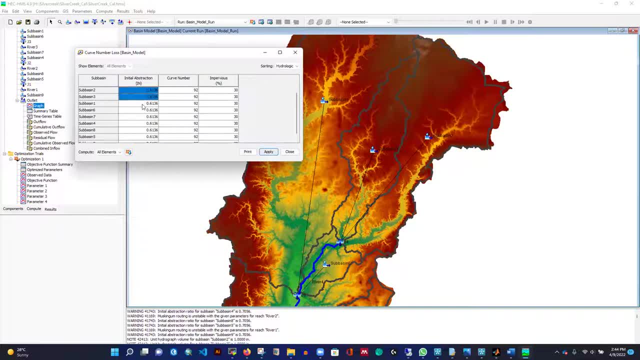 initial abstraction, like from 0.61 to initial abstraction, like from 0.61 to okay, okay, okay, 0.6, or okay, i can even reduce it 0.6, or okay, i can even reduce it 0.6, or okay, i can even reduce it from this one. so 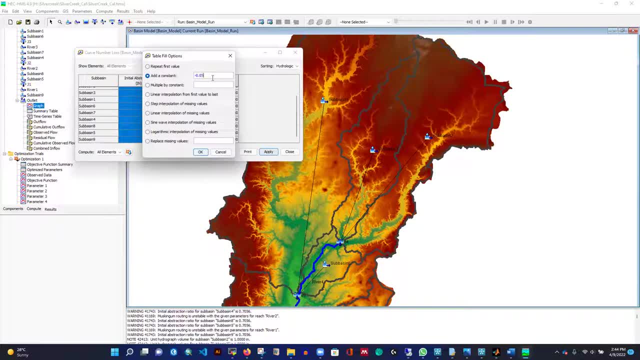 from this one, so from this one. so minus 0.05, minus 0.05. minus 0.05. how about that? let's see so 0.56. that's how about that. let's see so 0.56. that's how about that. let's see so 0.56. that's okay. 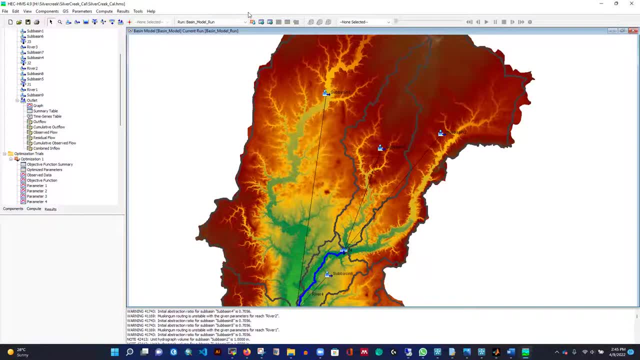 okay, okay, we can even run with that one. because we can even run with that one, because we can even run with that one, because initial abstraction is less. initial abstraction is less, initial abstraction is less. there will be less abstraction, so more. there will be less abstraction, so more. 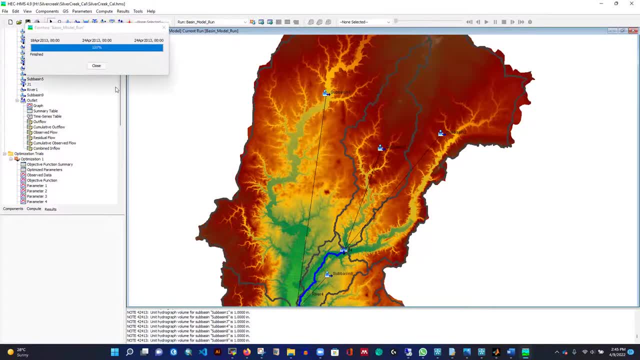 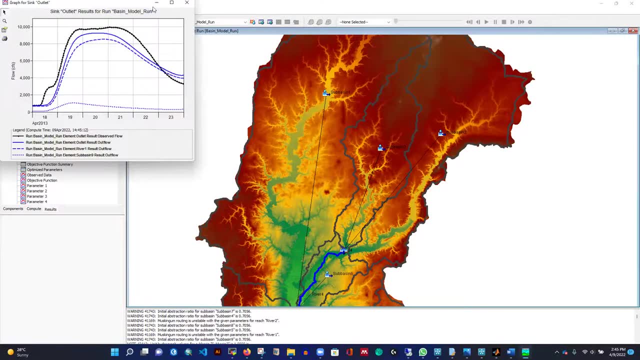 there will be less abstraction. so, more runoff, we can increase the gap between runoff. we can increase the gap between runoff. we can increase the gap between these two, these two, these two. there will be lower loss. maybe there will be lower loss, maybe there will be lower loss. maybe we can get more closer. 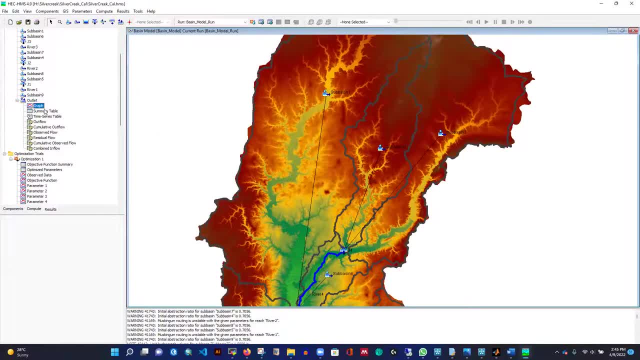 we can get more closer. we can get more closer, okay, yeah it even close to that one. so okay, yeah it even close to that one. so okay, yeah it even close to that one. so you can see 89, that means it is. you can see 89, that means it is. 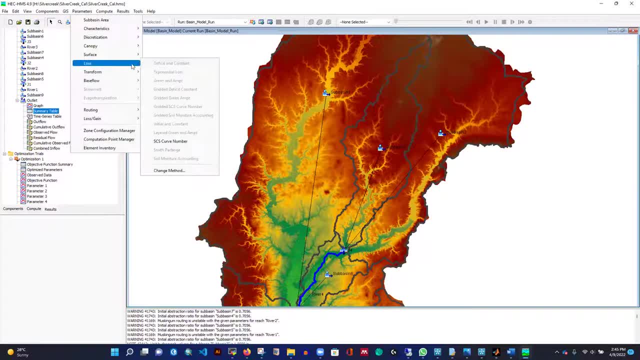 you can see 89, that means it is increasing, increasing, increasing the performance. okay, so we can play the performance. okay, so we can play the performance. okay, so we can play with that parameter, with that parameter, with that parameter, we can even uh play with this one. we can even uh play with this one. 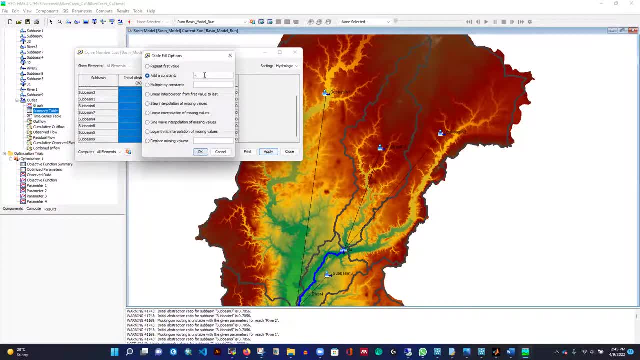 we can even uh, play with this one first. we can even reduce that minus 0.0. we can even reduce that minus 0.0. we can even reduce that minus 0.0. okay, then 0.02. okay, then 0.02. 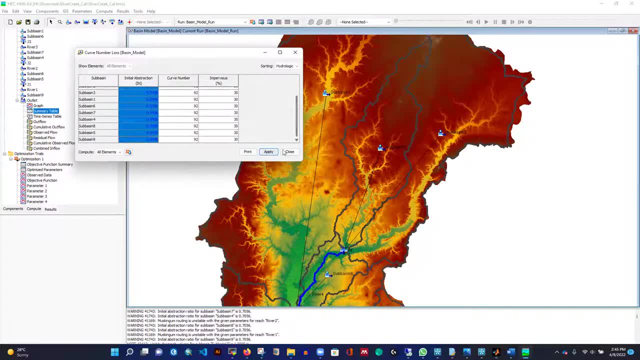 okay, then, 0.02, let's play with that. and then we'll even let's play with that, and then we'll even let's play with that, and then we'll even play with uh, play with uh, play with uh, individual sub-basin. okay, if it won't. 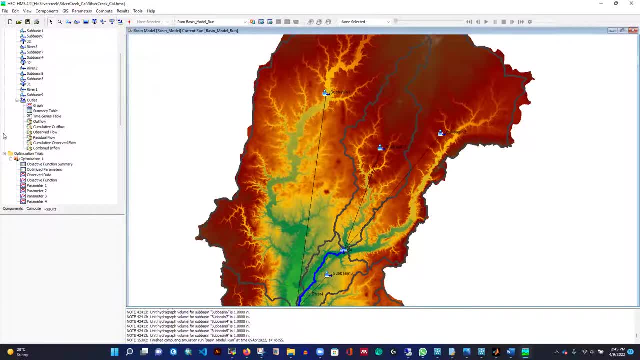 individual sub-basin, okay. if it won't, individual sub-basin, okay. if it won't work, work, work, let's see. let's see, let's see close and check that, yeah, close and check that, yeah, close and check that, yeah, or what will happen, or what will happen. 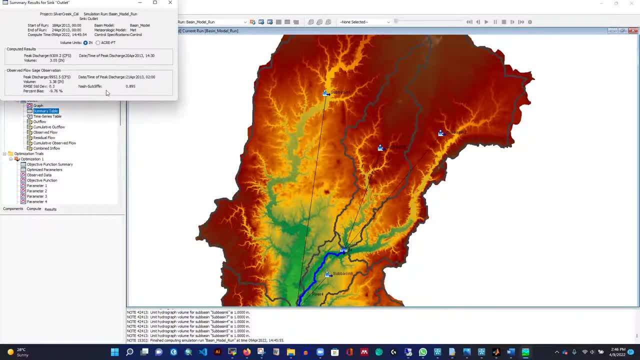 or what will happen if we, if we, if we individually reduce, individually reduce, individually reduce? yeah, yeah, individually reduce. yeah, yeah, individually reduce. yeah, is there any increment a little bit? is there any increment a little bit? is there any increment a little bit? but? but, but okay, see, let's see your scrub number. 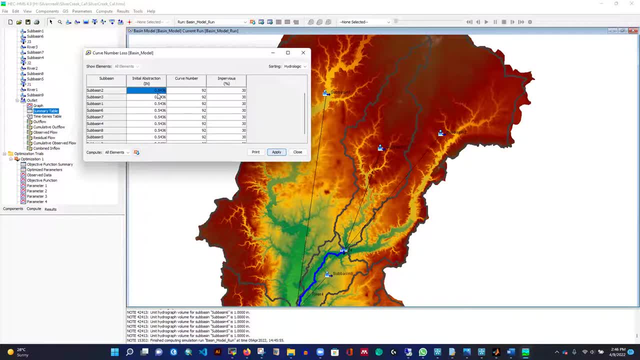 okay, see, let's see your scrub number. okay, see, let's see your scrub number. and here and here and here, i can even reduce this value. i can even reduce this value. i can even reduce this value drastically to 0.3, drastically to 0.3. 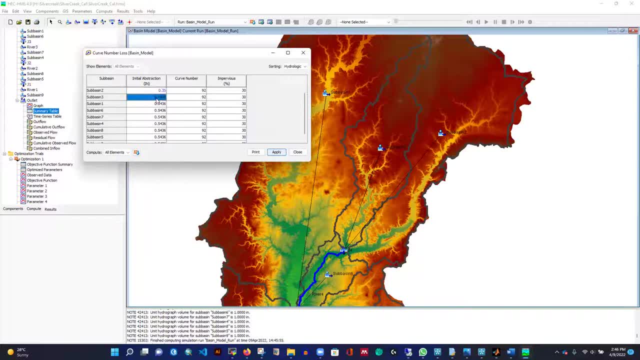 drastically to 0.3. or okay, not three, four, oh, three five is. or okay, not three, four, oh, three five is. or okay, not three, four, oh, three five is. okay, okay, okay and for. because i'm doing this for and for. because i'm doing this for. 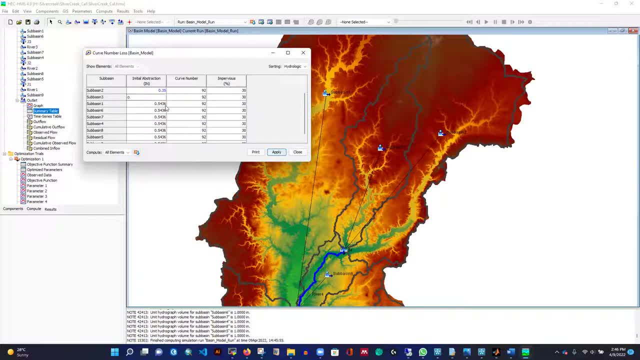 and for, because i'm doing this for upstream, upstream, upstream. and this value, i can even do it as, and this value, i can even do it as, and this value, i can even do it as- 0.35 as well, 0.35 as well, 0.35 as well, and sub base in one, i can do the same. 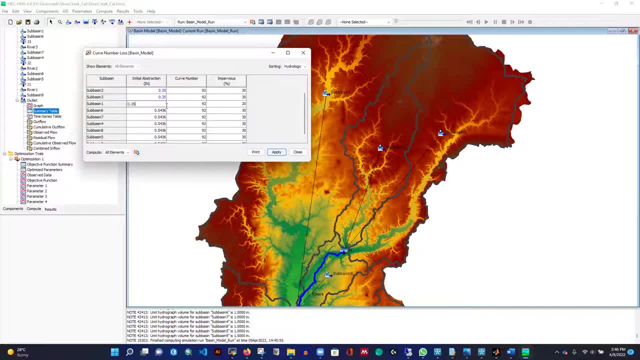 and sub base in one, i can do the same and sub base in one, i can do the same thing for all these three thing for all these three thing for all these three: the upstream 0.35 and i'm keeping this, the upstream 0.35 and i'm keeping this. 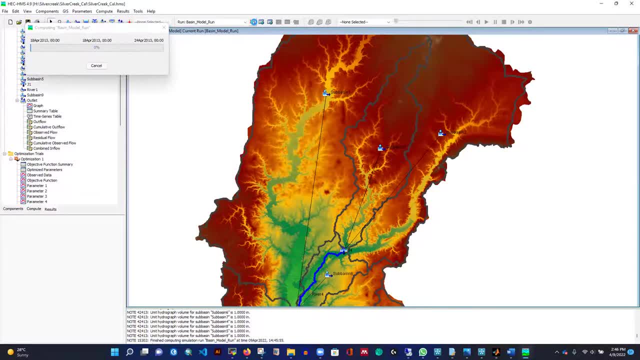 the upstream 0.35 and i'm keeping this as it is and let's run it as it is. and let's run it as it is and let's run it if we can get any improved value, because if we can get any improved value, because 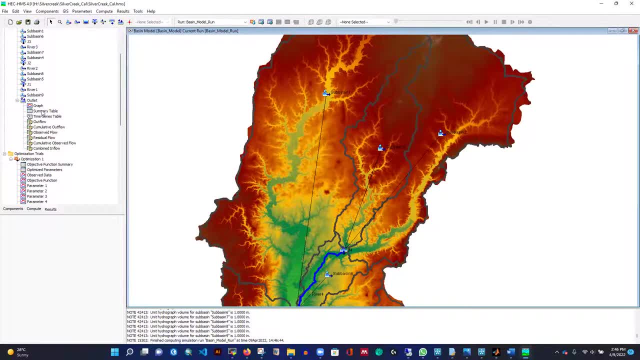 if we can get any improved value, because the initial abstraction won't be the same. the initial abstraction won't be the same. the initial abstraction won't be the same for all of this right. that is even for all of this right. that is even for all of this right that is even realistic and expected and see we can. 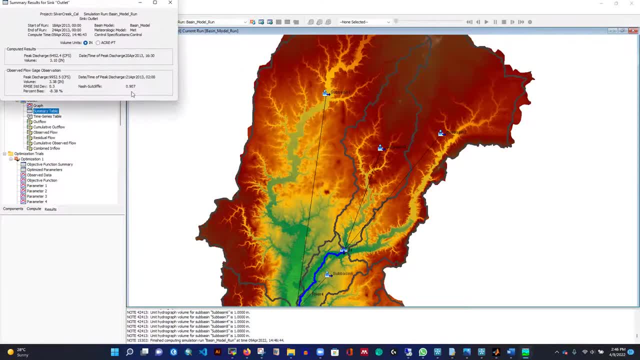 realistic and expected and see we can. realistic and expected and see we can get the closure carb and check that. yeah, get the closure carb and check that. yeah, get the closure carb. and check that. yeah, it's 90: 0.90, it's pretty good. it's 90: 0.90, it's pretty good. 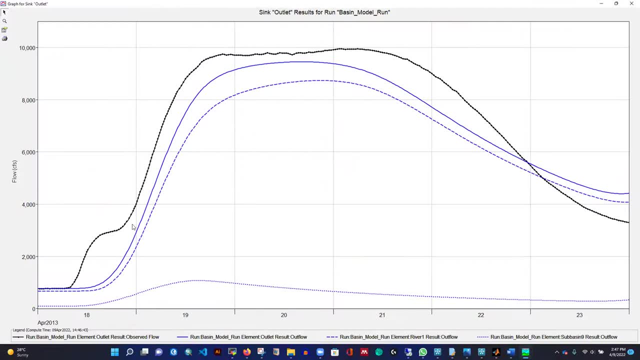 it's 90- 0.90. it's pretty good because i want more. so what do you have because i want more? so what do you have because i want more? so what do you have to do? you have to keep in mind that okay to do. you have to keep in mind that, okay. 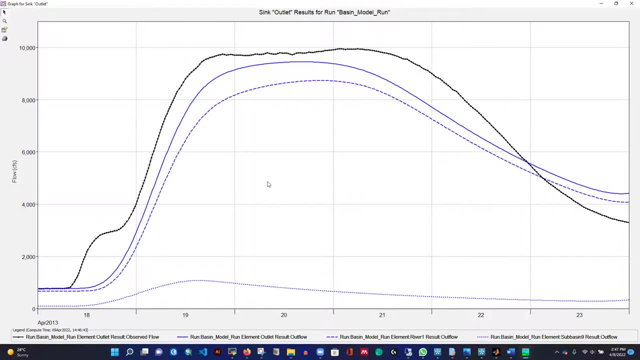 to do. you have to keep in mind that, okay, at the same time, you have to capture, at the same time you have to capture. at the same time, you have to capture the peak, the peak, the peak, and you have to capture the volume as, and you have to capture the volume as. 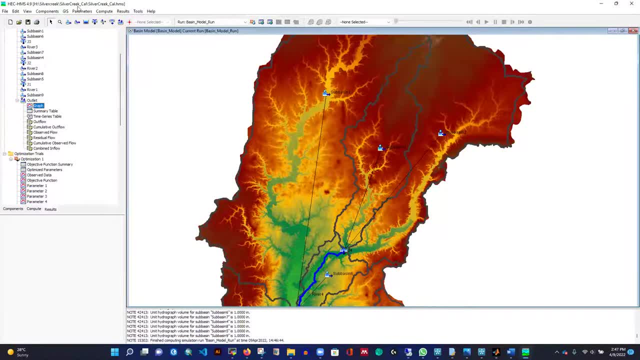 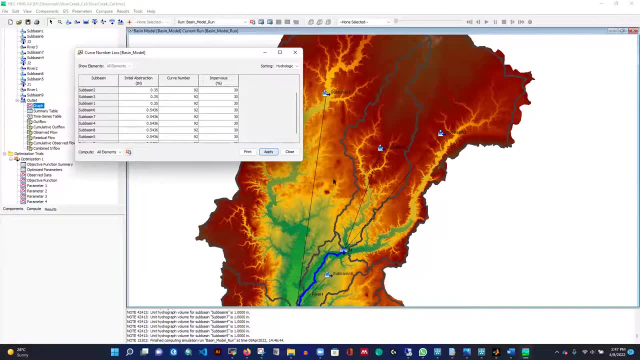 and you have to capture the volume as well. well, well, okay, so we can even reduce that a little. okay, so we can even reduce that a little. okay, so we can even reduce that a little bit bit bit and go to parameter and go to parameter and go to parameter loss and, instead of reducing the six, 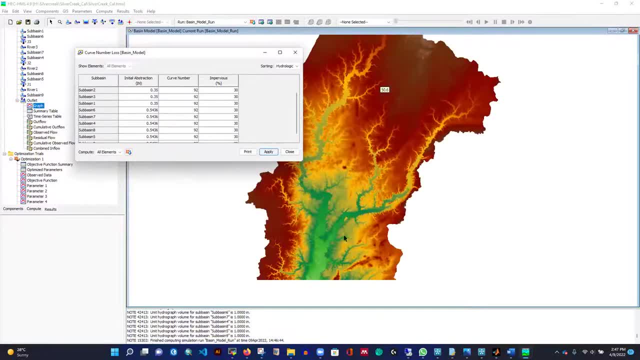 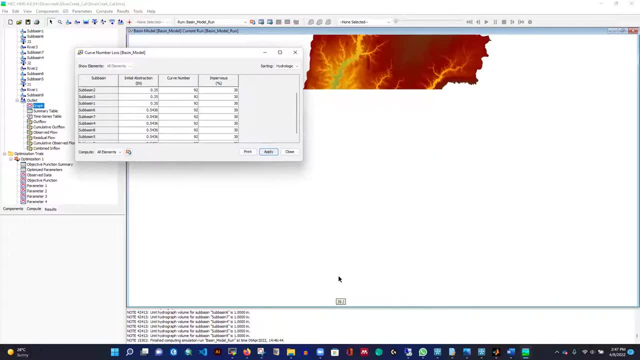 loss and instead of reducing the six loss and instead of reducing the six, these are the middle one. these are the middle one. these are the middle one. even i can reduce, even i can reduce, even i can reduce. okay, i can even reduce for i can even reduce, for. 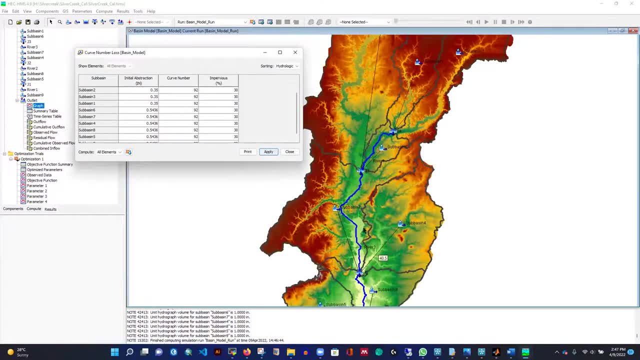 i can even reduce for uh, this one, that are even close to my, uh, this one, that are even close to my, uh, this one, that are even close to my outlet, okay, outlet, okay, outlet, okay. like this one for for the first time, i like this one for for the first time i 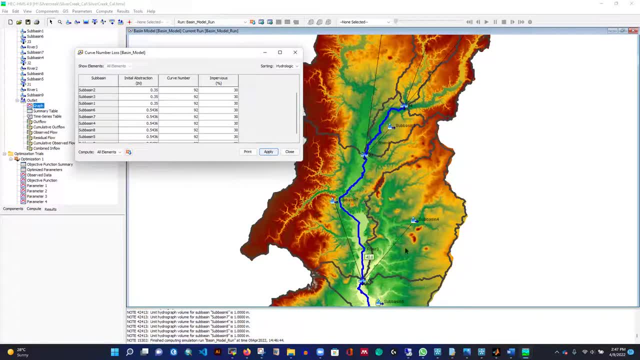 like this one, for for the first time, i did it, did it, did it, and then for seven, and then for seven, and then for seven, and we have four, so we can change this, and we have four, so we can change this, and we have four, so we can change this parameter. like: 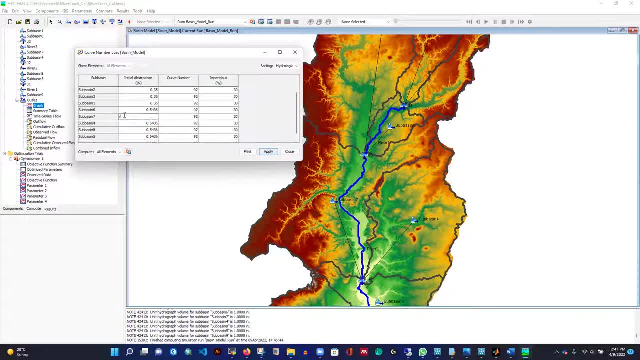 parameter like parameter like seven and four, seven and four, seven and four. okay, we can change the same like three. okay, we can change the same like three. okay, we can change the same like three, five, five, five and four do the same thing as and four do the same thing as. 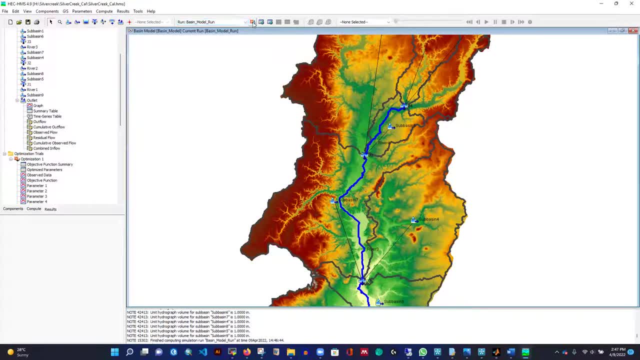 and four do the same thing as three five, three, five, three, five. yeah, this is the. yeah, this is the yeah. this is the boring job you have to do. boring job you have to do. boring job you have to do, and let's run it okay, and then it's done. 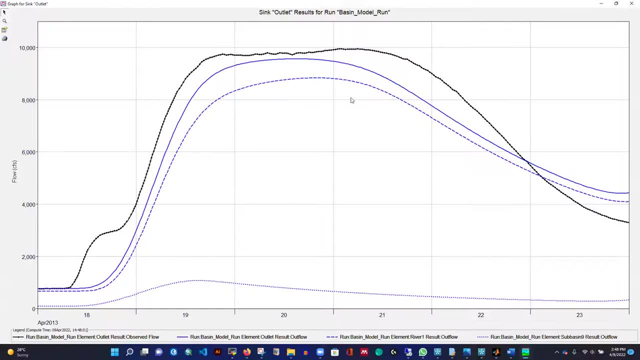 and let's run it okay, and then it's done. and let's run it okay, and then it's done. check, maybe it's even closer right. check, maybe it's even closer right. check, maybe it's even closer right, closer than before. okay, that's pretty. closer than before. okay, that's pretty. 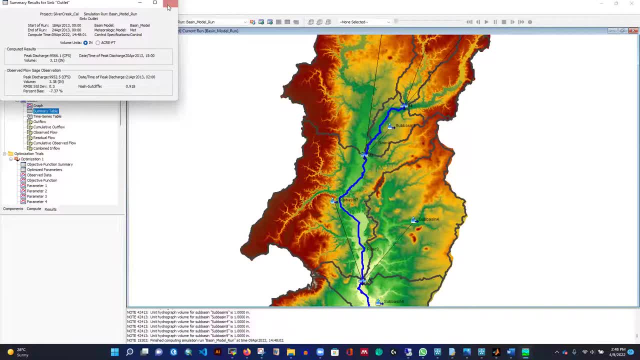 closer than before. okay, that's pretty good, and let's see good and let's see good and let's see, yeah, we have nine one eight when it's: yeah, we have nine one eight when it's: yeah, we have nine one eight when it's increasing. it's really good. 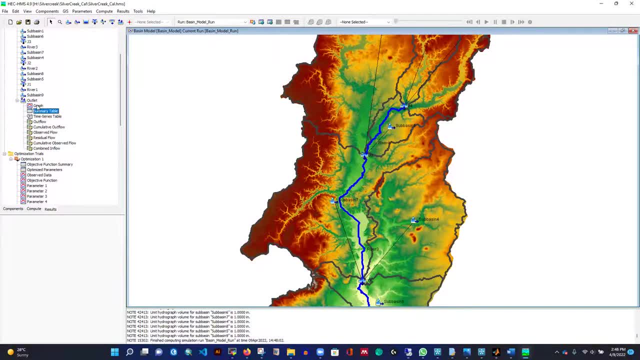 increasing it's really good. increasing it's really good. so one thing we can do is still our. so one thing we can do is still our. so one thing we can do is still our. model is under model, is under model, is under estimating. so we have to even reduce. 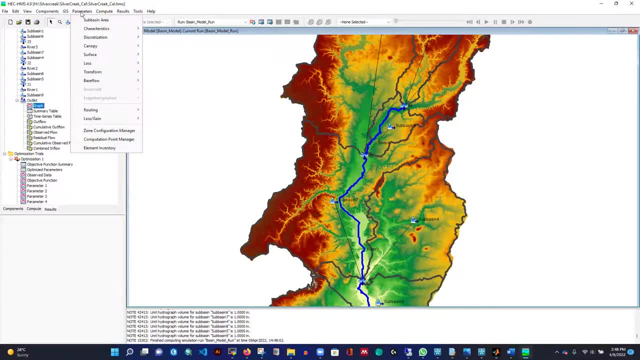 estimating. so we have to even reduce estimating. so we have to even reduce the loss, the loss, the loss. then we'll fix the transform. so from then we'll fix the transform. so from then we'll fix the transform. so, from parameter loss, and we are just doing the 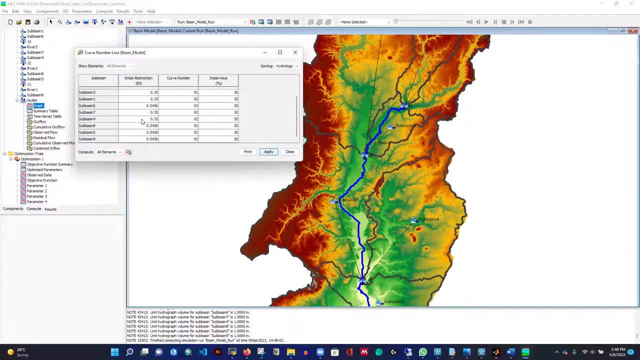 parameter loss, and we are just doing the parameter loss and we are just doing the same thing there. so, instead of doing that, even we can. so, instead of doing that, even we can. so, instead of doing that, even we can use uh 0.30. use uh 0.30. 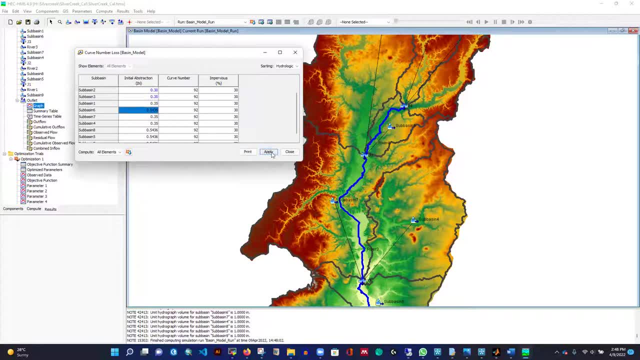 use: uh, 0.30. okay, there, 0.30. okay there, 0.30. okay, there, 0.30. and let's see if we can get any. and let's see if we can get any and let's see if we can get any improvement. 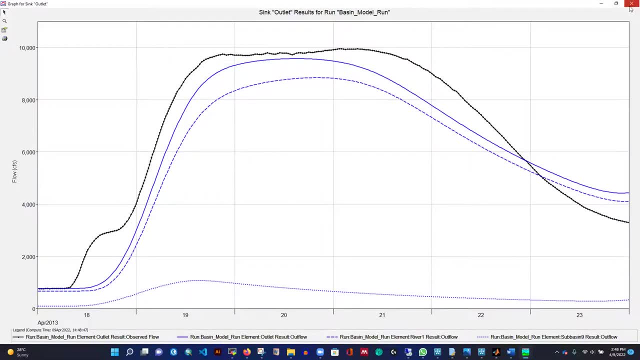 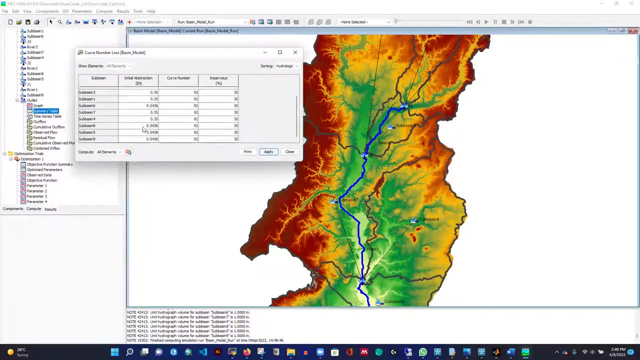 that's okay, but i need to toss that line. that's okay, but i need to toss that line. that is my objective loss. that is my objective loss. that is my objective loss. scs curve number: this time i'll reduce. scs curve number: this time i'll reduce. 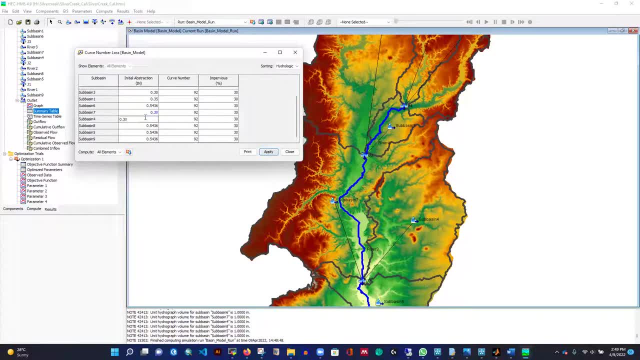 scs curve number. this time i'll reduce this one, this one, this one, to 30 to 30, to 30 to 0.30, and then i'll do the rest of the to 0.30, and then i'll do the rest of the. 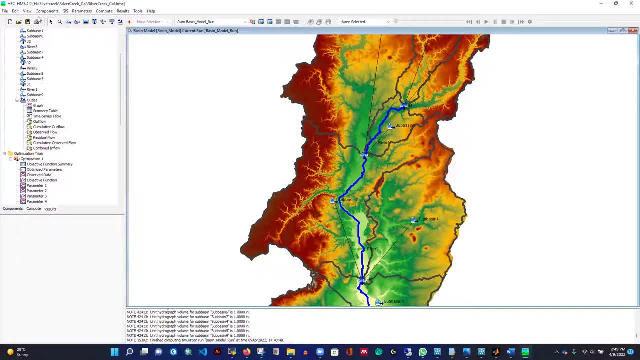 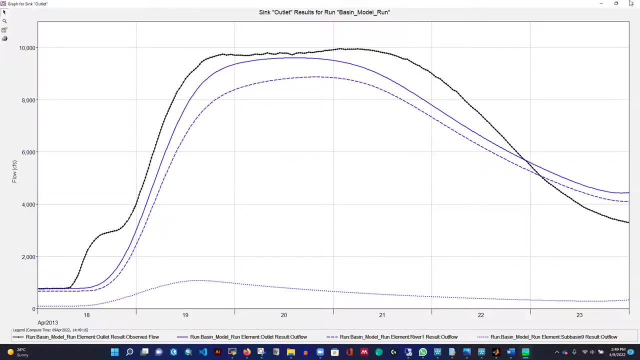 to 0.30, and then i'll do the rest of the thing for other subbasins as well, that thing for other subbasins as well, that thing for other subbasins as well. that doesn't matter, doesn't matter, doesn't matter. two, it's already nine. two, that means it. 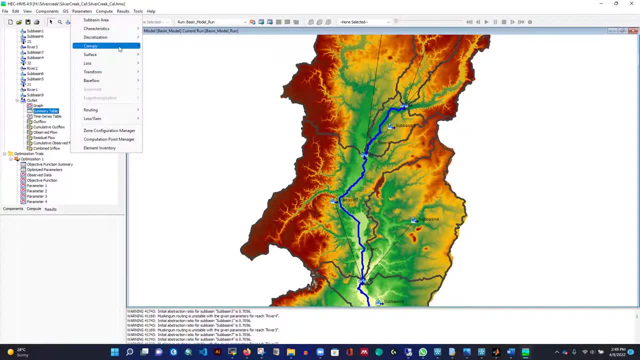 two, it's already nine. two that means it. two, it's already nine. two that means it is, is is improving right. so another thing we can improving right. so another thing we can improving right. so another thing we can do, do, do, uh, loss method, scs, curve number. 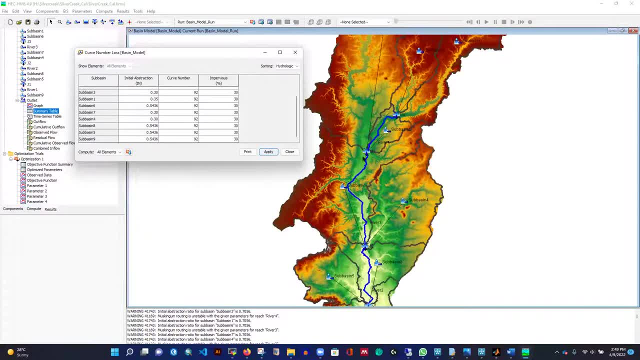 uh loss method- scs curve number. uh loss method- scs curve number. and then we can even reduce the values, and then we can even reduce the values, and then we can even reduce the values for for for: uh three, this one, six right. what is the? uh three, this one, six right. what is the? 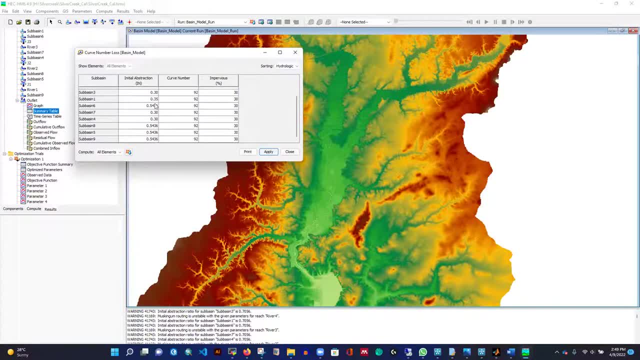 uh, three, this one six, right, what is the value? value? value of subbasin or subbasin number six. so we of subbasin or subbasin number six. so we of subbasin or subbasin number six. so we can do this to subbasin number. 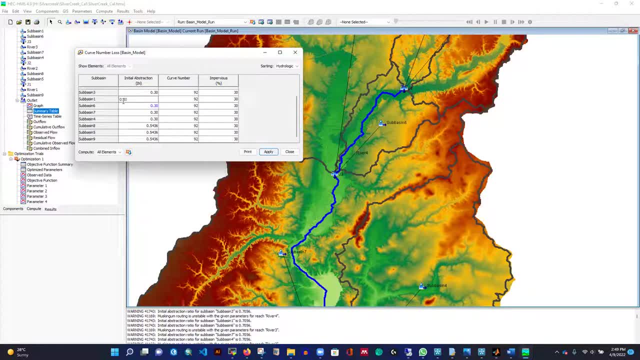 can do this to subbasin number, can do this to subbasin number: this one, three. oh, you have to even reduce this one, three. oh, you have to even reduce this one, three. oh, you have to even reduce this one zero point three, zero, so that we 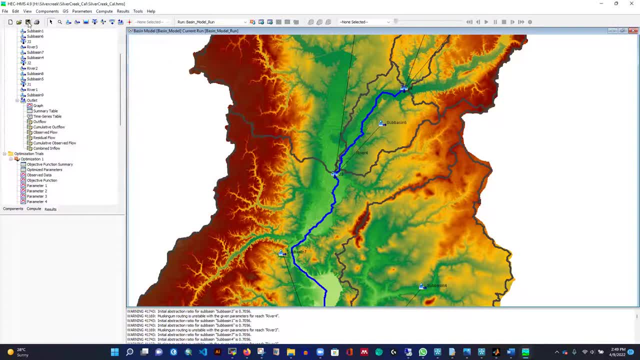 this one zero point three, zero, so that we this one zero point three, zero, so that we can get any improvement there can get any improvement there, can get any improvement there. okay, so save the model. definitely it. okay, so save the model. definitely it okay. so save the model. definitely it will improve this time. 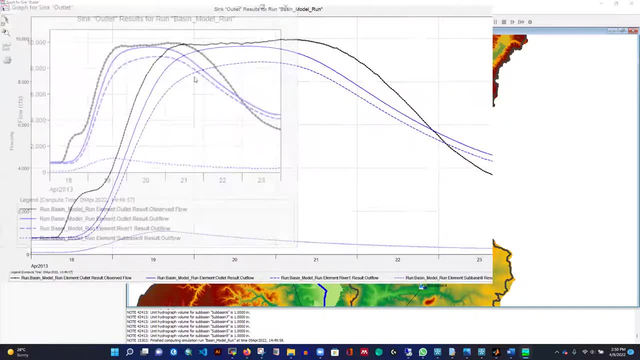 will improve this time, will improve this time a little bit. i guess, yeah, touching i a little bit. i guess, yeah, touching i a little bit. i guess, yeah, touching i guess. right, it's close enough to toss? guess, right, it's close enough to toss? guess, right, it's close enough to toss that. 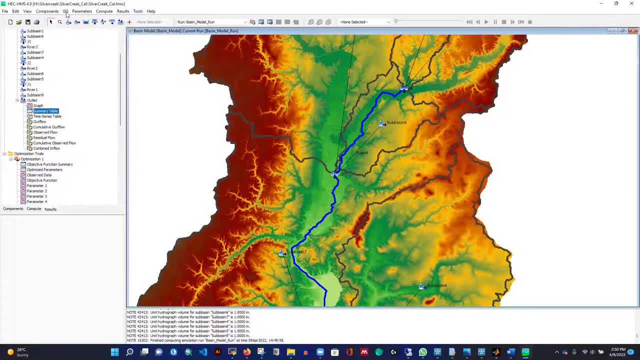 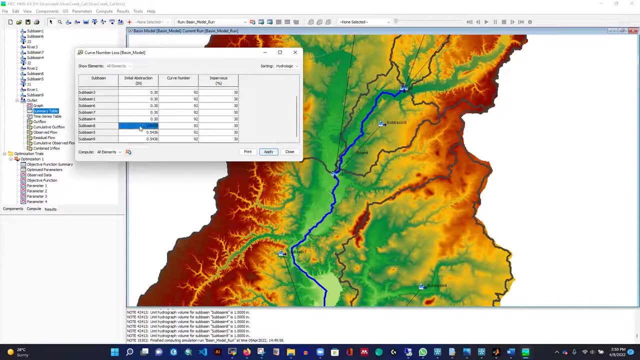 that, and then we have even nine to three, and then we have even nine to three, and then we have even nine to three. that means, if we even reduce, that means if we even reduce, that means if we even reduce the value for the value, for the value for other as well, everything. 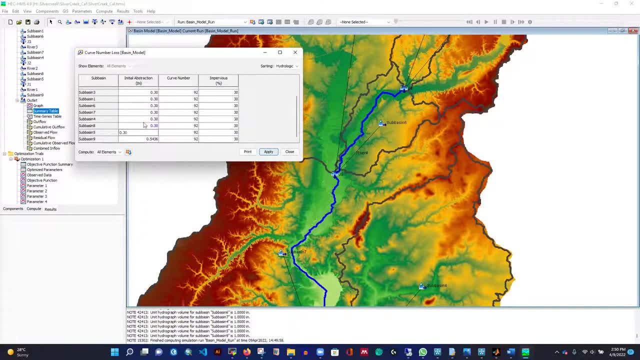 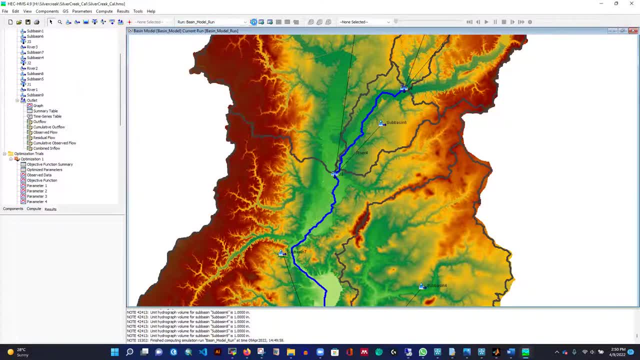 nine is basically 0.30 as well. the nine nine is basically 0.30 as well. the nine is the outlet that is draining directly. is the outlet that is draining directly? is the outlet that is draining directly? okay, so let's see if we can definitely. 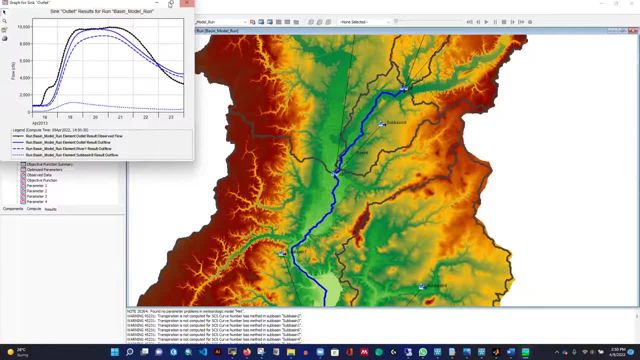 okay, so let's see if we can definitely. okay, so let's see if we can. definitely we'll get some visible improvement there. we'll get some visible improvement there. we'll get some visible improvement there in the graph. yeah, it touching that see in the graph. yeah, it touching that see. 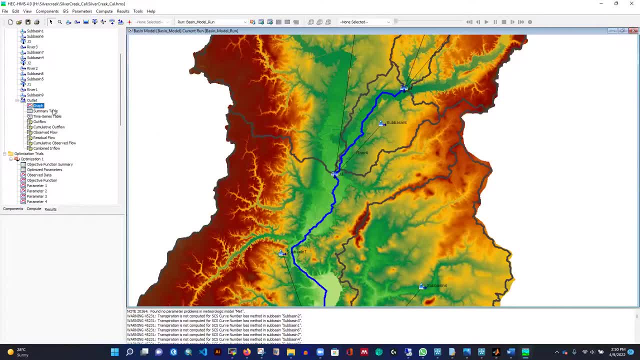 in the graph. yeah, it touching that see, it's touching now, it's touching now, it's touching now. so, so, so, and you can see it's nine to eight, and you can see it's nine to eight, and you can see it's nine to eight, and we can even- okay, let's investigate. 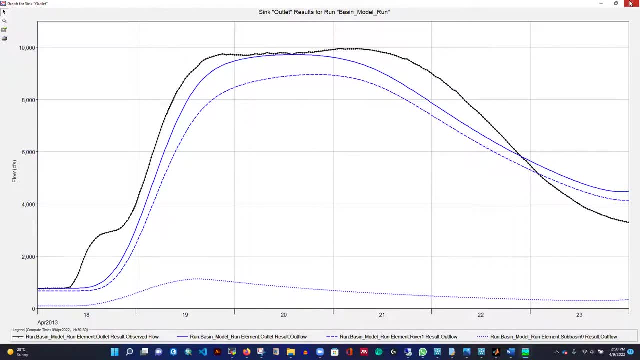 and we can even, okay, let's investigate. and we can even, okay, let's investigate the, the, the graph. we can even increase it a little graph. we can even increase it a little graph. we can even increase it a little bit bit bit. right so i can, right so i can. 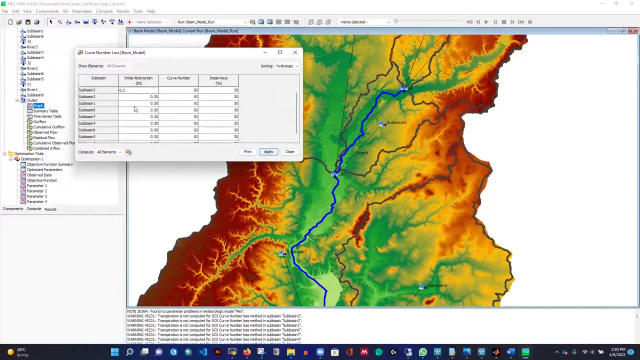 right, so i can even reduce the loss for this two, even reduce the loss for this two, even reduce the loss for this two to 0.25 and this 0.25, and for this to 0.25 and this 0.25 and for this. 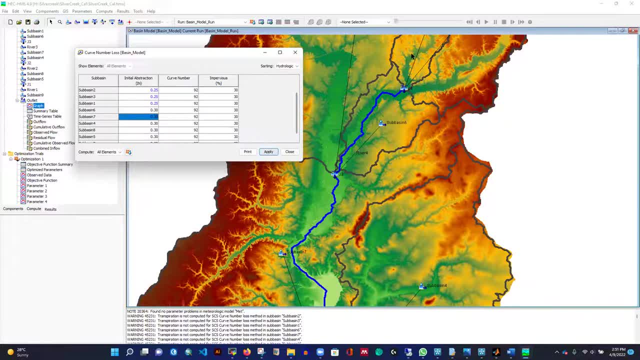 to 0.25 and this 0.25 and for this upstream: okay, i'm doing this for upstream. okay, i'm doing this for upstream. okay, i'm doing this for this three upstream sub basins, this three upstream sub basins, this three upstream sub basins. and now, if i can, 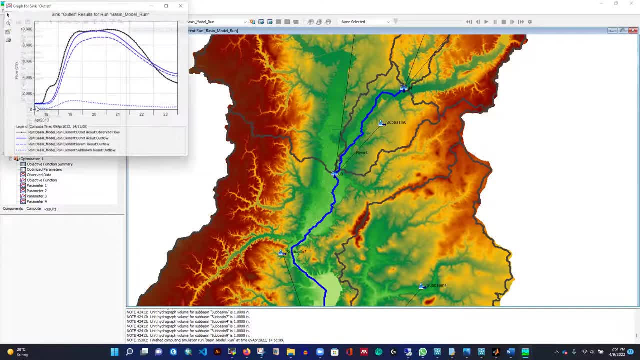 and now, if i can, and now if i can do that, do that, do that, you close it and then see the graph, it's. you close it and then see the graph, it's. you close it and then see the graph: it's touching, pretty touching, pretty touching, pretty accurately touching okay. 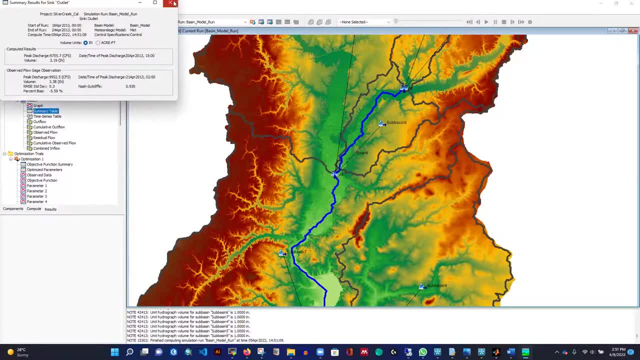 accurately touching okay, accurately touching, okay. so that's good, so that's good, so that's good. and let's check that is nine three and let's check that is nine three and let's check that is nine three, even. okay, i want more. okay, because it is. 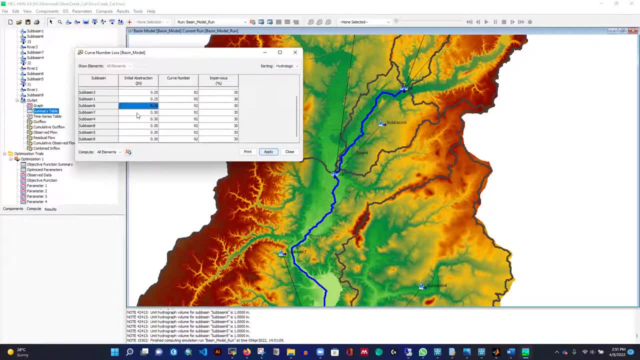 even okay. i want more okay because it is even okay. i want more okay because it is responding the way i'm responding, the way i'm responding the way i'm expecting. so reduce that to 0.25. expecting. so reduce that to 0.25. 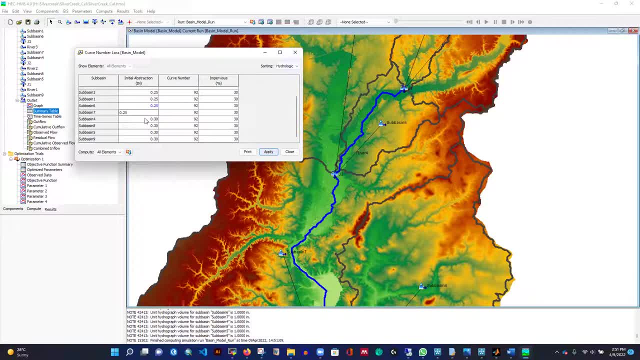 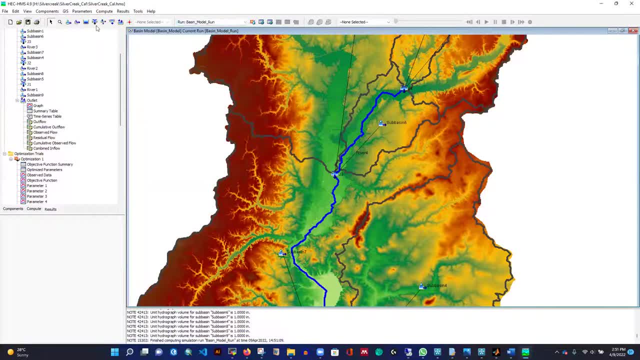 and for four and seven as well: 0.25. okay, okay, okay. so let's see, save the model, so let's see save the model, so let's see save the model and run it, and run it, and run it. hopefully it is gonna work this time. 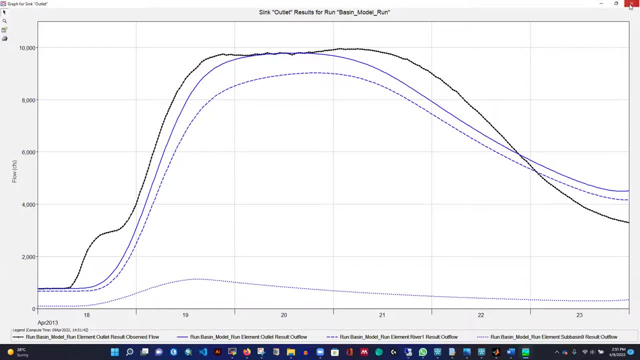 hopefully it is gonna work this time. hopefully it is gonna work this time. okay so reduce the gap. it pretty okay, so reduce the gap. it pretty okay, so reduce the gap. it pretty equally toss the, equally toss the, equally toss the peak, peak, peak. and we can see any improvement there. so 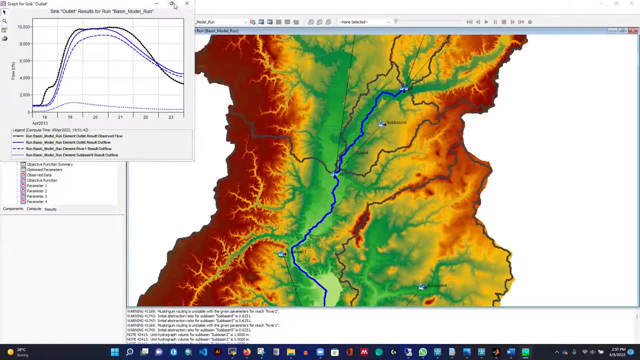 and we can see any improvement there. so, and we can see any improvement there. so, nine three, two. nine three, two, nine three, two, and let's investigate further what we have and let's investigate further what we have and let's investigate further what we have to do. i think we are done with this one. 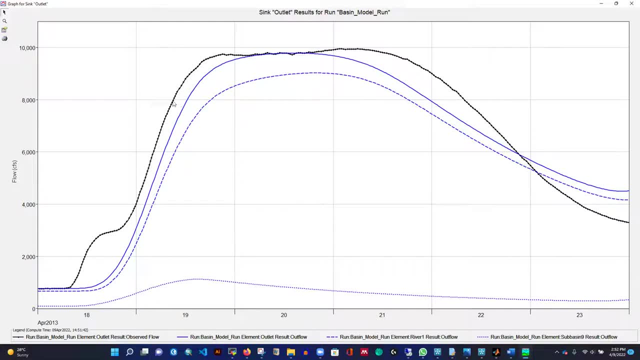 to do. i think we are done with this one to do. i think we are done with this one: uh, other than capturing this peak, uh, other than capturing this peak, uh, other than capturing this peak, we can even match these two, right, we can. we can even match these two, right, we can. 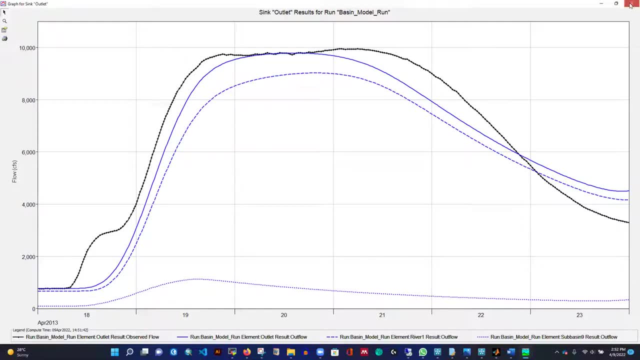 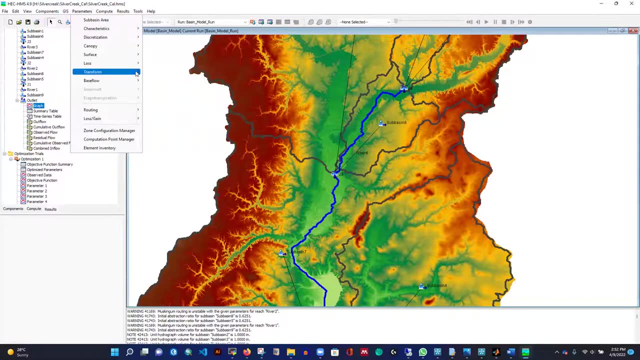 we can even match these two right. we can reduce this gap, reduce this gap, reduce this gap. so we can use our, so we can use our, so we can use our net time of concentration to do that net time of concentration, to do that net time of concentration to do that. so go to transform. 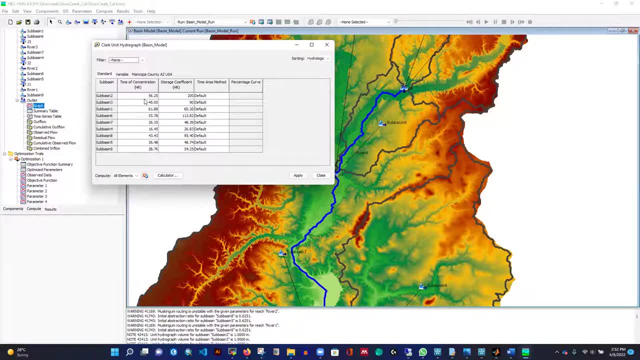 so go to transform. so go to transform: clark unit hydrograph, clark unit hydrograph, clark unit hydrograph and reduce this time of concentration. we can play with time of concentration. we can play with time of concentration. we can play with that one as well. 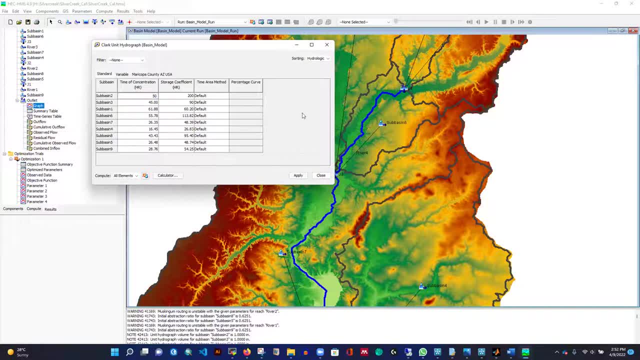 that one as well, that one as well. right, you can use 50 and right, you can use 50 and right, you can use 50, and we can check that. okay, if it works, we can check that. okay, if it works, we can check that. okay, if it works, and run it- see how many times i'm running. 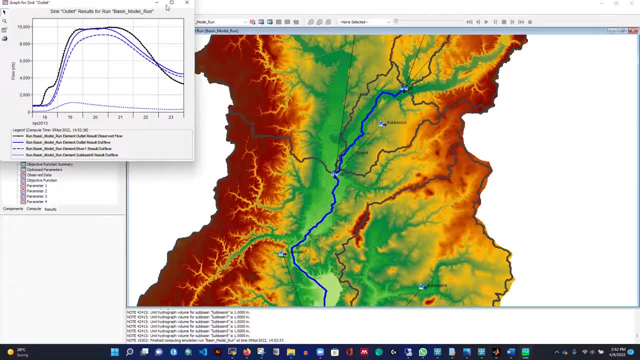 and run it. see how many times i'm running and run it. see how many times i'm running the model, the model, the model. so it's really so, it's really so. it's really hectic job, hectic job, hectic job. maybe it shifted a little bit. that's why. 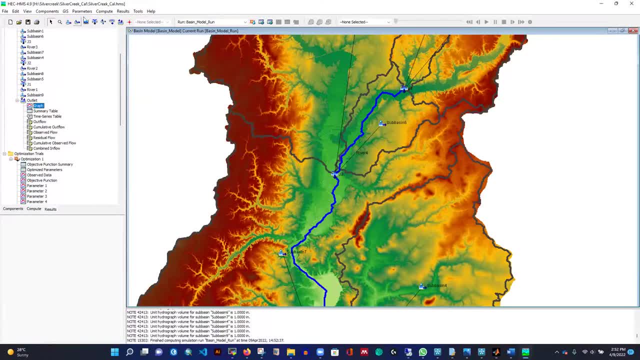 maybe it shifted a little bit. that's why maybe it shifted a little bit, that's why it is crossing that line. it is crossing that line, it is crossing that line. and if i even reduce, and if i even reduce, and if i even reduce the, the, the time of concentration for 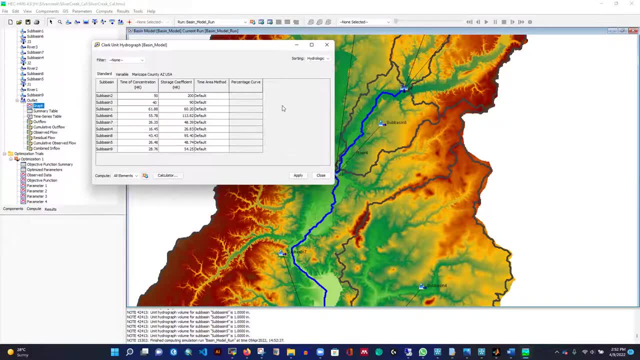 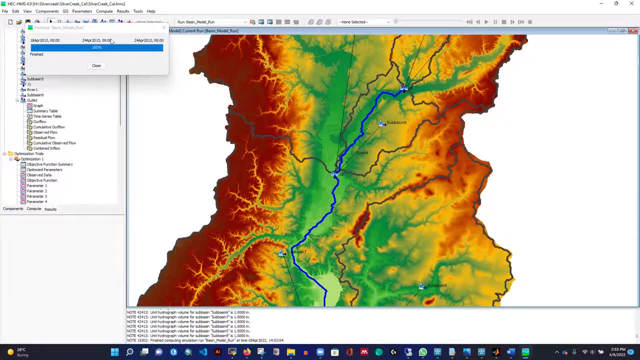 time of concentration for time of concentration for this one. okay, this one, okay, this one. okay, use 40, use 40, use 40, 40, 40, 40 and saving it, and saving it, and saving it, running it again, running it again, running it again. let's see. 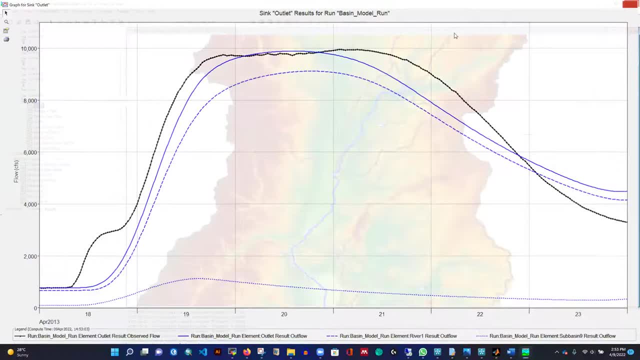 let's see. let's see, okay, yeah, it shifted a little bit. i okay, yeah, it shifted a little bit. i okay, yeah, it shifted a little bit. i guess, guess, guess, that's what i can see, and if it. that's what i can see and if it. 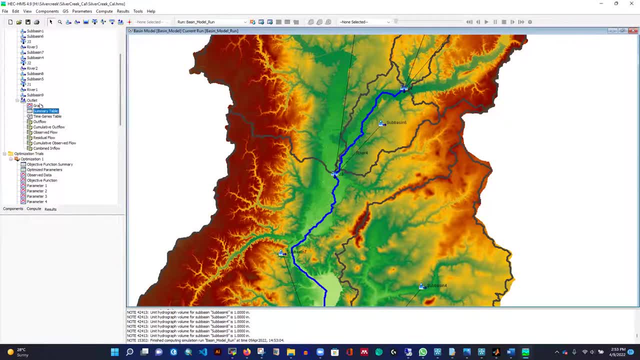 that's what i can see. and if it improved nine three i, i don't know if it improved nine three i i don't know if it improved nine three i i don't know if it is going to improve but is going to improve, but is going to improve. but we have to capture the shape. now we are. 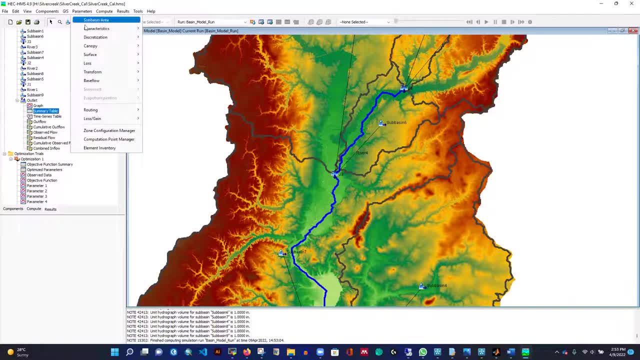 we have to capture the shape. now we are. we have to capture the shape now we are working on the shape, working on the shape, working on the shape and let's check if we can improve it and let's check if we can improve it and let's check if we can improve it more. 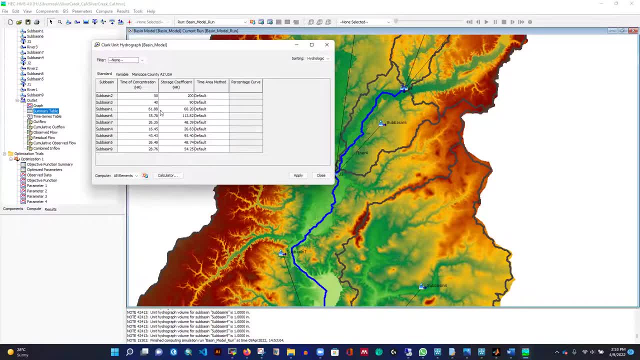 more, more or not. this one because we are working or not this one. because we are working or not this one, because we are working on the transform method, on the transform method, on the transform method. okay, so we can even use this one. okay, so we can even use this one. 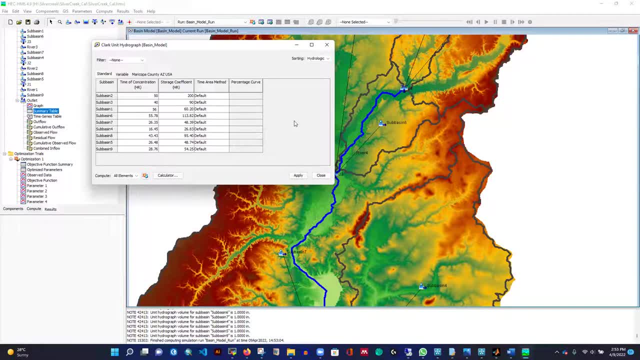 okay, so we can even use this one instead of 61. okay, 55 oh 56 instead of 61. okay, 55 oh 56 instead of 61. okay, 55 oh 56, okay, and then okay, and then okay, and then run the model. run the model. 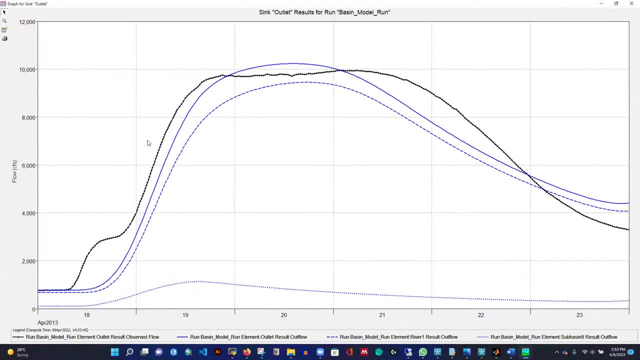 run the model and check it. yeah, maybe it is just and check it. yeah, maybe it is just and check it. yeah, maybe it is just getting closer and closer, getting closer and closer, getting closer and closer. right, okay, but at the same time see it. right, okay, but at the same time see it. 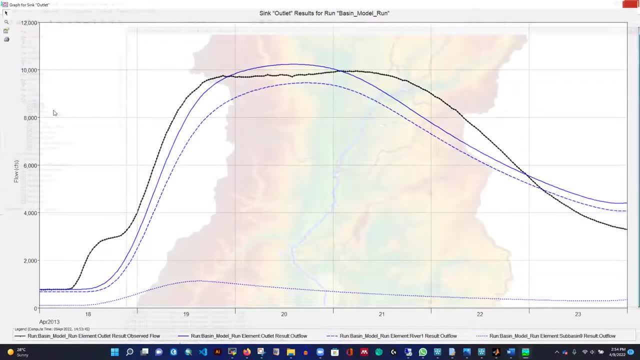 right, okay, but at the same time, see, it is even, is even, is even increasing the peak, and let's check increasing the peak. and let's check increasing the peak. and let's check this one as well, it is nine three. this one as well, it is nine three. 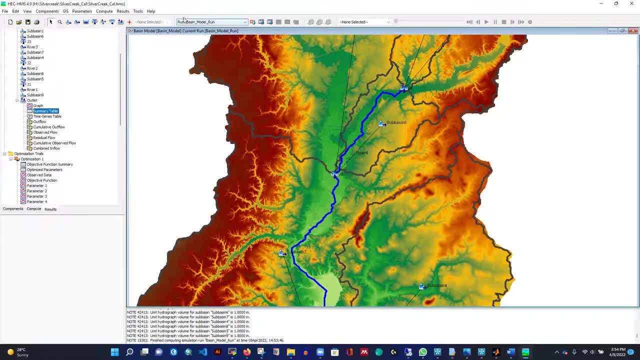 this one as well. it is nine three: reducing the performance: okay, that's reducing the performance. okay, that's reducing the performance. okay, that's okay. we can even reduce the loss. okay, we can even reduce the loss. okay, we can even reduce the loss. we can increase the loss, we can. 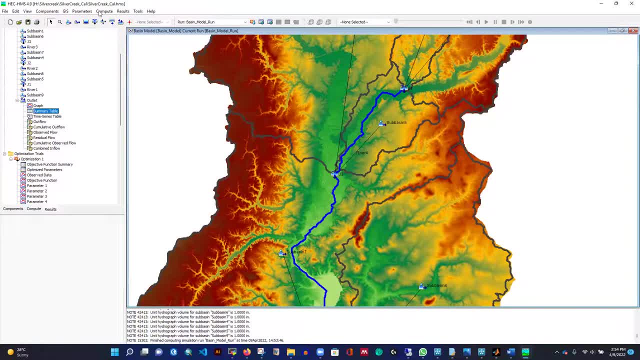 we can increase the loss we can. we can increase the loss. we can capture that, capture that. capture that pick, not a problem. so, instead of doing pick, not a problem. so, instead of doing pick, not a problem. so instead of doing that, that, that i can even change everything, okay. 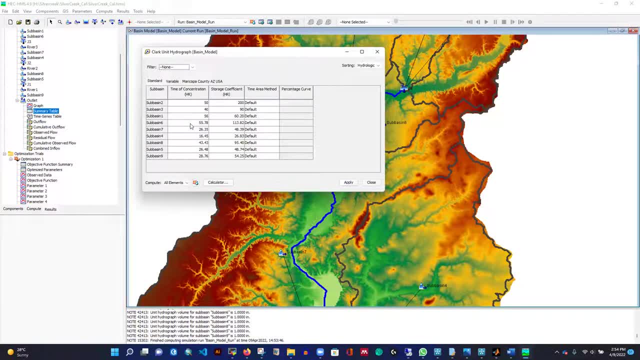 i can even change everything. okay, i can even change everything. okay at first. okay this time instead of at first. okay this time instead of at first. okay this time. instead of changing one by one, changing one by one, changing one by one, i can change all of this, okay. 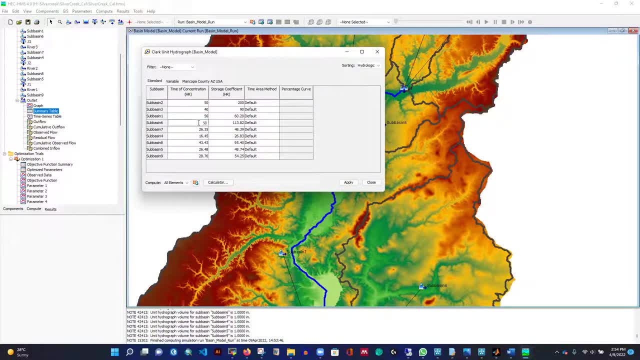 i can change all of this. okay, i can change all of this, okay. so, instead of this, i can even use as 50. so, instead of this, i can even use as 50. so, instead of this, i can even use as 50, and then i can even use that 26 to. 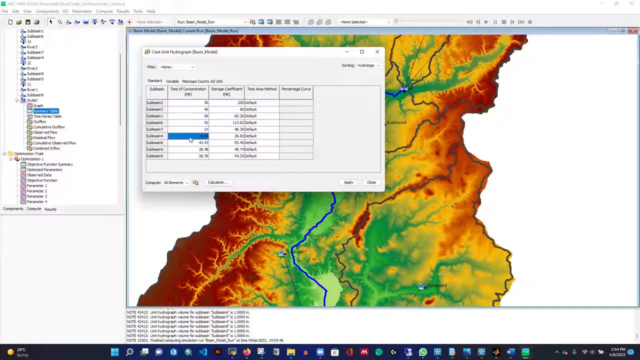 and then i can even use that 26 to, and then i can even use that 26 to 24, 24, 24, because these are smaller ones. so this is because these are smaller ones. so this is because these are smaller ones. so this is 16. 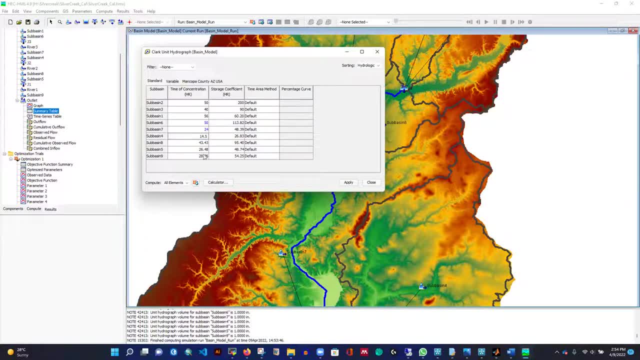 16, 16. then i can use okay 14.5, then i can use okay 14.5, then i can use okay 14.5. and for and for and for eight. i can use even 30. this is eight. i can use even 30, this is. 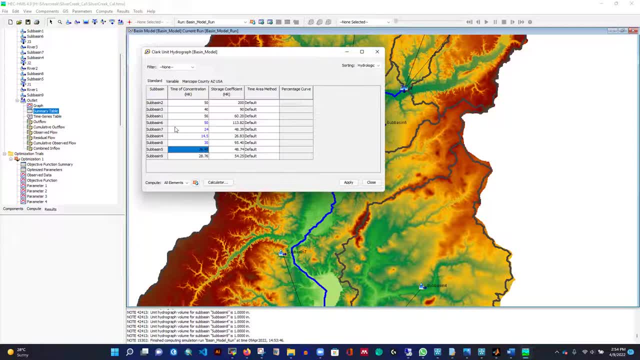 eight, i can use even 30. this is a little bit bigger, and instead of a little bit bigger and instead of a little bit bigger. and instead of 26, i can even use 26, i can even use 26. i can even use 20. that's okay. instead of 20, okay, this. 20: that's okay instead of 20. okay, this 20: that's okay instead of 20. okay, this is i can, is i can, is i can. nine: okay for nine. i can keep it as it. nine: okay for nine, i can keep it as it. 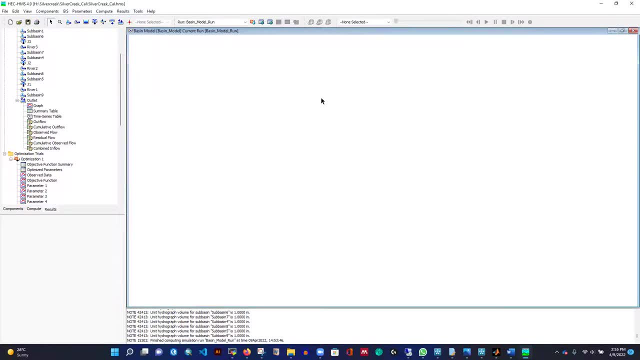 nine. okay for nine. i can keep it as it is. because i didn't change that much, is because i didn't change that much, is because i didn't change that much. nine is at the end, right at the end of. nine is at the end, right at the end of. 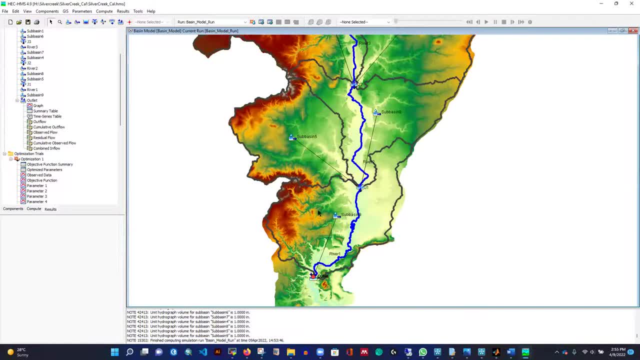 nine is at the end, right at the end of the watershed here. that is directly the watershed here. that is directly the watershed here that is directly draining into the draining, into the draining into the model. so let's run it if we can see any model. so let's run it if we can see any. 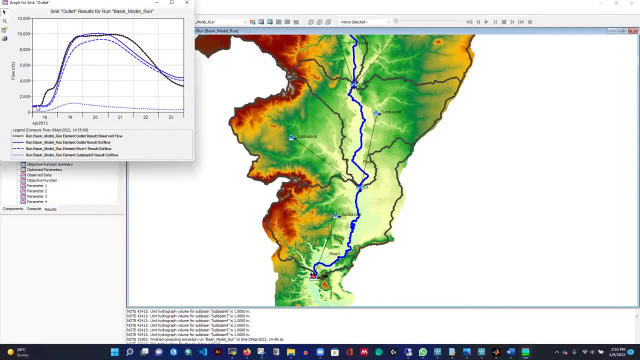 model, so let's run it. if we can see any changes, then we can change the value for changes. then we can change the value for changes. then we can change the value for nine as well, nine as well, nine as well. yeah, so see, it's getting closer. 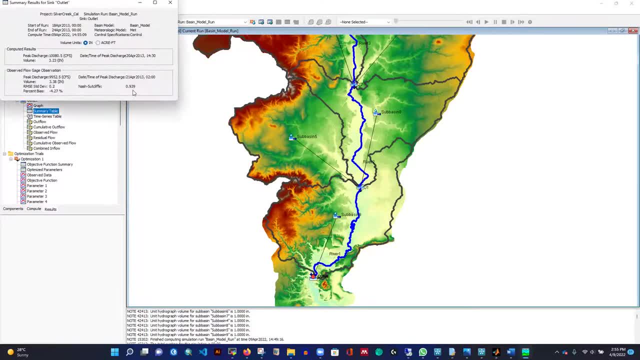 yeah, so see it's getting closer. yeah, so see it's getting closer, really closer and closer, really closer and closer, really closer and closer. so what is the value? see nine, three, nine. so what is the value? see nine, three, nine. so what is the value? see nine, three, nine. it's almost nine four. it's really good. 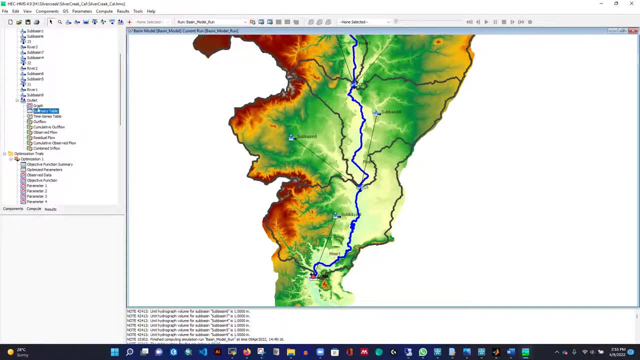 it's almost nine four, it's really good. it's almost nine four, it's really good. fantastic model. we can see the fantastic model. we can see the fantastic model. we can see the calibration is really good. even if you calibration is really good. even if you calibration is really good, even if you want to capture. 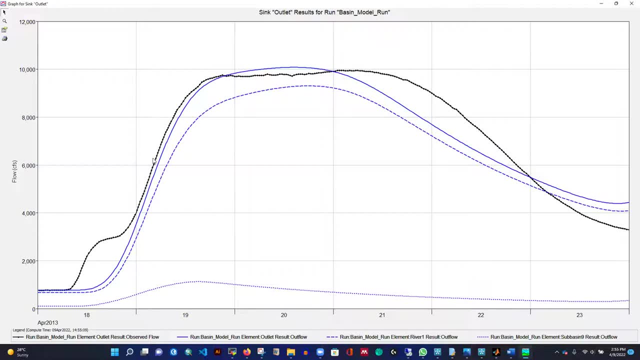 want to capture, want to capture this one pretty accurately. we can even do this one pretty accurately. we can even do this one pretty accurately. we can even do that, or we can even that. or we can even that, or we can even keep it as it is. see, i'm just cleaning it. 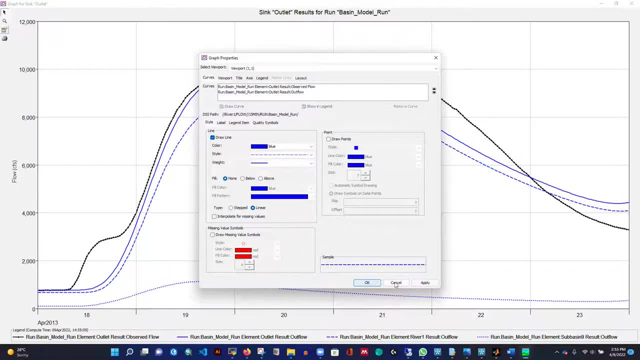 keep it as it is. see, i'm just cleaning it. keep it as it is, see, i'm just cleaning it. let's see if i remove this curve i can. let's see if i remove this curve i can. let's see if i remove this curve, i can remove this one as well. 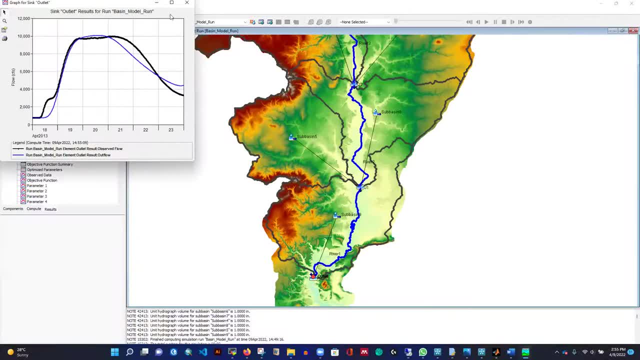 remove this one as well. remove this one as well, and i can see the changes here. see it's, and i can see the changes here. see it's, and i can see the changes here. see it's. looking really nice, right. looking really nice, right. looking really nice, right. yeah, it's really nice and it is possible. 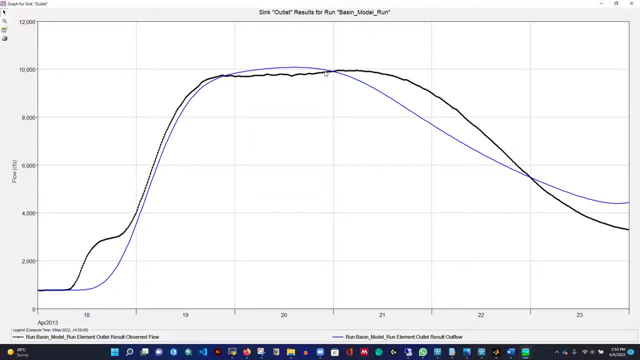 yeah, it's really nice and it is possible. yeah, it's really nice and it is possible to capture, to capture, to capture. but yeah, it is also possible to capture. but yeah, it is also possible to capture. but yeah, it is also possible to capture. then it will be. 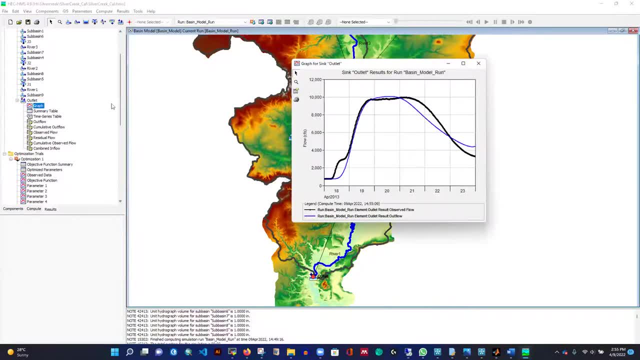 then it will be. then it will be uh improving but i think it's a really uh improving but i think it's a really uh improving, but i think it's a really good. calibration curve: the calibration good. calibration curve: the calibration good. calibration curve: the calibration curve is really good. 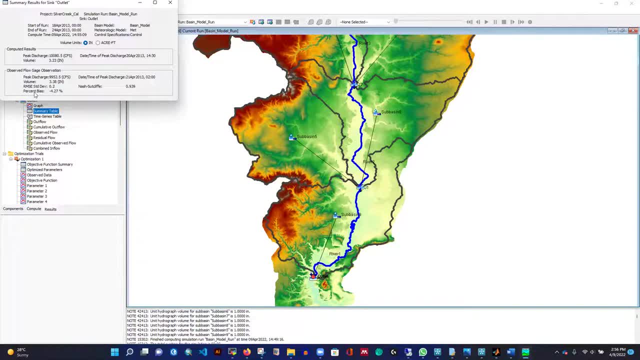 curve is really good. curve is really good. even it's really 939. and see the even: it's really 939. and see the even: it's really 939. and see the percentage bias is like less than five. percentage bias is like less than five. percentage bias is like less than five percent. 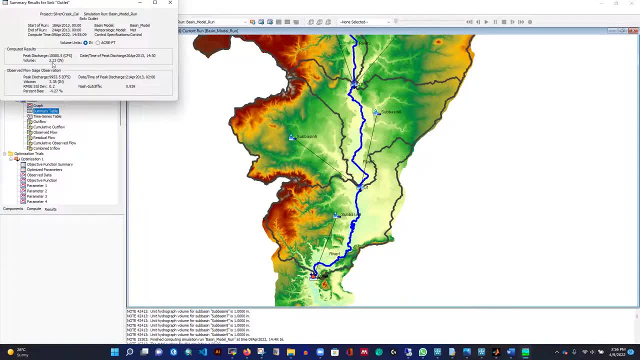 percent, percent right and the peak we capture like zero right and the peak we capture like zero right and the peak we capture like zero. three point two, three and the volume: three point two, three and the volume. three point two, three and the volume. this is, this is the volume. 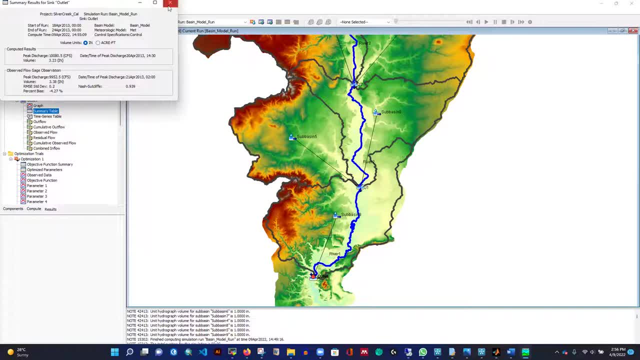 this is. this is the volume. this is: this is the volume, and the observation is like 3.38, so it's, and the observation is like 3.38, so it's, and the observation is like 3.38, so it's pretty close, pretty close. 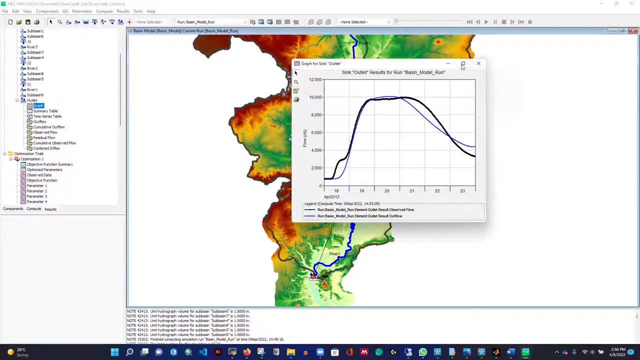 pretty close. so i think it's okay to, so, i think it's okay to, so, i think it's okay to validate the model. the calibration is. validate the model, the calibration is. validate the model, the calibration is okay. even we can okay, even, we can okay. even we can capture that one as well, if you try that. 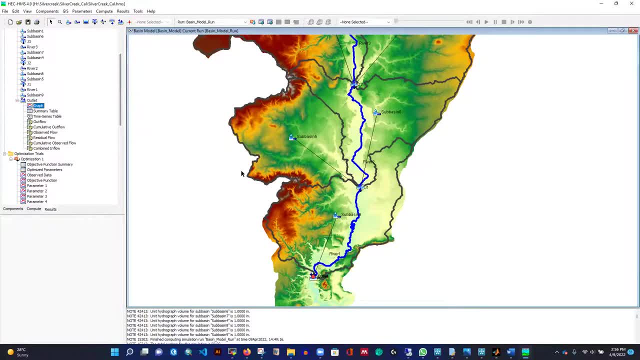 capture that one as well. if you try that, capture that one as well. if you try that, doesn't matter, doesn't matter, doesn't matter. so that's that. so that's that. so this is how we can even calibrate using. so this is how we can even calibrate using. 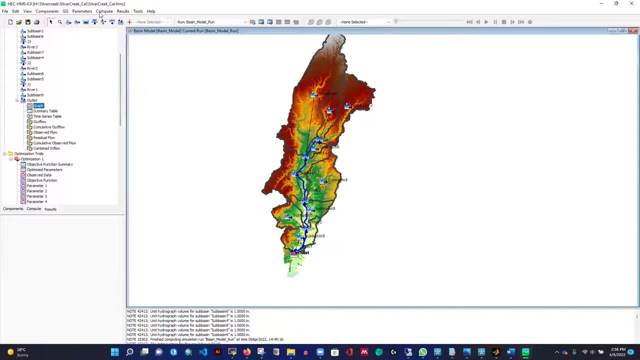 so this is how we can even calibrate, using automatic calibration: the optimization, automatic calibration, the optimization, automatic calibration, the optimization trial. you have trial, you have trial, you have, and if you already have the model, then, and if you already have the model, then and if you already have the model, then you can calibrate. but in this, 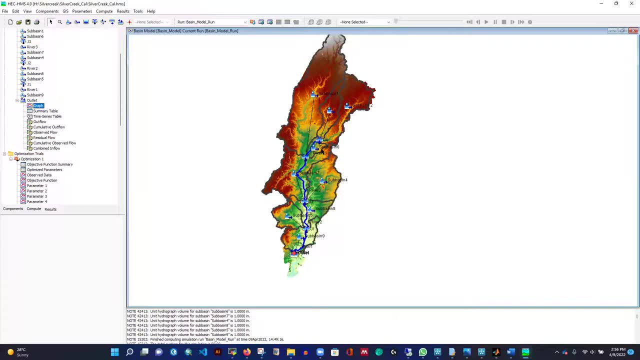 you can calibrate, but in this you can calibrate. but in this tutorial i didn't show how to set up tutorial. i didn't show how to set up tutorial. i didn't show how to set up the model, but i have different videos: the model, but i have different videos. 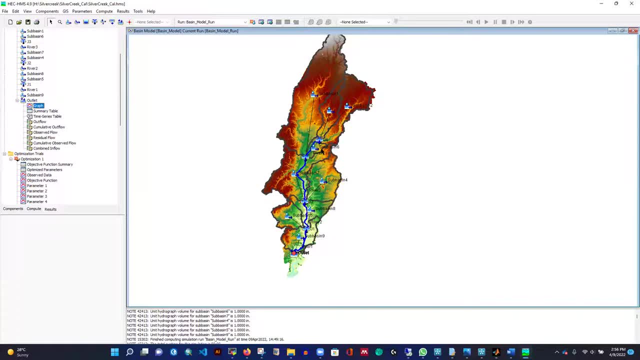 the model. but i have different videos. you can check that- how to set up the. you can check that how to set up the. you can check that how to set up the model from model from model, from dem data, so after that you can even calibrate the model. 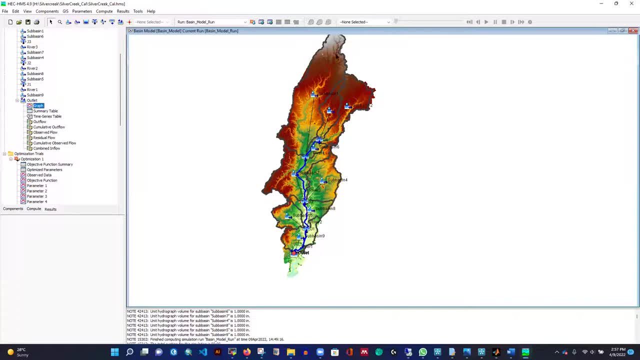 after that you can even calibrate the model. after that you can even calibrate the model, but it is even, but it is even, but it is even uh customary to calibrate the model, not uh customary to calibrate the model, not uh customary to calibrate the model, not for one single location, if you have like. 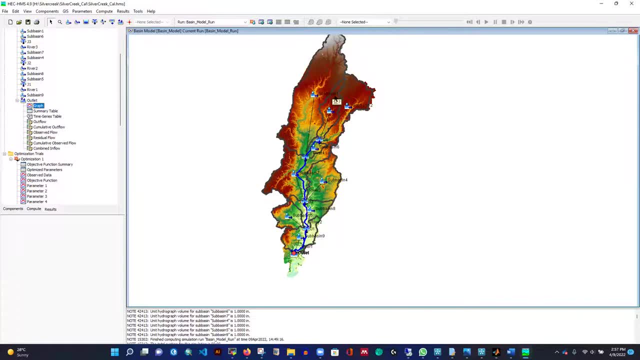 for one single location. if you have like for one single location, if you have like a larger, a larger, a larger watershed, then you can calibrate the watershed, then you can calibrate the watershed, then you can calibrate the model at multiple locations. model at multiple locations. 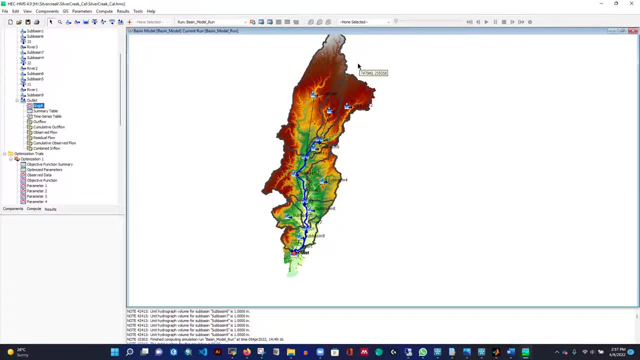 model at multiple locations. but for doing that, we have to have the but for doing that. we have to have the but for doing that, we have to have the observation data. but for this watershed observation data. but for this watershed observation data. but for this watershed, i don't have observation data here. or? 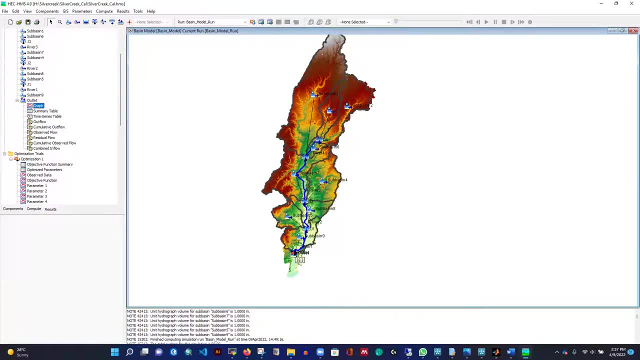 i don't have observation data here, or i don't have observation data here or here. i have only one outlet there. so here i have only one outlet there. so here i have only one outlet there. so that's why i'm just selecting this point. that's why i'm just selecting this point. 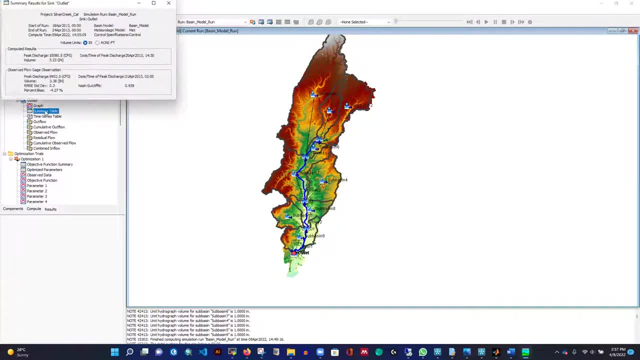 that's why i'm just selecting this point as my, as my, as my calibration point and i think the calibration point and i think the calibration point and i think the calibration looks pretty good. it is calibration, looks pretty good. it is calibration looks pretty good, it is almost uh. 0.93.